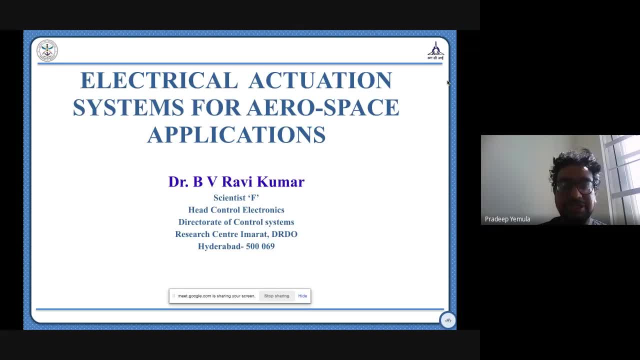 PDV for ballistic missile defence program, Design and development of electromagnetic propulsion technology for missile applications. So we have our future Abdul Kalam with us. So meanwhile, he has a lot of knowledge in the area of field development. What are his? he has a lot of awards, that is, agni award for excellence in self-reliance for development of. 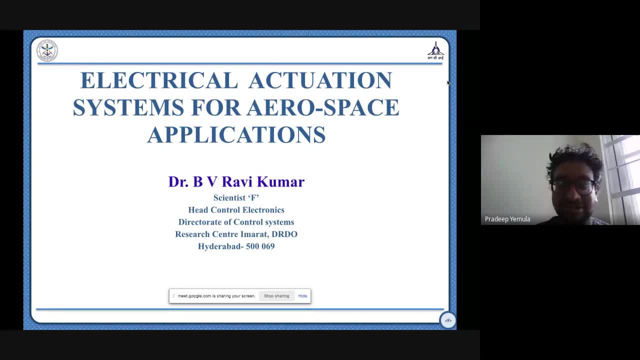 compact rotary activation system for pdv warhead gimbaling. and we have a dr devo award- uh, not we. he has the drd award for performance excellence for development of activation system for nearby cruise missile, and he also has an agni award for excellence in self-reliance for development of 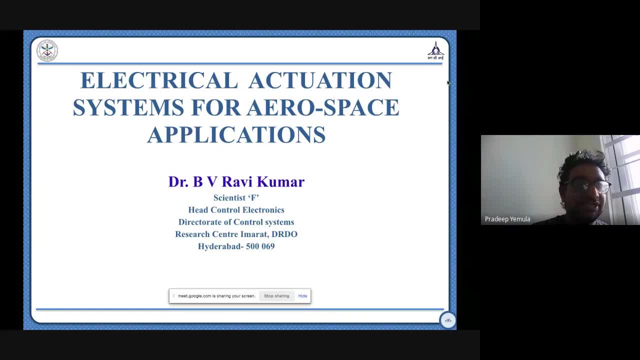 actuation systems for long-range guided bombs. so with this brief introduction, i would like to pass on the floor to dr ravi kumar to conduct his presentation, and we have a good number of students joining us, both from power electronics background, power system background and also. 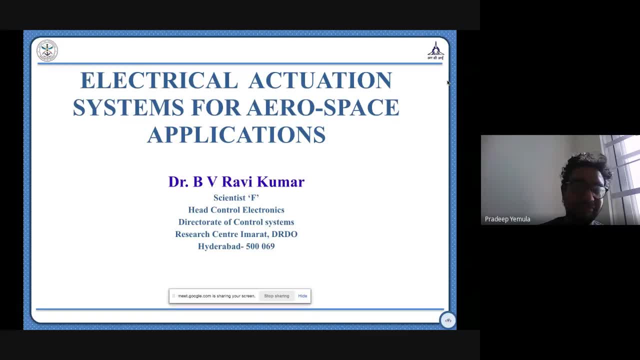 i think a few of the students are from different other backgrounds across the iit hyderabad. so with this, uh over to dr ravi. thank you very much, dr pradeep, for the introduction. so it's very. i would like to first thank dr pradeep for giving me this opportunity to share my experience and whatever. 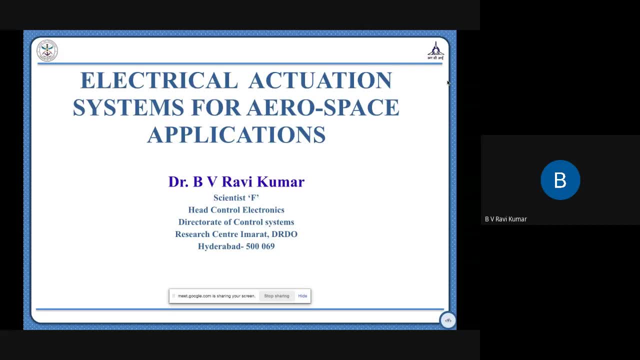 work we are doing in the missile area to especially for mtech, power systems and power electronic students, because always cherish, uh like it will be a pleasure for me to share with youngsters, especially because it is a. it is very much required for our country to make our technologies in-house and make an india policy, which our prime minister also 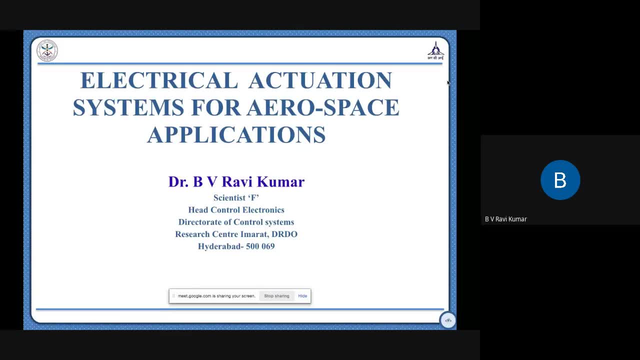 is more on that. so, and once again, thanks dr pradeep for the introduction, so i'll just go to the presentation because, coming to the topic, in fact i want to give more on the related to electric drives but i could not find time and whatever slides i have prepared for actuation system and 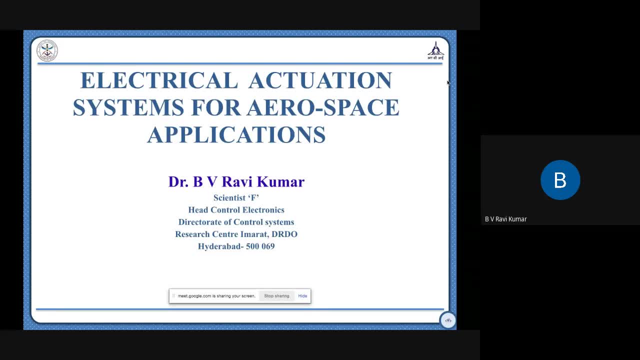 sharing with you. probably during the discussion we can have more information and i want the session to be more interactive. and as a power electronics mtex probably, you have a lot of opportunities, especially in electric vehicles and aerospace applications. in fact, aerospace applications- very few industries are there which are working in india especially for aerospace and we are depending. 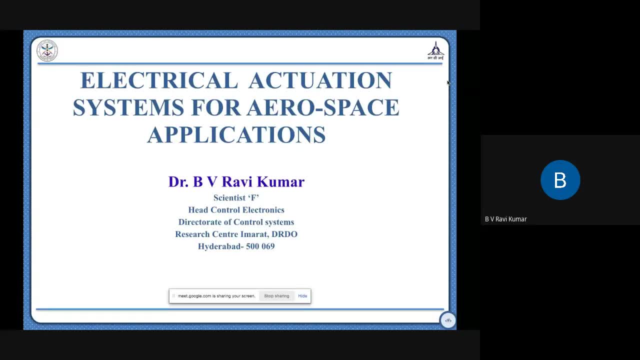 a lot on the abroad for importing a lot of technologies. instead of that, we can have our own technologies and our own people who are graduating from iits and nits and other good universities can work along with this in these applications and can make india this, make india dream true. so that is a concept behind 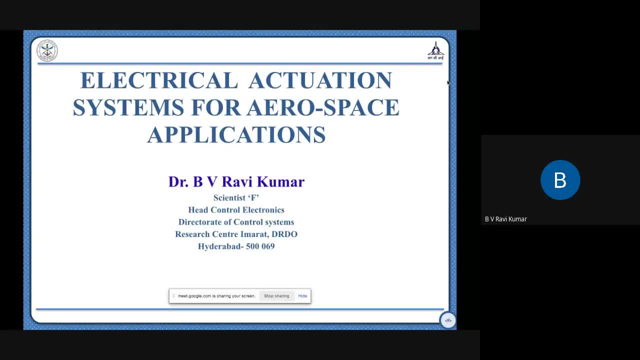 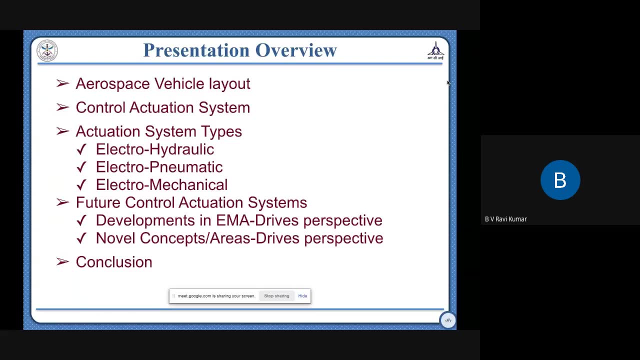 sharing with you all these concepts, so i'll just go through the presentation. so, coming to the presentation, i'll just first initially give you about the aerospace vehicle layout, because most of the people probably will be the industries. you will be knowing what is going on. but in aerospace very few literature is available and very few 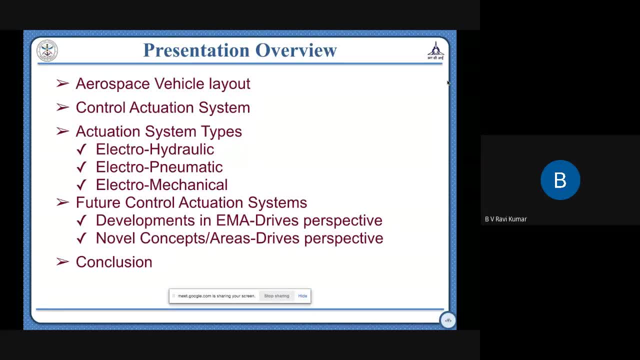 application oriented technologies will be there in internet. so i will be sharing some of the things which are from the drives and the powertrain point of view, even though power systems is a one of your core area i'll be touching, because we will be dealing with only powertrain and drives, so that 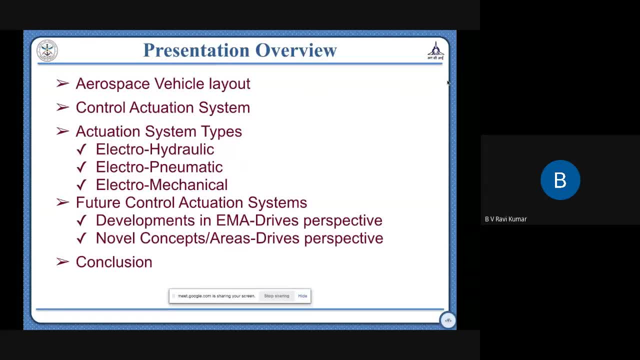 area will be stressed more and i'll just tell about the control action system. what is the design things, all those things that i'll just briefly go and not go in depth, and i'll just talk about the. what are the different actuation systems? like the years to be here, i think, from past. 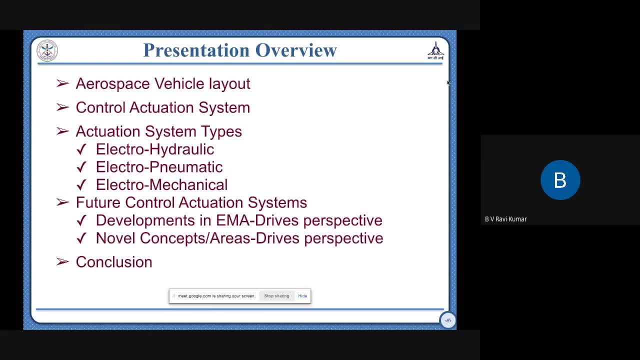 56 years we were working on the missiles and we are doing a lot of aerospace vehicles and space cycles for ISRO also. but there are a lot of evolution in terms of action system, So that I'll just touch it like electrohydraulic, electroneumatic and electromechanical. 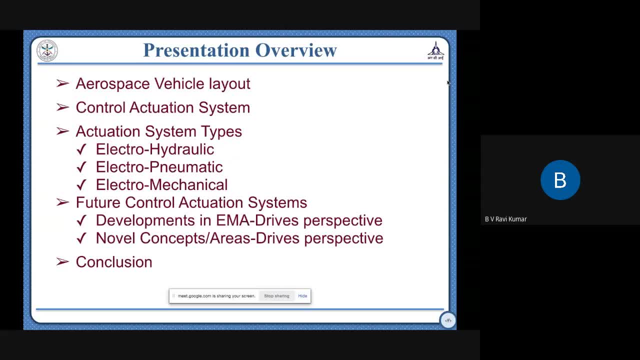 So electromechanical thing which I'm calling as electrical also because it is more towards electrical. So there comes all the drives and power electronics concepts, So that I'll stress more, And next comes to the future control action systems, which I want to especially you youngsters. 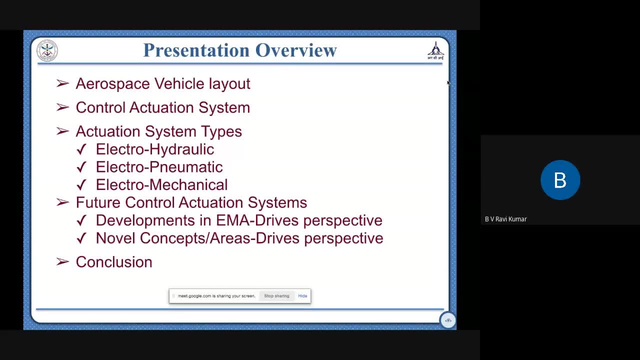 has to come into that area, because whatever has been done till now it's almost proven and has almost become absolute in terms of research. but there are a lot of area in which, by combining with other divisions of engineering, because now we can say there is no core research- 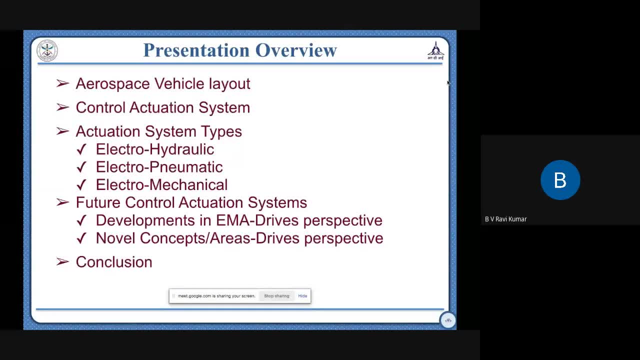 In fact we can say it is always a multidisciplinary requirement is there, whether it's a control systems or power electronics or drives, a power electronics alone may not help in a complete analysis, So it's a combination of all. multidisciplinary knowledge should be there. 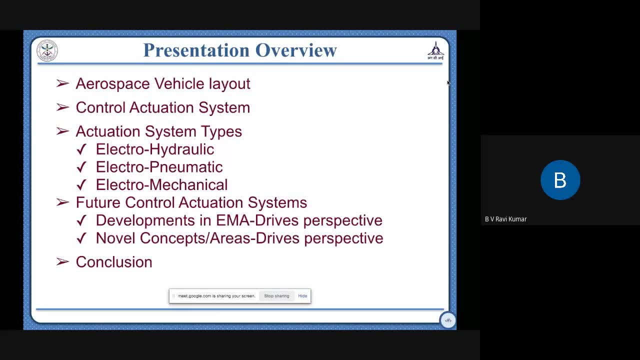 So that's what I'll be touching: some of the topics in the EMA drives perspective, the future requirements and also some novel concepts and areas. In fact, there are a lot of things which I can talk in terms of applications in aerospace. 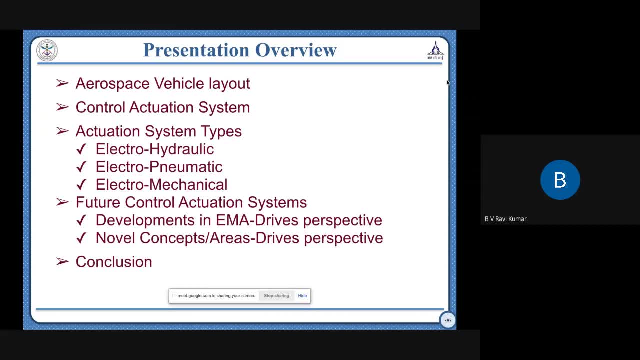 but I confine myself to few of things. few of them. One is because of the time restriction. Probably next time, if opportunity comes again, we can talk more about in depth design details and in depth We can talk about configuration requirements and constraints about electrical machine design. 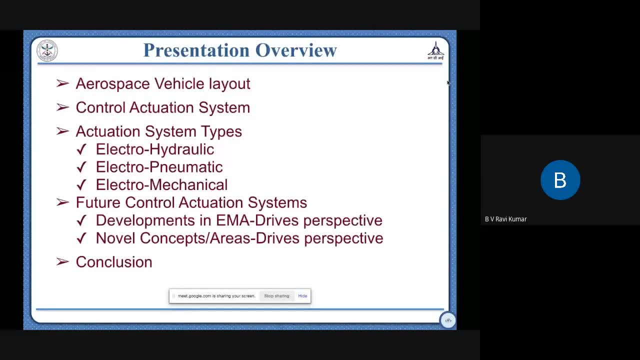 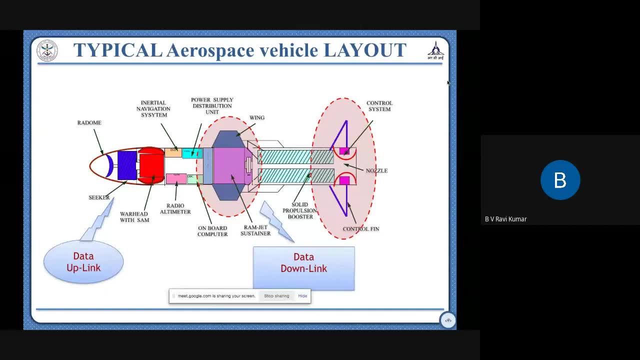 and as well as power electronics for aerospace vehicles. So this is how this presentation is made. So, coming to the, we'll start with aerospace vehicle. Basically, whatever aerospace vehicle I'm talking can be an aircraft, can be a missile, can be a guided bomb, or it can be a launch vehicle. 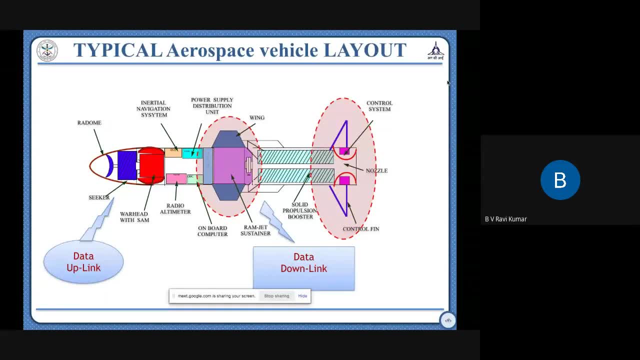 But specifically since I am from DRDO, which is a missile complex, so I'll be more stressing towards the missile. But as far as the actual system is concerned, it's a missile, It's a missile, So it's a missile. 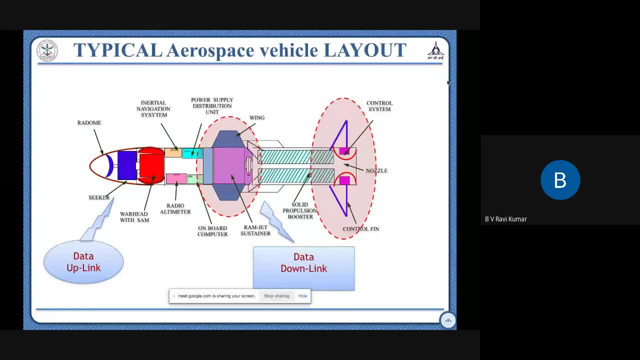 So, what it's concerned, whatever type of vehicle it is, the requirements remain same. Probably some constraints may be different from different type of application. So this is the layout of aerospace vehicle where you can see there are major things. We can say three things. 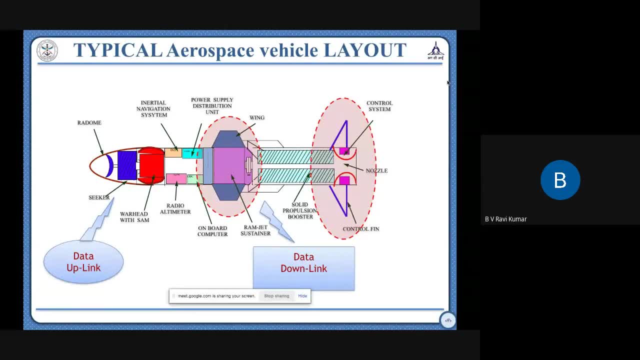 One is the propulsion, guidance and control. So these are the main three heart of any missile system or any aerospace vehicle. So propulsion comes to the chemical propulsion, what normally used in all missiles, whether it is a liquid, Liquid propulsion or solid propulsion. 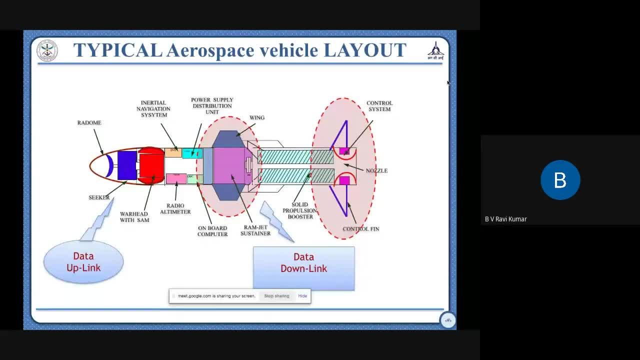 So next is the control. There comes the actuation system. So here in this figure you can see the fins which we are calling as a control fin, which is nothing but which will according to the given command from the onboard computer. it. 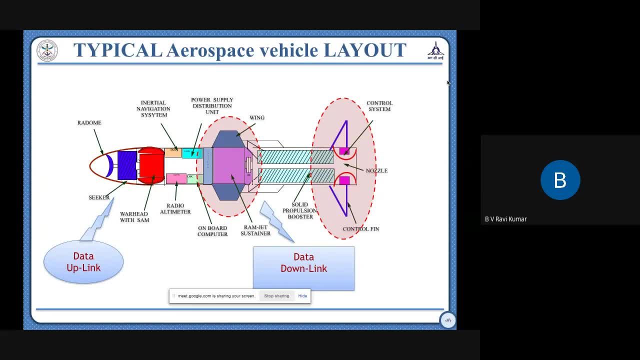 has to generate the deflection in order to give the control force by which the vehicle will be moved as per the desired trajectory. So that is what the function of action system, which is a very important, and there lies total power- electronics drives place A very important role. 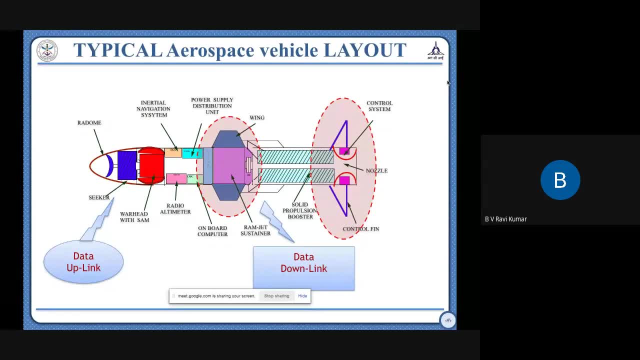 And in fact we have a lot of opportunities in from aircraft industry also, which I'll be coming in terms of technology, What are the opportunities and what are the limitations and where we can improve. So that area also I'll be talking. So that is a control system and comes in between. 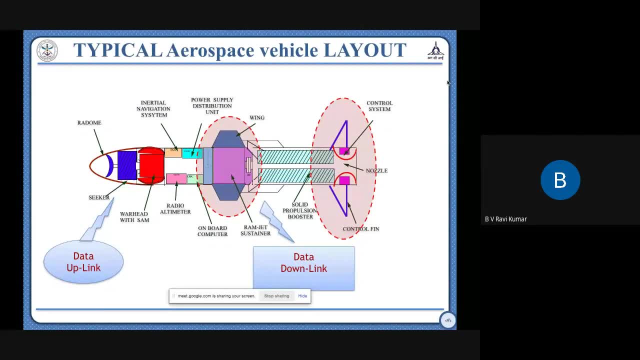 We have a guidance. Guidance is nothing, but what is the algorithm required to control the vehicle? whether it is a proportional navigation- PN guidance- or whether it is a homing guidance, where we will have a active sensor that is seeker, which I am showing in this slide. 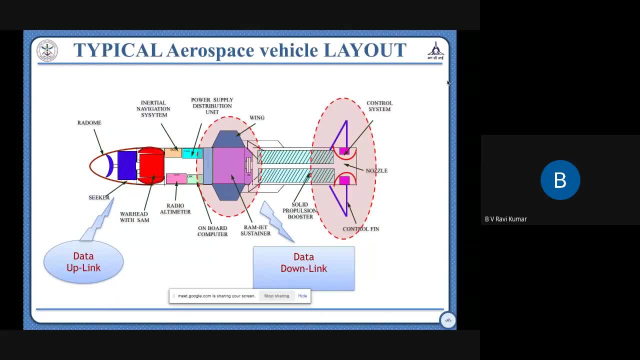 So that is a sensor. Basically, the guidance algorithm depends upon what type of target it is. Is it a moving target, Is it is a standstill target or is it a very slow moving target? So such type of things comes under the guidance algorithm. 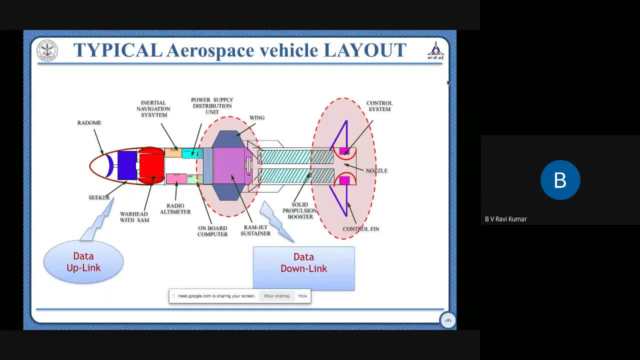 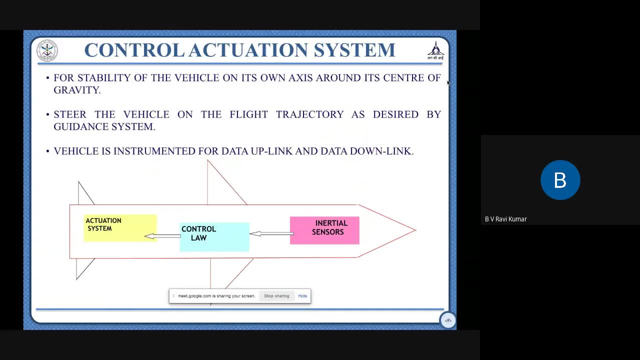 And next comes the. that is what control system, propulsion, guidance. These three are the major, important parameters or subsystems in any missile or, of course, aerospace vehicle. Now it comes to the control action system. So we could have seen in all our control system books in BTEC also we have used to see in 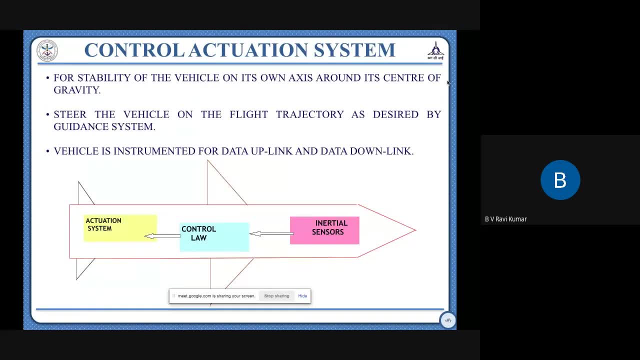 I think in second year We will send it somewhere. we will be having a we're, a controller- Sorry will be there- through which our action system should be controlled, based on the inertial sensors- The data will be there and, based on that action system has to move in order to move the total. 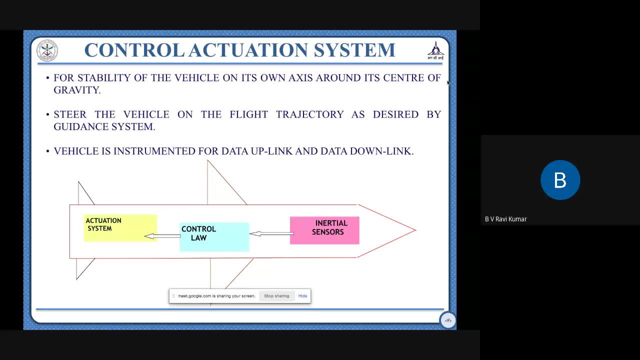 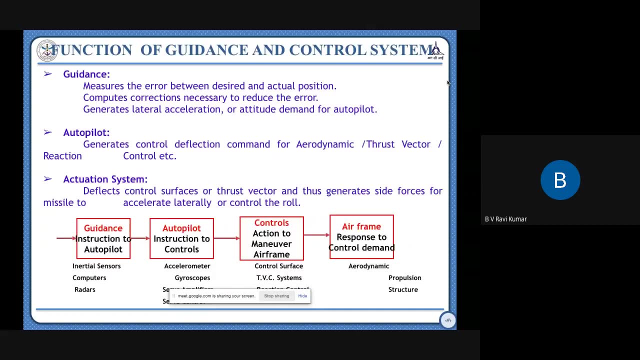 vehicle. So that's how the control system requirement. So the control system requirement is to steer the vehicle on the desired project. So it's a very thing- I'm not going in depth about this- And of course, the guidance function also. we all know it's. it's nothing but it's measures. 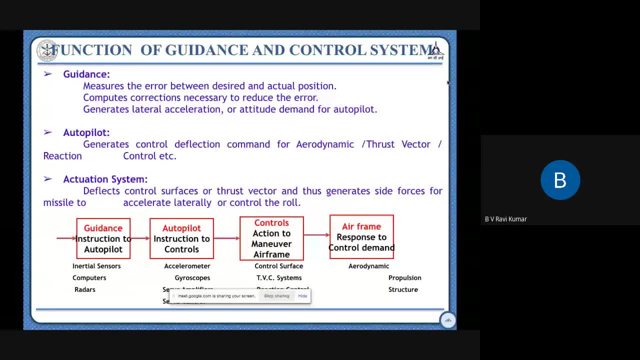 the error between a desired and actual position. based on that, it comp. it computes what is the necessary command required to reduce the error based on which the actuator moves and, finally, it corrects the vehicle attitude. so that's what i've written here. block diagrams. now coming to the in-depth explanation: guidance. 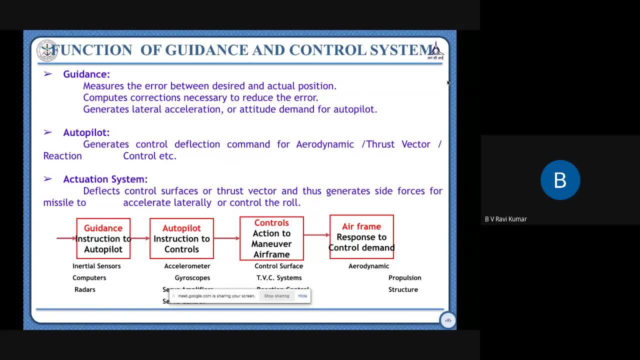 autopilot will just forget. we'll come to the controls. the main action of the control is to maneuver the airframe that is a vehicle. so what are the different control surface? we have a pvc action systems and we have reaction control systems and we have aerodynamic control system. 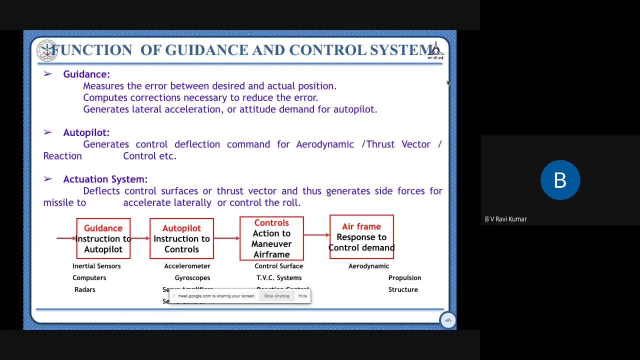 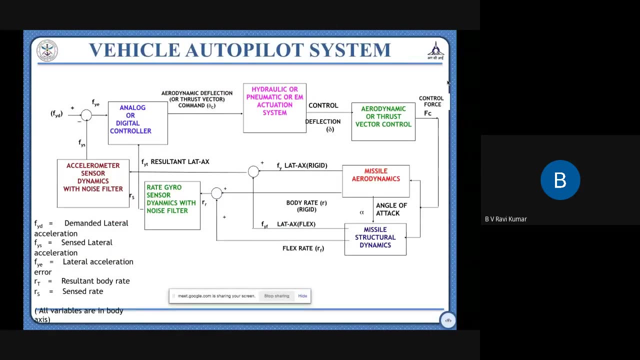 that is what airframe. so the aerodynamic and thrust vector control are the two control systems in which we use actuators to control the vehicle in its desired to move into its desired position. this is a brief vehicle autopilot system where this is a control autopilot system of a missile. 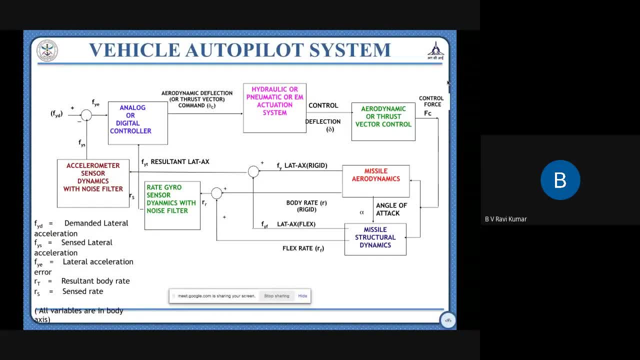 where we have a rate gyro for taking the rates and we have missile aerodynamics from which the structural dynamics will be acting and from which the airframe dynamics will come into the picture. so this is a control block diagram of complete vehicle and where the actuation system is inner loop to it, that's what i'm showing here: hydraulic or pneumatic or ema. 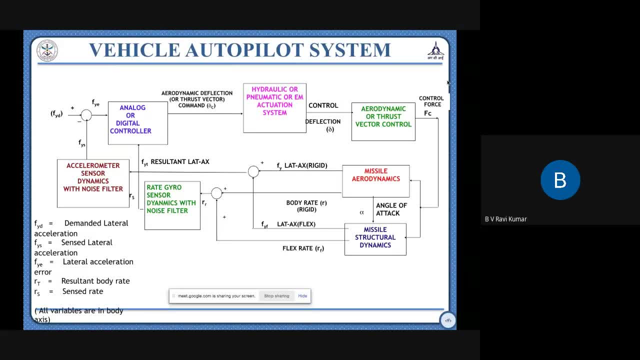 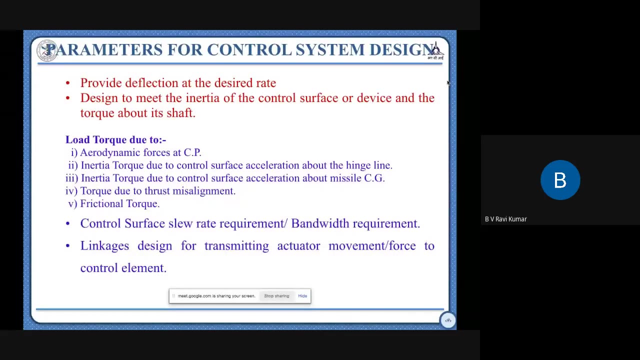 it's an inner loop to any vehicle missile system. that means it is much faster system. suppose you want to control vehicle to go to your desired target. your action system should be much faster than your outer loop, which is our guidance. so now we will come to what are the parameters for. 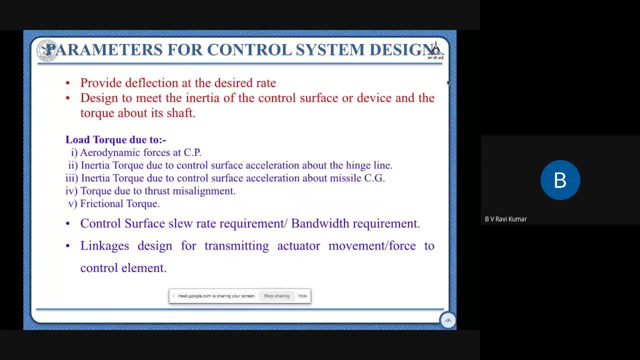 the control system design. so that also i'll very briefly i'll go about it. so, where we require a lot of aerodynamic forces, what is inertia? all these things i'm just bringing to you. you will notice that because the design of an action system which is nothing but from electrical point of it's a design of 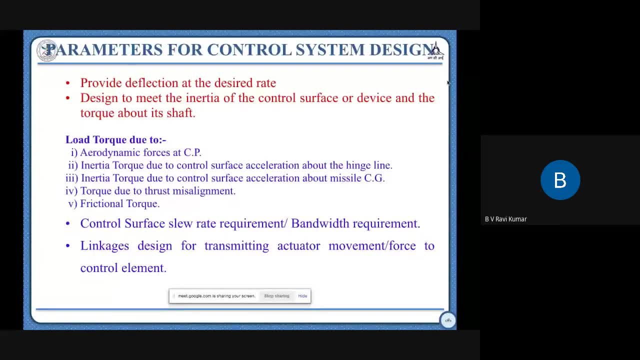 a brushless dc motor or any motor. it's a prime mover, basically, and it's power, electronics and control systems. it is equivalent to any industrial application, but there is a difference between industrial application and an aerospace application. so for that purpose i just want to bring you as a 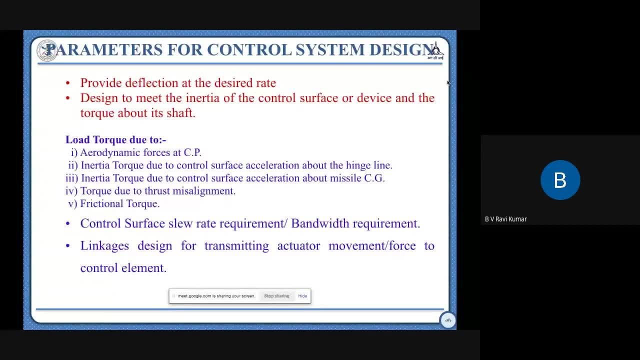 little bit more into the actual discussion that what is the criticalities and what are the main parameters for every design. so if you take, the major thing is the aerodynamic forces. so this is a very important parameter because the forces are varying, because if you are moving a missile at a 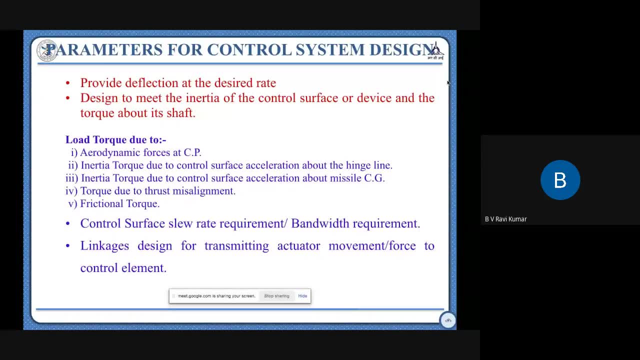 very high velocities, because now everyone is speaking about hypersonic missiles. so tomorrow we cannot rely on a simple missiles or a supersonic or subsonic missiles. we have to go for hypersonics so that our enemy should not be able to detect us. so that's what all we are. 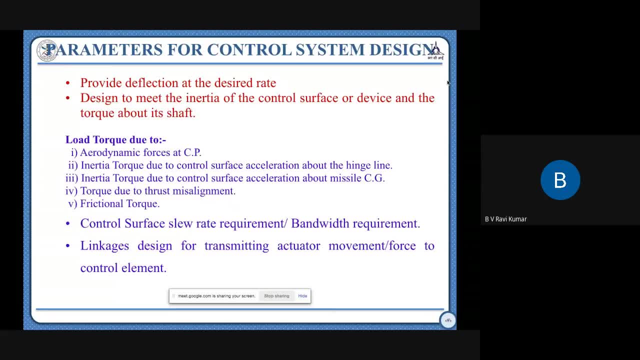 talking about hypersonic, which is the next generation technology- require very high aerodynamic forces on the missile. so your actuation system should be able to control that force, because you have a huge loads on the fins so you have to overcome along that load. so your motor design, your power electronics to handle that type of currents. 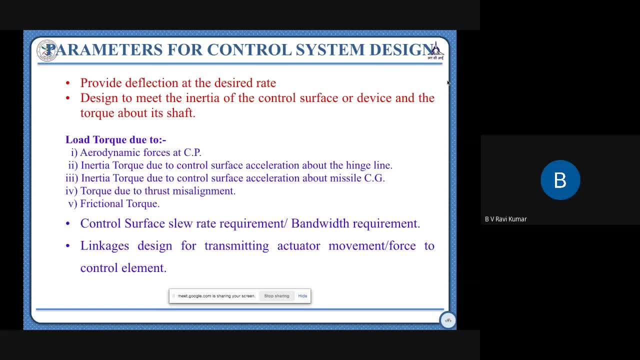 and your battery requirements. all these things matters a lot, so that is a major thing. that is, aerodynamic forces, which will be varying with respect to the time. at a very faster rate. the load is also not constant. and next is inertia, torque. inertia, torque is coming from the 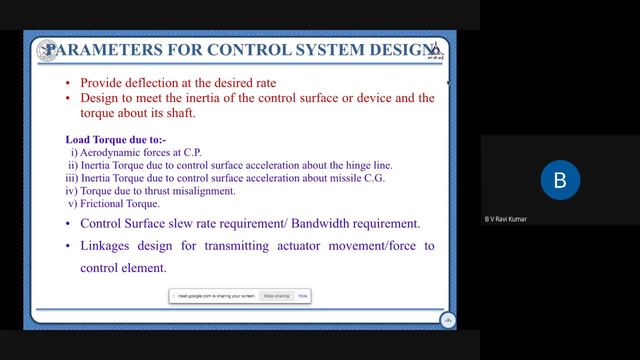 fin surface. you may have to use a very long control surface to control, which will add the inertia onto your motor because of your control system. characteristics will change and of course inertia, torque due to a controlled surface, acceleration about missile cg because the total missile is also moving, so that inertia will also come as a part onto your actual inertia. so all 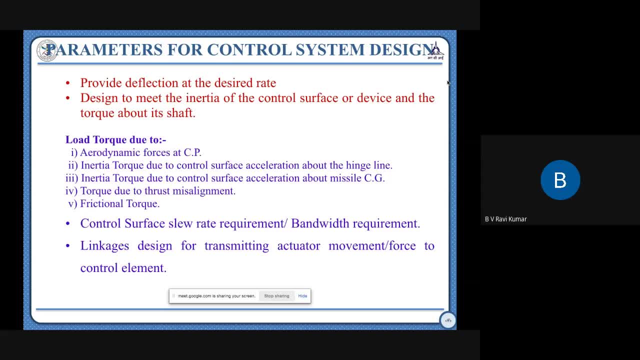 these things are the major parameters which, first of all, it's not standard- depends upon the missile aerodynamics, it depends upon the missile velocity, depends upon the missile maneuvering. these things are input to your load from which you derive what is the motor torque requirement. and, of course, another important parameter is a surface slew rate. slew rate is the rate at 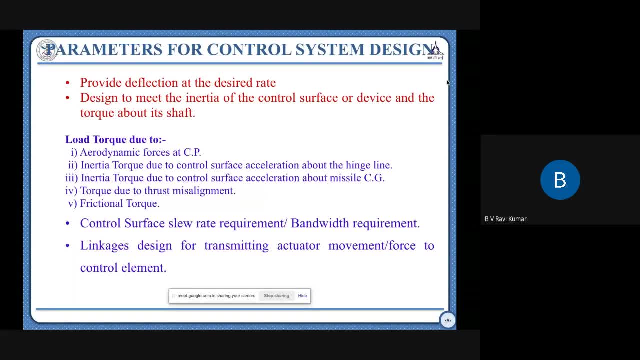 which you are able to correct the control system. so then, bandwidth requirement, so higher the maneuverability of the missile, your high bandwidth requirement which, again, it's a very important parameter for your motor design, for your power electronics design and control system, where you should use all the current control and flux weakening control techniques. so that's what. 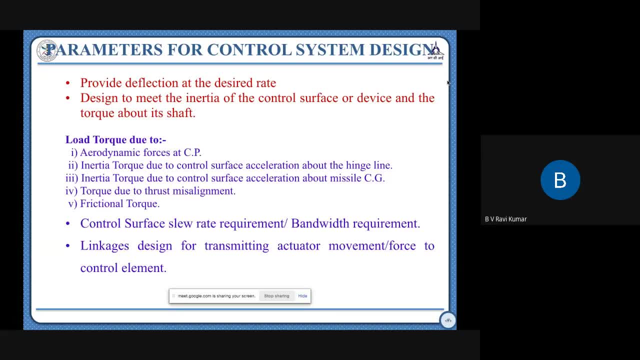 we are studying as a part of mtech curriculum. in terms of power, electronics and machines, they are definitely and very much useful and very much applicable for all our aerospace applications and it is very much improves the performance because still now a lot of hydraulic systems has been using in the aerospace vehicles which are. i will show the disadvantage and definitely 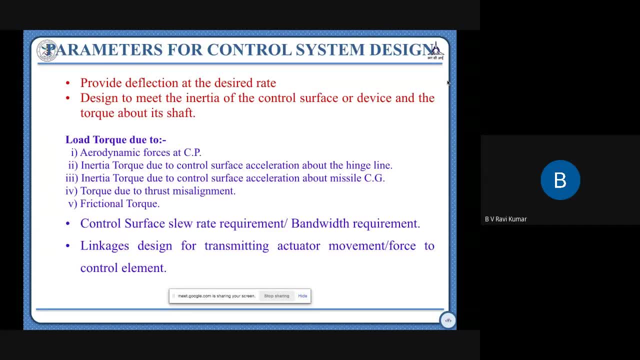 electrical actuation systems are the requirement of the day, for missiles anyhow, we are already into that, even for aircrafts also. people are going to the all electric aircraft where you will be using all the electrical elements and then you have the complete electric motors for propulsion where you could require multi-phase machines, where you could require inverters, with all. 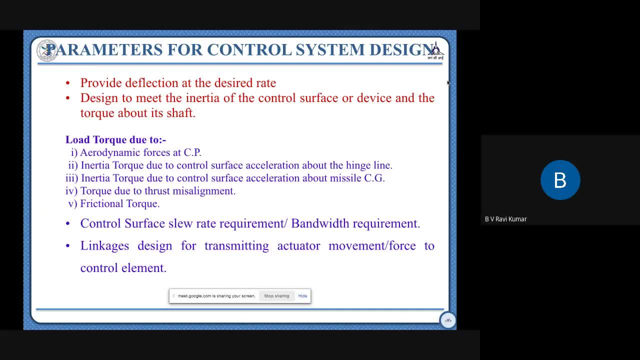 fault diagnosis. it's a lot of huge requirements out there and use technical requirement is there, and especially india, if you see a lot of power inverters. even though we speak about a lot of configurations and a lot of things, we are always buying, depending on the outside world for some of the equipment to be imported, so that all we can overcome by doing. 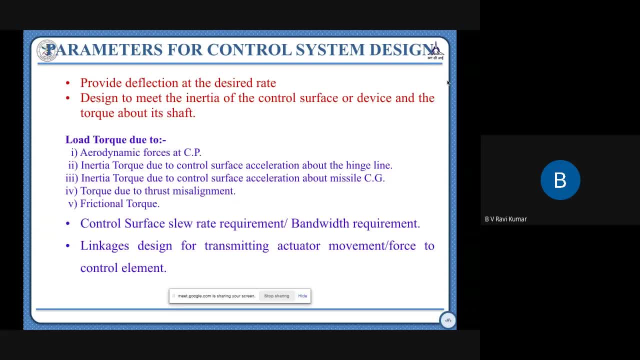 we studied, we can just apply as an application and we can overcome all those issues. that's the reason i'm just going in depth about this slide, where i want to show you that these are the actual requirements which has to be taken in the design and by our application of power electronics and 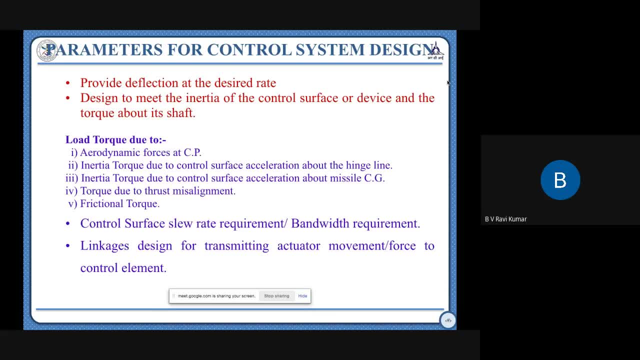 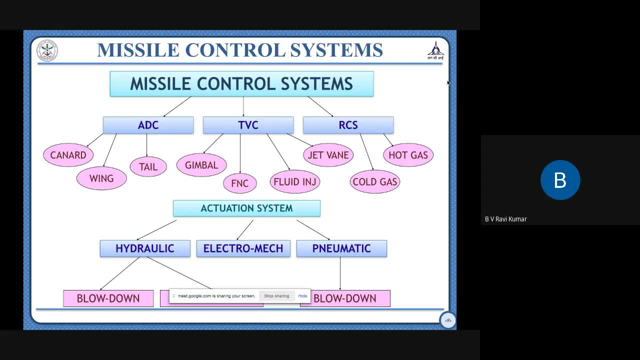 drives. you can overcome all these things. and just this is overview, because you should know what is a for any vehicle. this is not only for a missile, because normally for any aircraft- even it's a fighter aircraft also- you have aerodynamic control, thrust vector control and reaction control system. 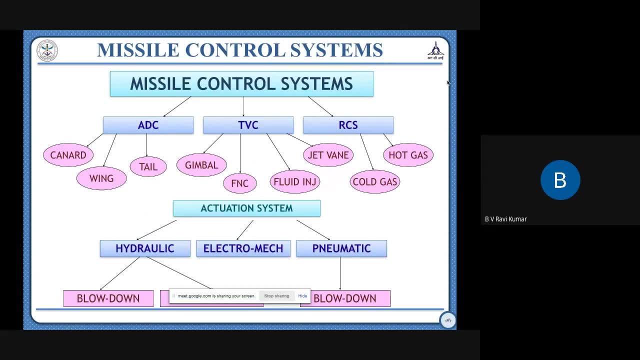 so reaction control system is a very interesting control system which i'll show in the last of my presentation, where i'll show you a video also where we have done something with respect to very small improvement with power electronics where we could achieve a lot of improvement at. 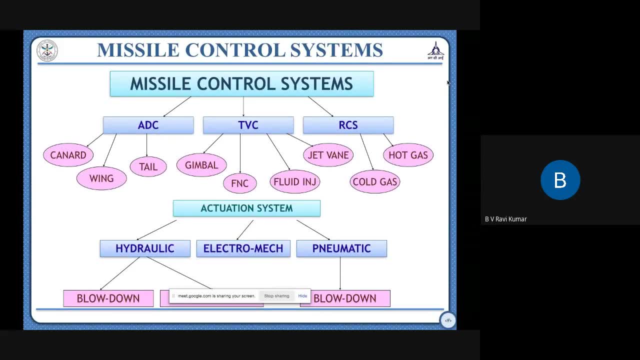 vehicle level, so that i'll come to that. so normally the action control system will be used out of atmosphere. next is a thrust vector control. where is nothing but we use the thrust vector, will change in order to change the direction of the missile and is aerodynamic control by the velocity. 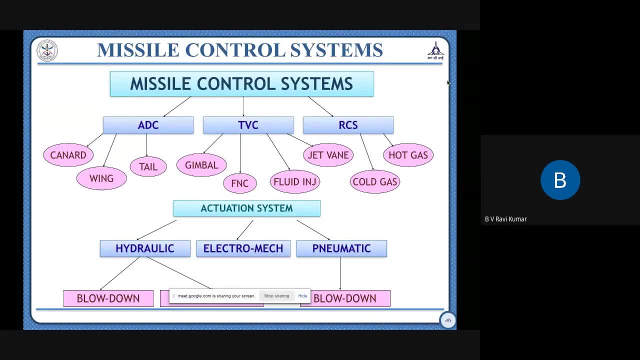 air which will act as a. from the aerodynamic pressure, the force will be exiting on the fins. so by changing the fin direction we will change the steel, the direction of the vehicle. so these are the three different type of control systems normally employed in a space vehicle or missile. 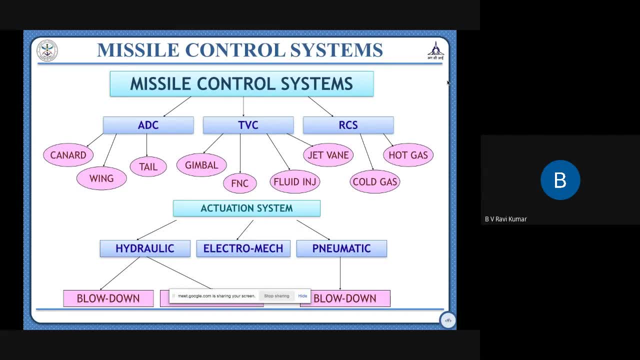 so next comes to what type of actuation system. so we have a hydraulic, electromechanic and pneumatic. so hydraulic pneumatic, i'll just very briefly one or two sides i'll just show, and we'll directly go to the electromechanical, which is nothing but electrical action system which i'm talking. 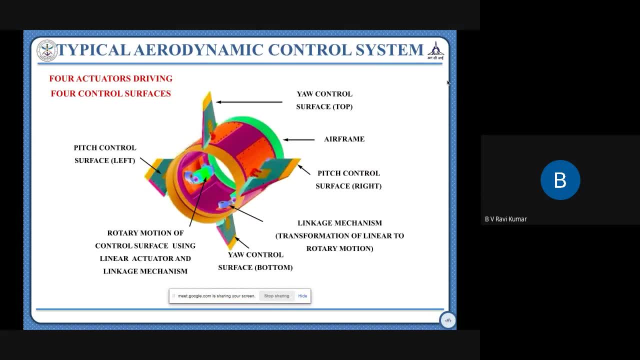 we'll concentrate on that. this is um, just because just dr. this is pradeep. uh, sorry to interrupt. yeah, so i have just a brief uh observation. yeah so, uh, uh, your presentation started on a very interesting note and it's going fine. yeah, now my question is: um, some of the things that you are covering today you might have picked? 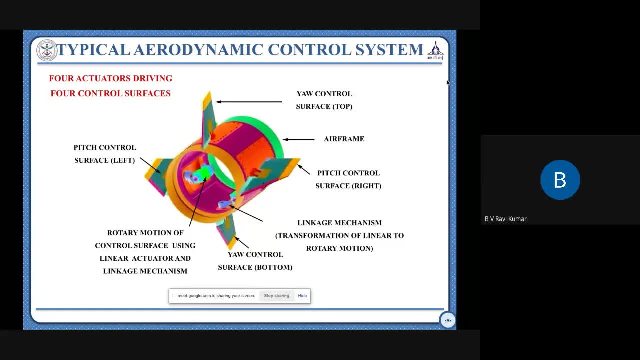 up or learned from your organization, right. so? so for a student in a institute like you know- iit, hyderabad, or any uh institute- see some of the things that you are covering today- you might have picked up or learned from your organization, right. so some of the things that you are covering today, you might have picked up. 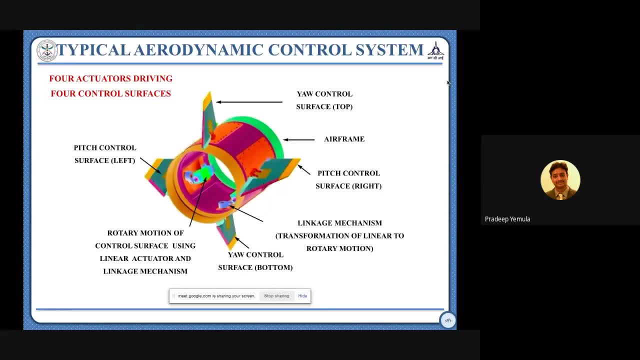 these things. you know how they will learn uh like. is it like after joining an organization they will have to pick up these things, or uh at the stage of uh being in academics? only how they can get this kind of uh exposure to in-depth things. so can you throw some light on that? i don't know. 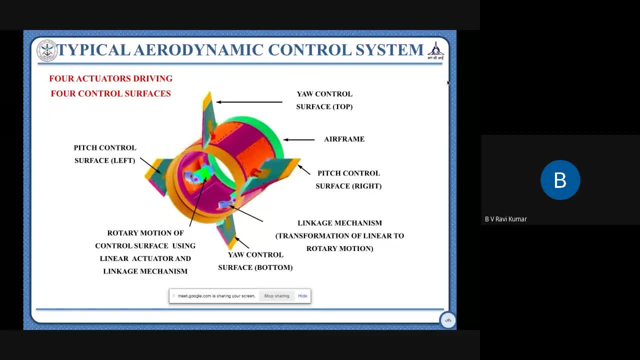 whether i'm making sense in asking this question, but i hope you got the language i'm asking. it's very valid question. actually, as you said, it's rightly for a poletonics or electrical engine. i i've given you some examples, but i think that i i had to make this point. uh, and that's okay. 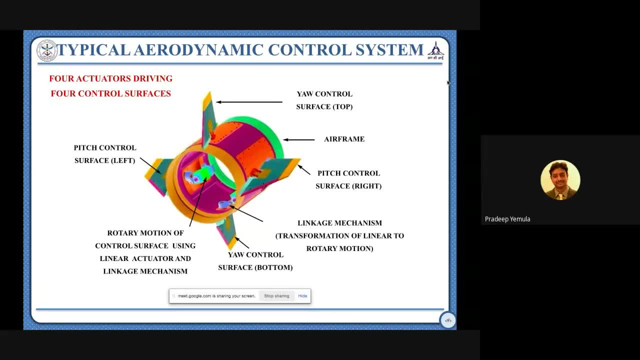 if you're interested in going to a non-athletic institution, it's very easy to come over and just learn from a lecture. it's very easy to come over to a non-athletic institution and see the kind of uh that they're interested in, while also it's yeah. so i think it's a very 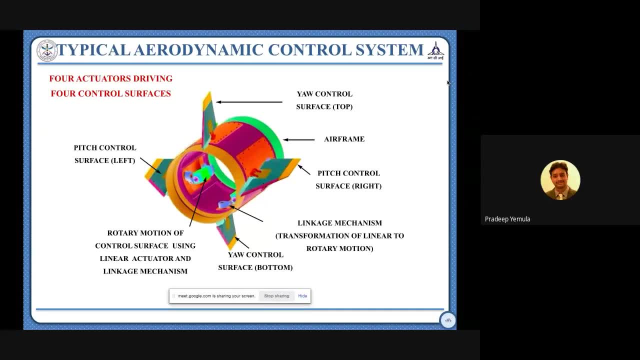 good idea if you were to have a lecture and come over and see the kind of- uh, technical stuff that you have to learn from i. you know some of the components you just discussed, like the, So so, yeah, I'm sorry I interrupted, So you can. 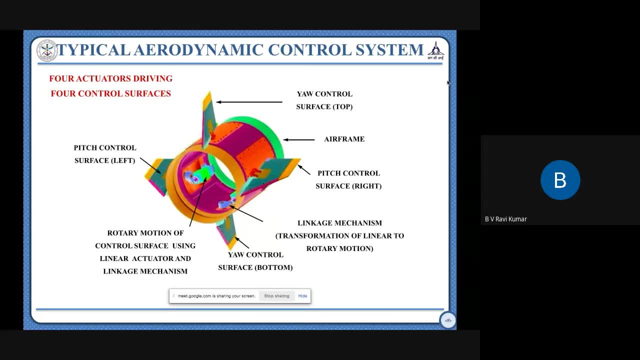 It's a valid point what you're telling, but it's, it's exactly right that normally this will come from the industry application only. But if you look into it, whatever I'm presenting, what I'm showing, the ultimate, if you go in- 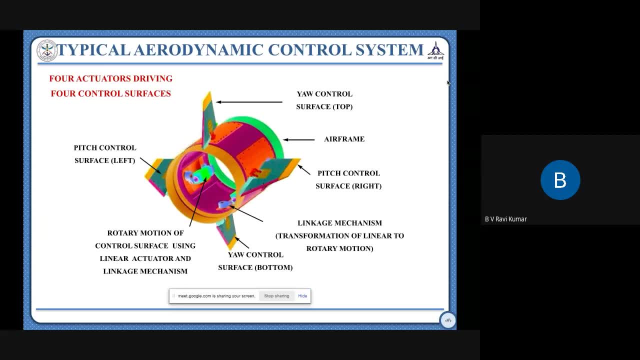 depth design that finally comes to whatever you're teaching. only what I think, because this is an application orientation. My application may be this, but as an as electric vehicle industry, the application may be different, But ultimately, once you go in depth design, it will come to definitely whatever we are. 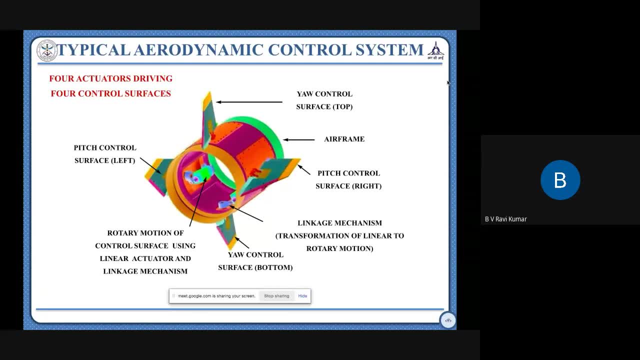 learning in the electric, for example, mathematical modeling of electrical machines, what may be probably one of the codes you're having. definitely that is a base for all these things. That's what I will come to them. This is maybe at academic level. we may not and it's not. I don't think it is required. 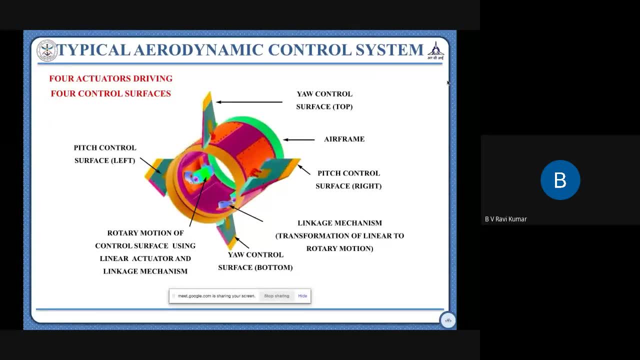 also means if you're doing for a power electronic subject, definitely we don't expect you we to have in details about this application, because applications are vast, we have different industries having different applications, But what I mean to say tell is ultimately the all the applications, the root cause will. 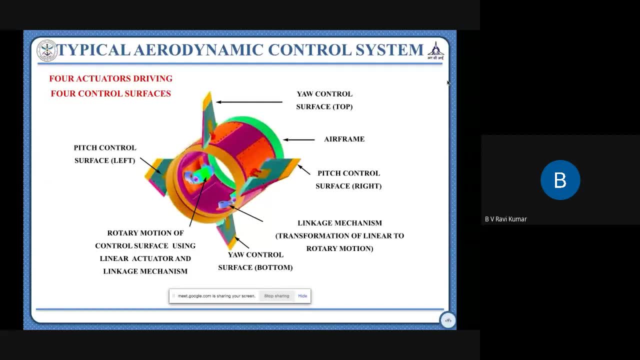 be from the basic. suppose if you're using a machine for an actual system, the basic equations comes from whatever you're having, you're covering in the academics. So it's only application part which normally it comes as a you join an industry or that. 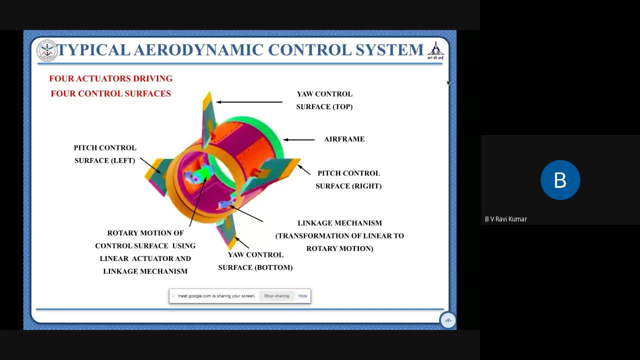 thing That we don't expect in academics. So I don't think that is it means it's not very much important. also, we should be like: this will definitely connect the real world with the academics world, So that's why it is very important. 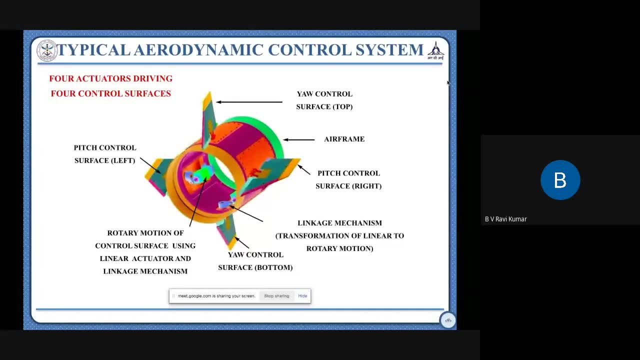 So yeah, please, Actually, yeah, what I what I mean to say is whatever we are covering in the academics, they're very much important. Only thing is where to apply them. So that application will come based on the industry, what we are working. 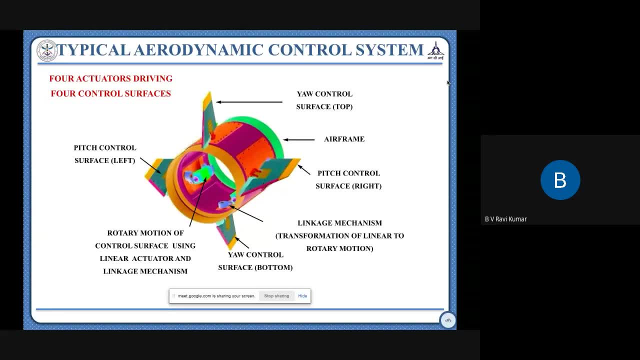 So that is that. So this is the four actuators running control surfaces. So just to just to have a view, like how an arrow aircraft or a missile will have. So these are the four actuators which will be used for the role pitch and yaw control. 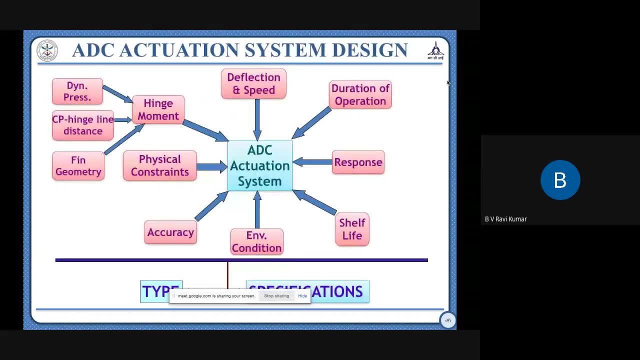 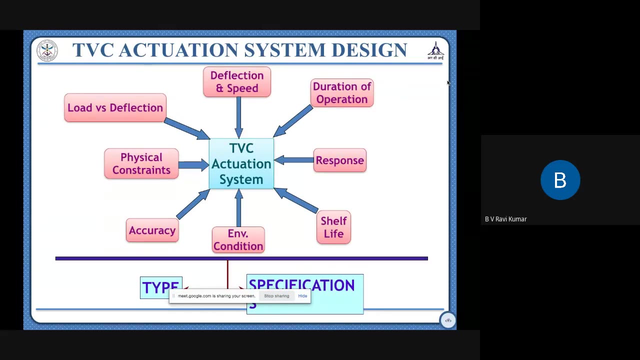 where we use actuators. So this is just a dissection system, having a different requirement, as I already told you, what is the deflection and speed accuracy. So these are the important parameters for design, often actuators. This is a thrust vector control, which already told you that. I will show some figures also. 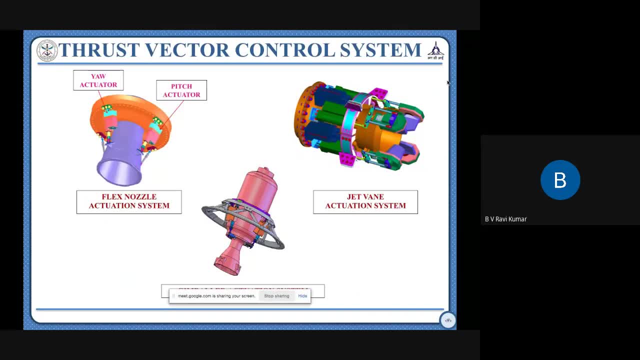 I'll come to that in that I can explain you better. So this is the figures. So if you can see first one, it's a flux nozzle control system. That means the flux nozzle is a nozzle from which the thrust will come out. 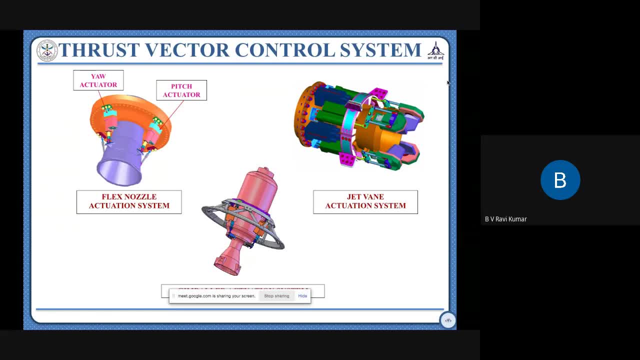 So you will have a rocket motor front of that and the propulsion will take care, will will happen and it just will come out of this nozzle. And these are the actuator which I mentioned: pitch actuator and yaw actuator. they will actuate, they will move forward and reverse. 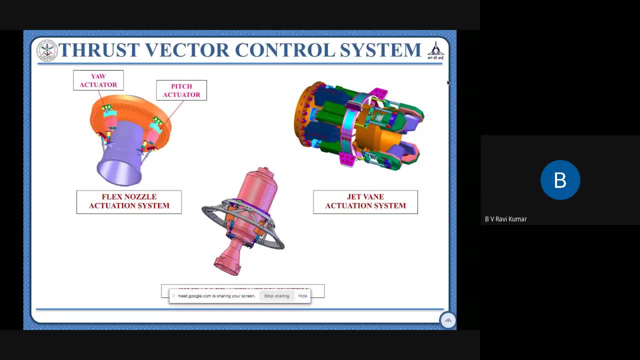 In order to control the angle of this nozzle by which the thrust angle will be controlled and thrust vector will happen and vehicle will move based on the commanded direction, So that commands will be given by an onboard computer based on the desired algorithm. And next one is a jet vane actuation system. this is also a thrust vector control one. 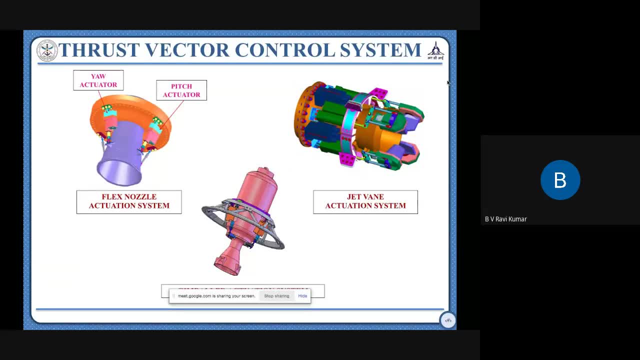 of the type of thrust vector control where you will use some vanes where the flow is coming out. the vanes will be controlled in order to control the flow. So that is done by actuators- that green one, what I'm showing. 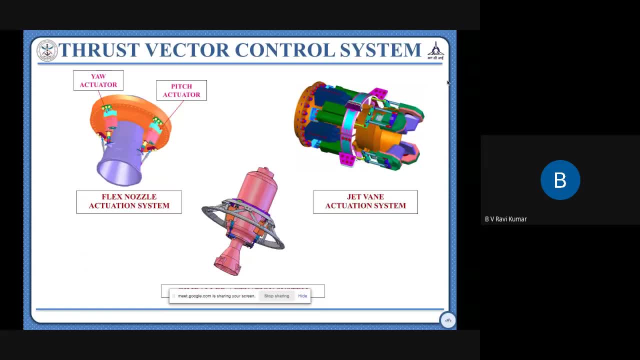 This is an actuator which will move, for these are called linear actuators. Similarly the last one, it's a gimbal rocket motor where complete propulsion motor will be pitch and yaw direction will be controlled And next comes a control system. reaction controls, normally reaction control system. 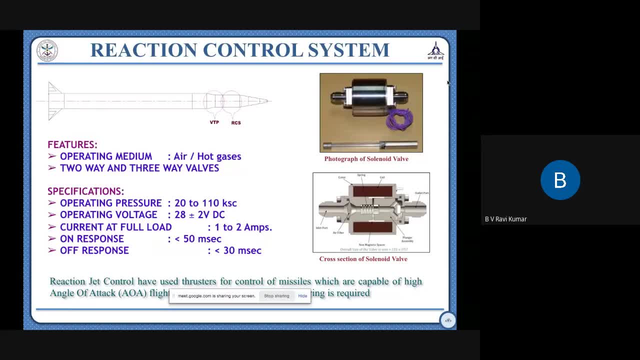 It's a. normally it uses a simple solenoid valve. but I'll just come to that, the last one. I already told you there is a huge requirement for reaction control system, especially in one of our application, So where It uses some power electronics controller. very small concept by which complete scenario. 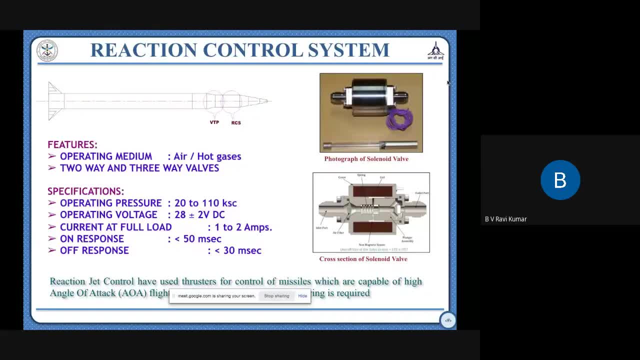 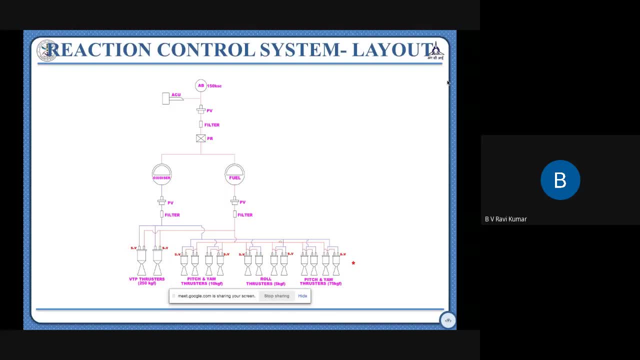 has been changed that I'll come to that. So this is a reaction control system where you have an oxidizer tank and a fuel tank and both will be coupled to produce the thrust. So valve is an electromagnetic device. it should be used for on and off. 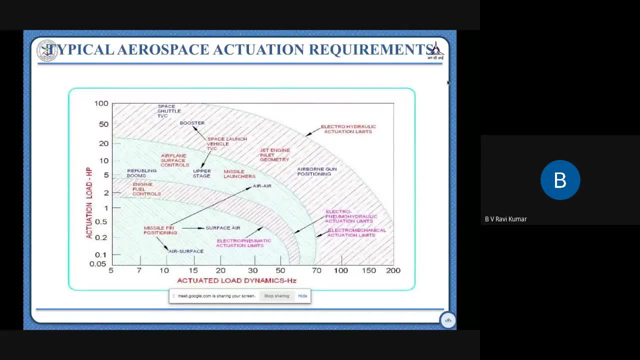 So this is the actuation load versus actuated load dynamics. So, based on the requirements, like why hydraulic action system is famous is, you can see the upper limits of electro hydraulic system. That means it can handle very high loads, whereas electrical actuation system it comes. 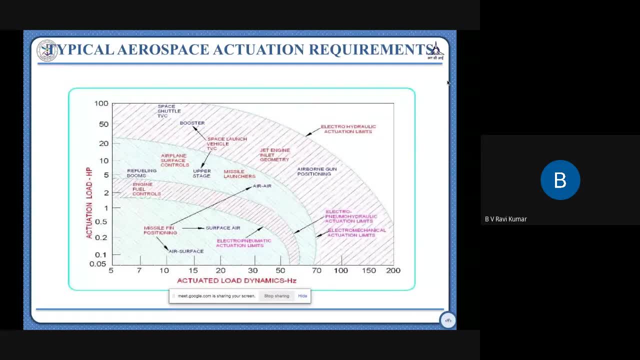 in between a very less compared to hydraulics. So there, the electrical action system is. one of the limitation of the electrical action system is it's load capability. Now the problem lies with the electrical engineers to make electromechanical action system more power. 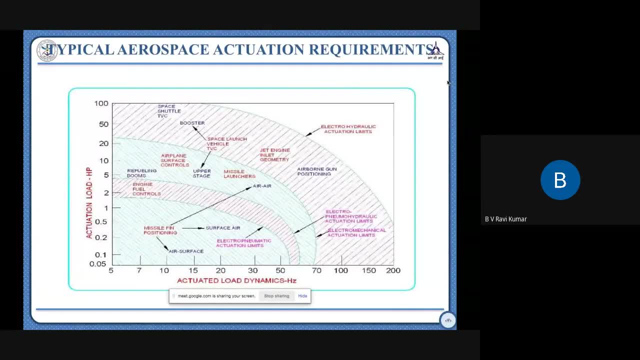 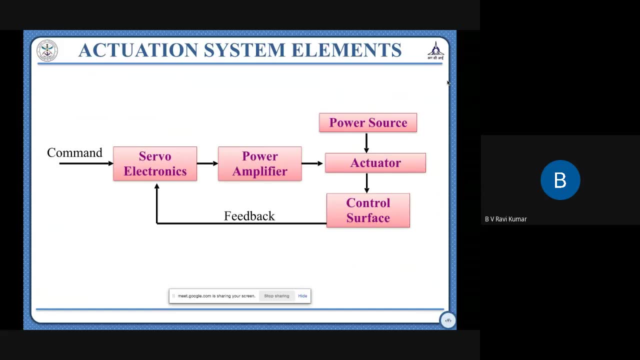 I mean more capability. that that is where the challenge lies. That's what I'll be coming to, that also, And this, of course. whatever I covered in the last slide, same thing, is summarizing here. So this is the control system. it's a very simple thing. we have a servo electronics. 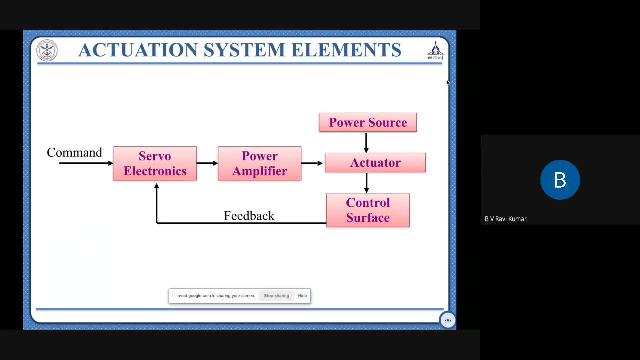 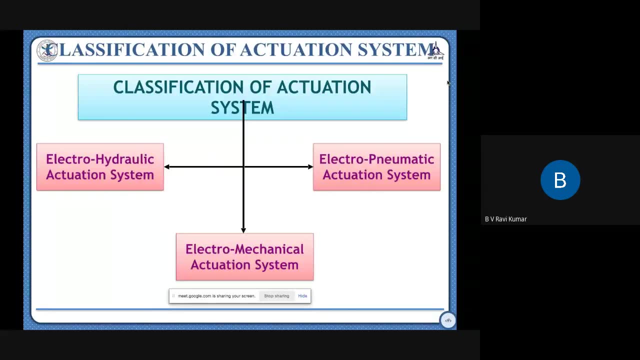 we have a power inverter for driving a brushless DC motor or a stepper motor or SRN. whatever the motor it is, it is a. we should require a power amplifier, servo electronics and it acts as an actuator. This, anyhow, this same thing. now we'll just, I'll just only. I will not go in depth about. 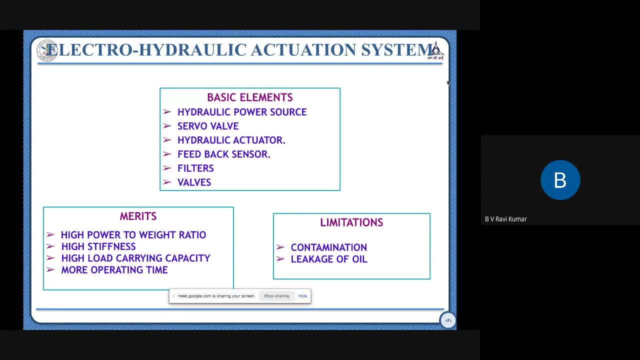 this, because this is not our topic actually. just I want to tell you what is the merits and demerits, because based on that we have to develop our electrical action systems. So the basic elements of hydraulics is: So this is the control system. 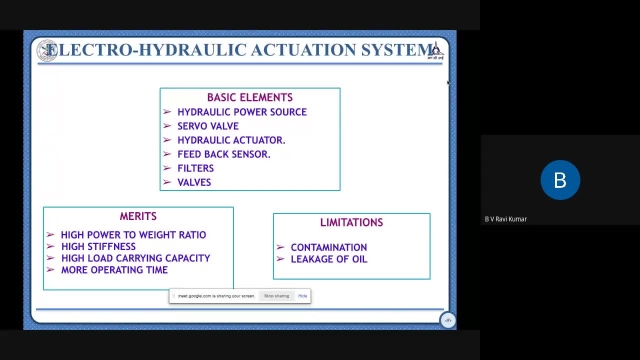 The main thing is we require hydraulic power source and they have. we have a servo valve And the main merits of that is it's having a very high power to weight ratio, And limitations are a lot of subsystems are there and it is continuous leakage of oil. 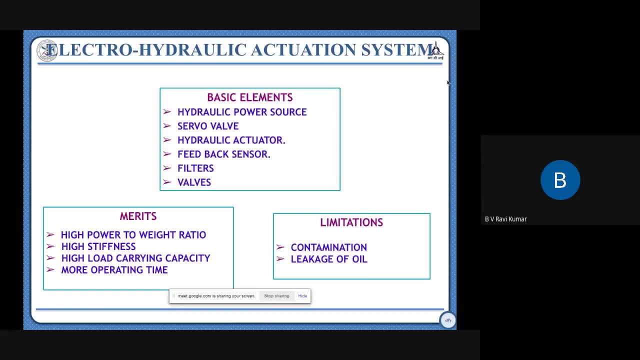 So it's a lot of maintenance. but all aircrafts, what we are flying- commercial aircrafts- use hydraulic actuators and all space vehicles- launch vehicles like PSLV, GSLV, first stages- they use hydraulic action system because of load carrying capability but they're having 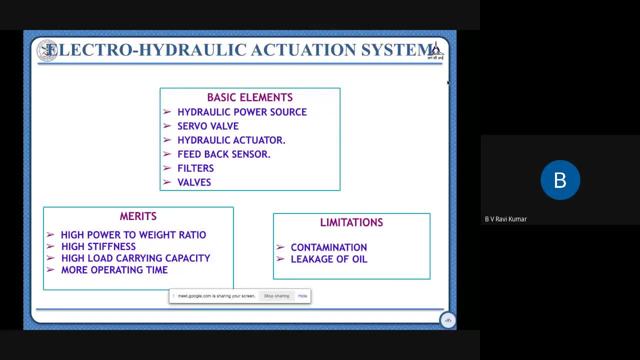 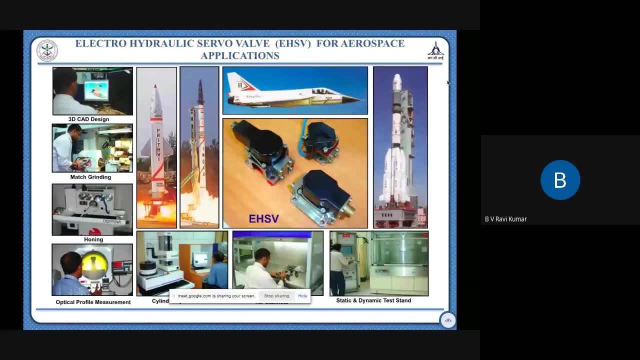 a lot of limitations. There is a contamination, leakage of a lot of maintenance is required. So this I'll just skip this slide. this also can skip it because it's about hydraulics. There's only some figures. I want to show you Prudhvi, which is our first generation missile. 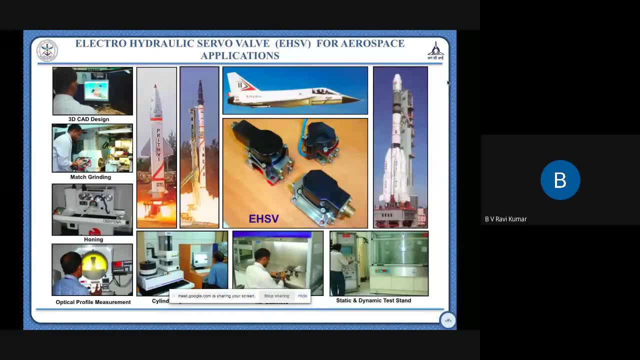 surface to surface missile which is using a hydraulic action system, Agni and the PSLV. These are all using hydraulic action systems where the heart of the hydraulic action system is a servo valve, which we are calling the electro hydraulic servo valve, which is the 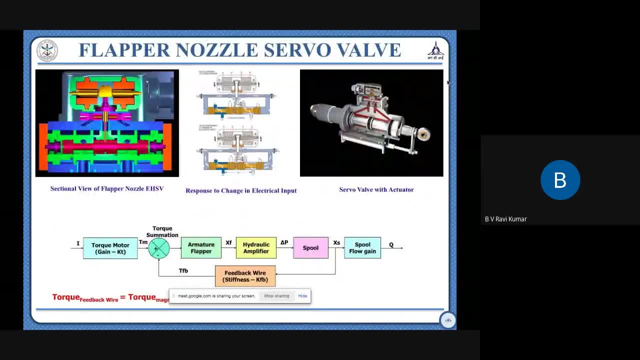 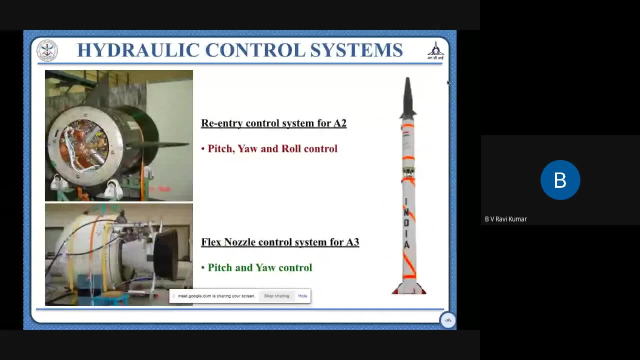 heart of an Hydraulic action system. So this is a brief construction in which it's also not very much relevant to our thing. So I can just only just explain you about this. I can skip it. So these are different hydraulic hydraulic systems for different designs. 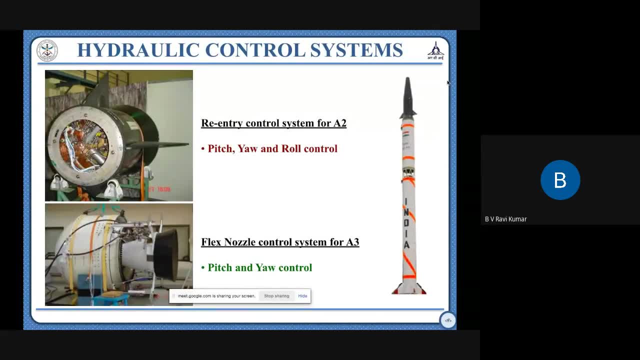 So these are just figures to tell you actual hardware figures so that you'll get a feel of how a nozzle looks. So this is the nozzle and in front of that is you have a rocket motor which is for different actuation systems. Okay, 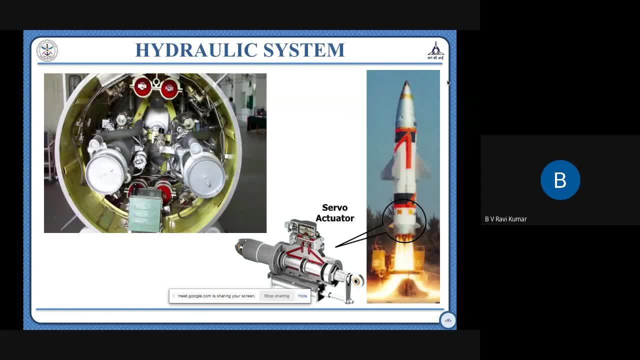 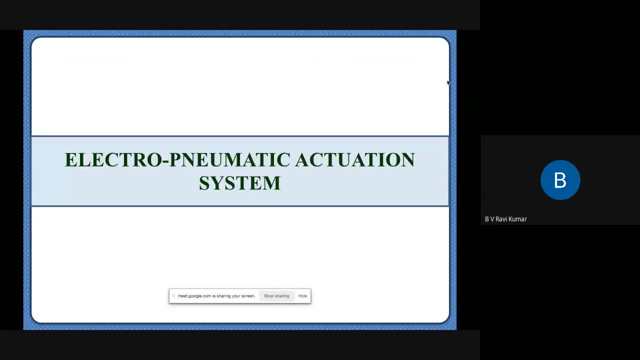 So this is a hydraulic action system where it is an actuator for actuating the engines. So this is the first generation missiles. what we have now we'll just go to electro pneumatics, which in fact we can tell absolute. we are not using in any of the missile these pneumatic. 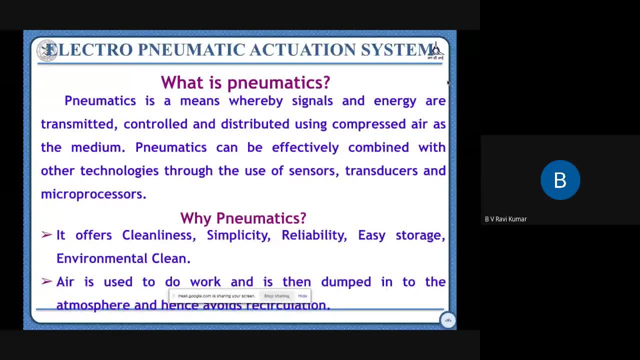 action systems because it also has same problems with hydraulics, But in fact it is much lesser- torque to weight, I mean. compared to power wise it is much lesser than the hydraulics. So it became almost absolute. only in Akash missile we have this pneumatic action systems. 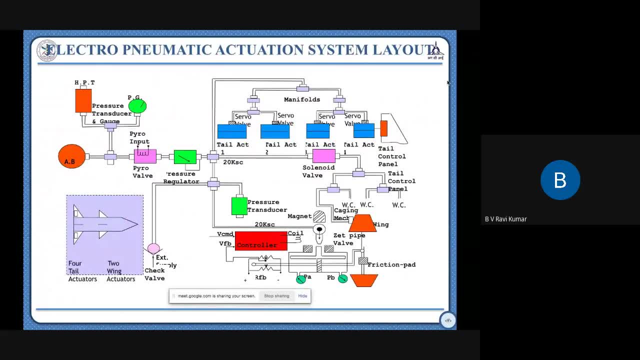 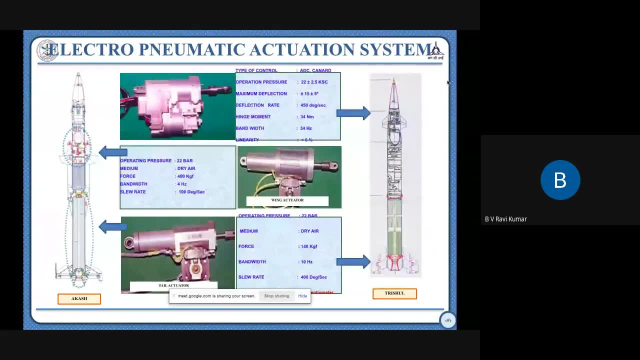 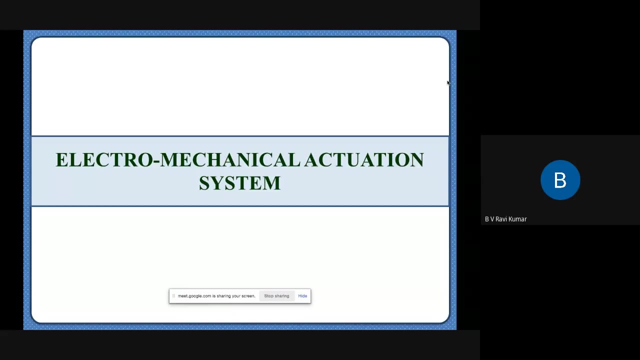 So this is also similar configuration of hydraulics. only use pneumatics instead of hydraulics. So these are the some of the Akash missile where we're using this action system: pneumatics. So this will come to the electromechanical, but they're actually will concentrate more. 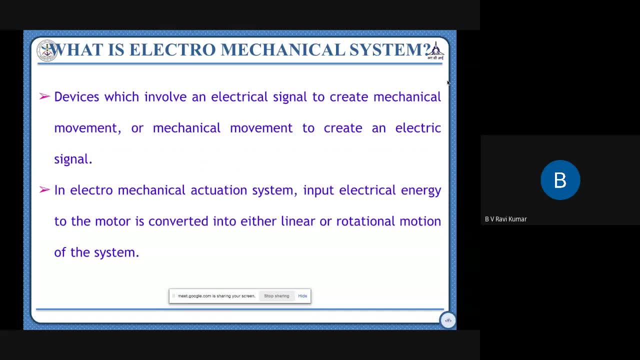 So, basically, any device you can use which will convert electrical signal to create a mechanical moment for this action system that we will call it as a prime mover. So we can use a breathless DC motor. Okay, We can use a breathless DC motor. we can use an induction motor, any motor. 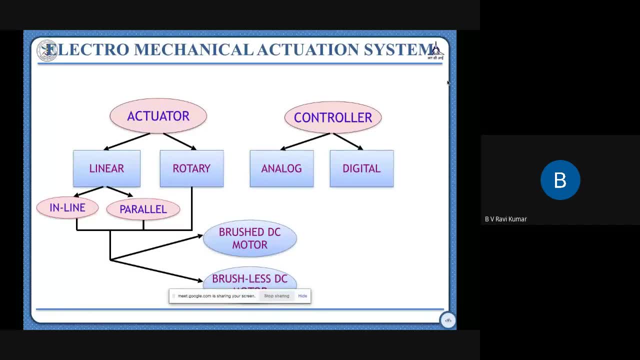 So in this also we have, one is a linear electromechanical actuator, rotary electromechanical actuator and most of the action systems in the missile throughout the world, not only India, not only missile, even space vehicles. wherever we using electromechanical, we go for either. 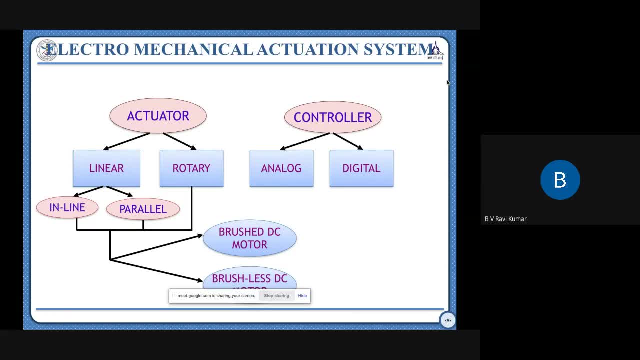 a breathless DC motor or breathless DC motor And now breathless DC motor also. nobody's using. everything is shifted to BLDC motors Only in first generation, small missiles, we are using breathless DC motor, Like NAG and other things, but otherwise all missiles. now we are using BLDC motors. 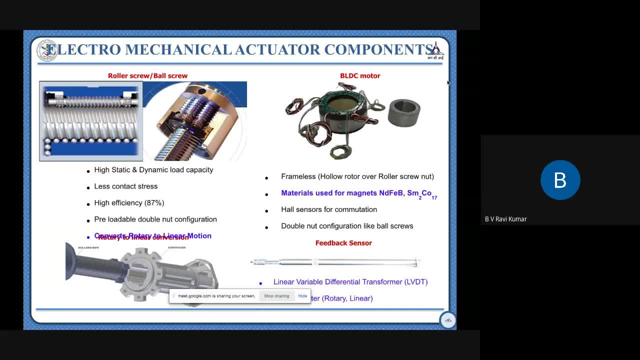 for our electromechanical actuation systems. So now we'll see brief components of what actuation system? electrical actuation system, the major, what I, whatever it will, heart of an actuation system for hydraulics is servo valve, whereas heart of electrical action system is the servo motor. 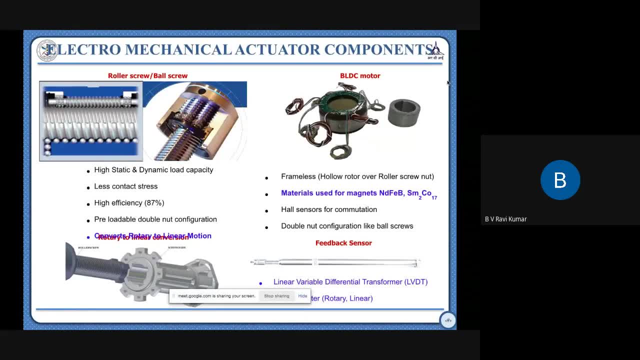 That is a. it can be a BLDC or any motor, but it's a servo motor. So and we have it. screw mechanism. If it is a linear actuator, it requires a screw mechanism. either it can be a ball screw. 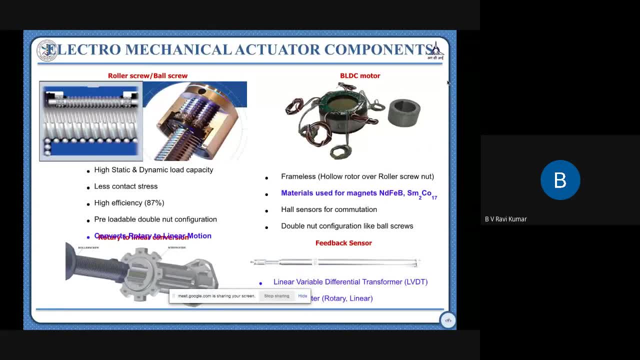 or roller screw, And it requires a feedback sensor which can be an encoder or it can be LVDT. So these are the major elements and out of them, the major and you can say, the heart of the total system where complete bandwidth, complete dynamics, complete load requirements. 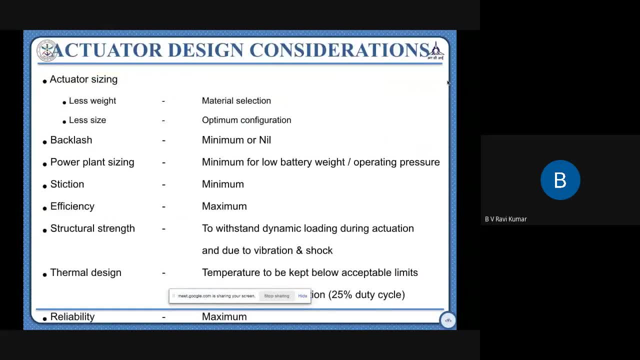 will come from the servo motor And this is, of course, the sizing where we require material selection. What is the configuration And main is the power plant sizing there? actually, that is the area where electromechanical actions system is lagging behind hydraulics. 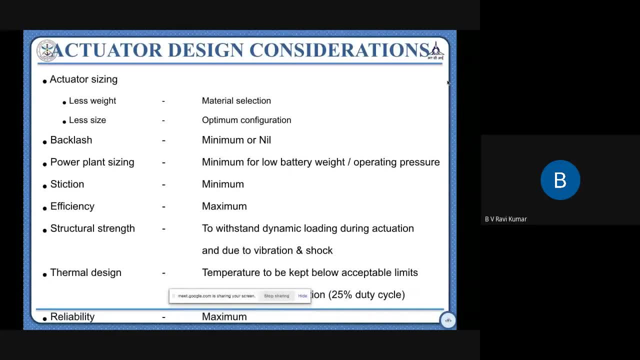 Because the moment you require high power, your battery requirement will be more. So your power plant sizing is very important And there you will design of the machine, design of power electronics and total action system design lies, And I'll just show some of the configurations. 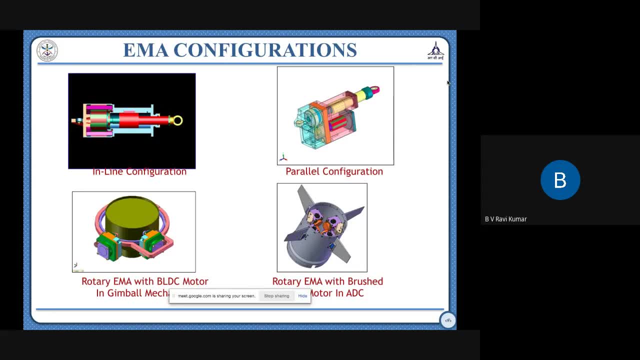 Inline configuration means the motor will be directly coupled to the screw mechanism, Where the motor direction can be controlled, by which the screw will move forward and reverse. And next is a parallel configuration Where you have it A gear drive to reduce the speed and increase the torque so that the motor torque can be. 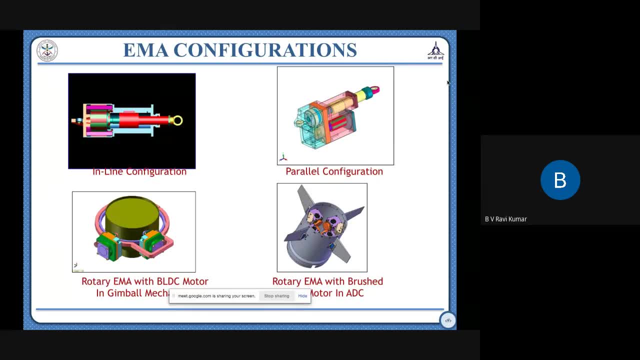 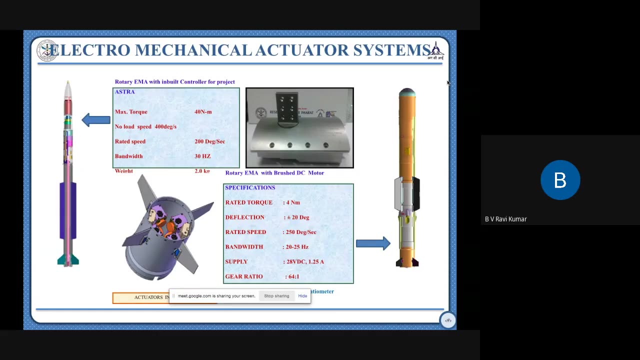 enhanced by the mechanical combination. So there is a parallel configuration and we have a rotary EMA in which there will be no screw mechanism, only motor coupled with gears. So these are different configurations with electromechanical action systems. Now these are the different action systems which are developed for some of the missiles. 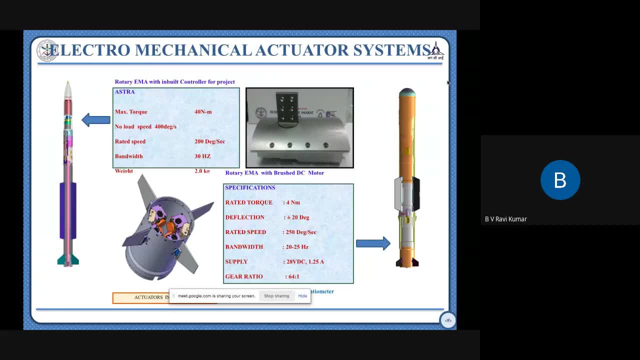 Like we have Astra missile, which is an air to air missile, We have a different action system having different power requirements. The reason behind showing this slide is we have a different action system requirements for different missiles. It's not one action system. cannot go in all missiles. 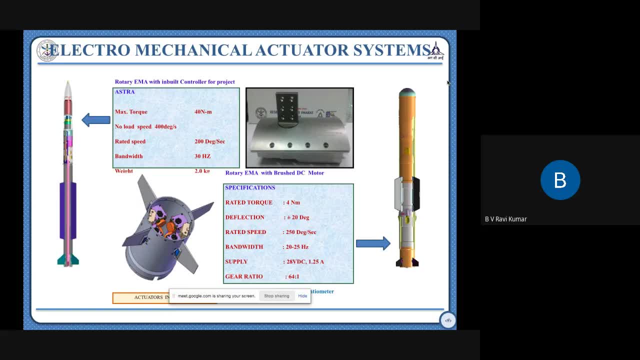 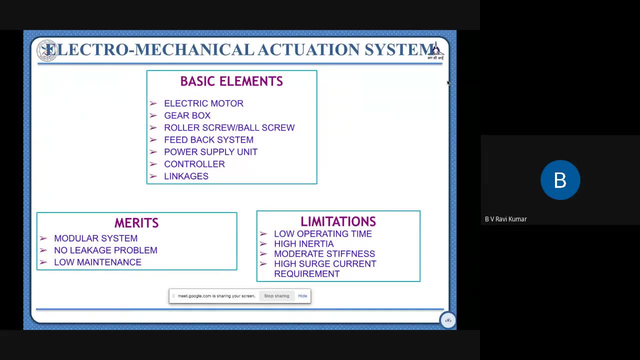 Based on the space requirement, bandwidth requirement and force requirement, the action system design will vary. So now coming to the basic designs and what are the design criteria we have to do. So that is the electric motor. as I already told you, it is the main thing. 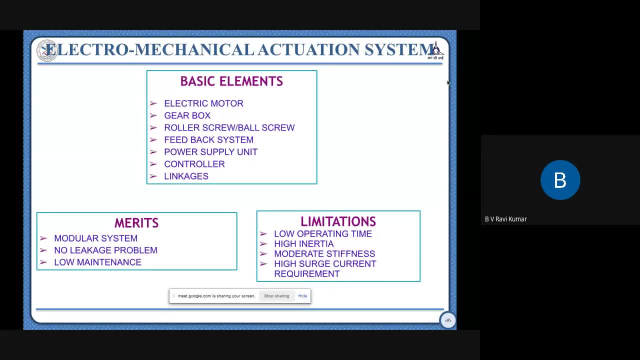 Next we have gearbox roller screw mechanism. which mechanical elements, The power supply unit and major one, is the controller, where complete control algorithm, whether it's a current controller, voltage control, the control system, compensators, everything has to be taken care in the controller. 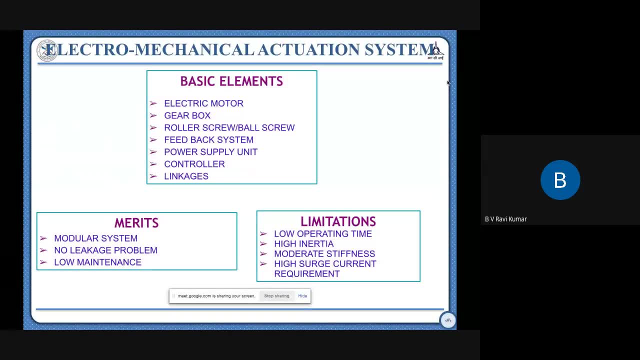 So these are the major systems for, and basic elements for, servo motors. then we'll see what are the merits. It is a modular system, no leakages. it's like an electric vehicle. you can compare this with an electric vehicle where you're driving with only motor. 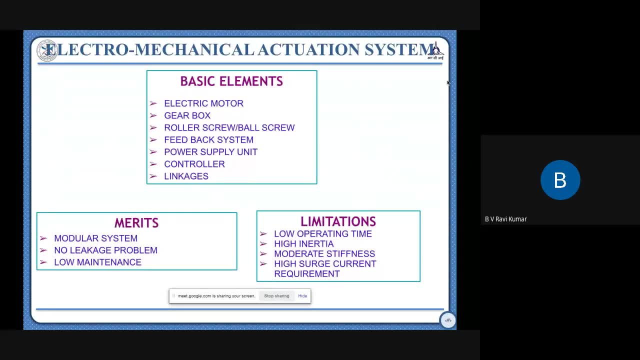 So definitely, compared to hydraulics, it's always better because you don't have much subsystems. It's very modular system, no leakage, very low maintenance. So that's it Coming to the limitations. So this is the area where we have to work more, because the industry is moving towards. 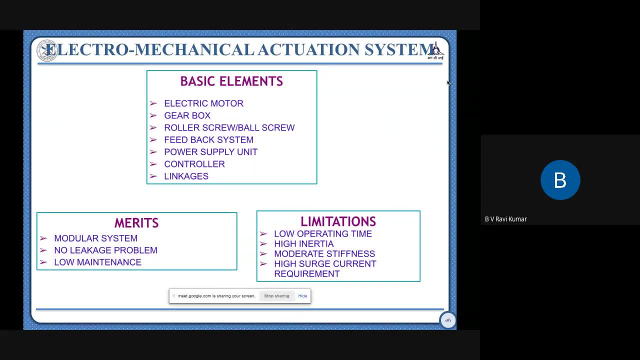 all electric aircraft and even electric propulsion is one of the area, and missiles also we are working on. So what are the limitations? low operating time, high inertia and moderate stiffness and high surge. current requirement. These are the main things. that is, a low operating times comes from the battery or low operating. 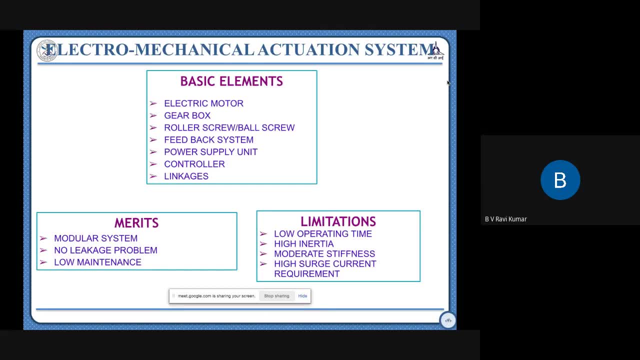 time, because of the temperature of the motor and also the power electronics. So these are the areas which we have to work on to make it more usable for all applications, including aircrafts. So this is the basic block diagram how the control is done. 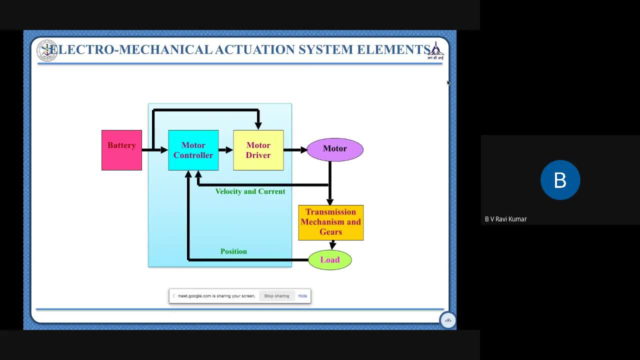 We have a motor controller, motor driver transition mechanism and from which we are getting a position as a feedback, and velocity current can also be used as a feedback based on the application. This is a complete block diagram of actuation system, Now in depth, if you go a little bit in depth. 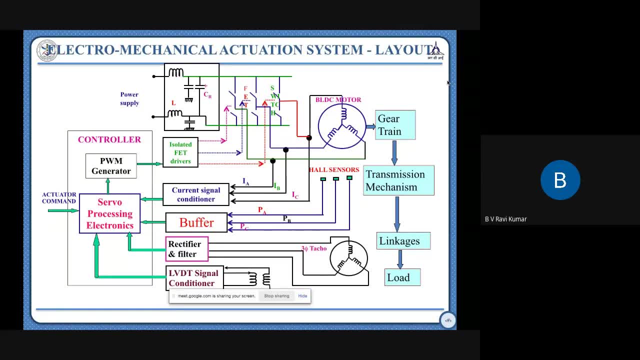 We have a power invert, Basically slides. we'll be talking about the bridge bl dc motor, so the power inverter, what i'm talking will be for a bl dc motor only. so definitely i will come to the what are the next level challenges and next level developments, which is which may, may, i'll stress on that, but whatever. 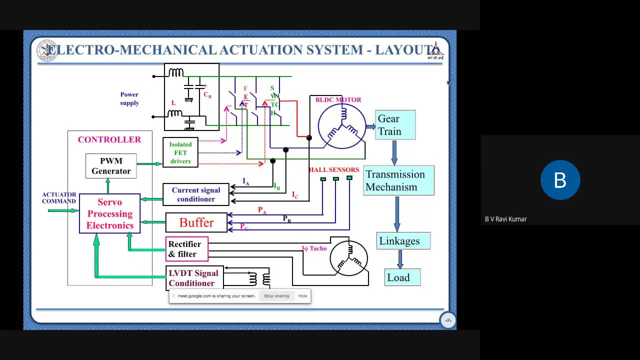 slides i'm showing now. we'll generally speak about bl dc. so this power inverter is a hexbridge inverter where you will have six, six MOSFETs to control the bl dc motor. it can be a triple shuttle commutation or a sinusoidal commutation, based on the application. so this is the hexbridge. 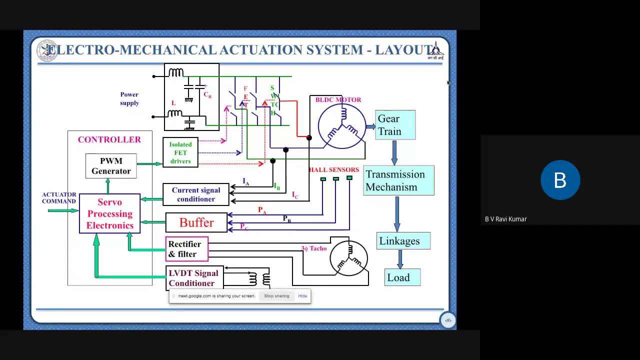 and we have a emimc requirement. that is one of the major requirements for any aerospace application, because all the power source will not be common to the actuator alone. the power source will be shared among different subsystems, so that emimc design, which is a critical design, 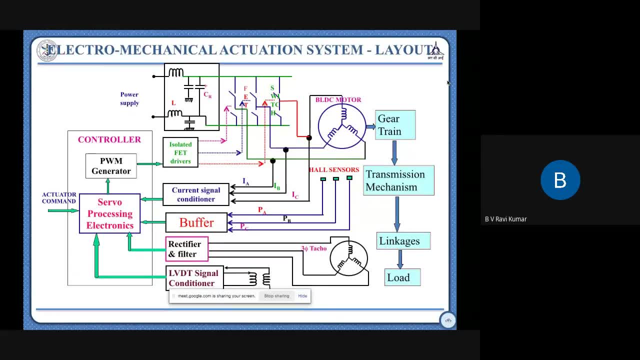 is very much important for any actuation controller. so that's what i'm showing in a block here which is nothing but emimc filter through which it will go and finally go to inverter. from there we have a bl dc motor and we have hall sensors for the sensing if it is a trapezoidal. 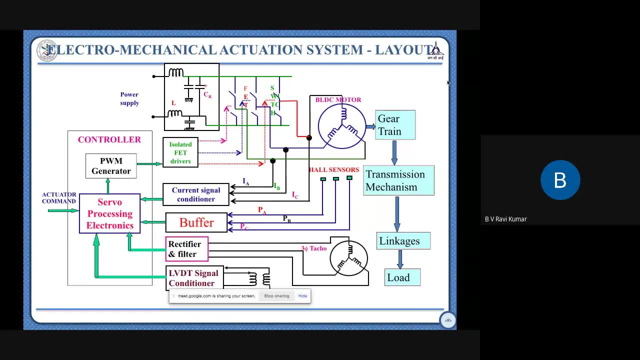 control encoder for some of applications where we're using the sinusoidal controls and we have a separate controller based on our communication interface, which is the obc onboard computer. we have different communication protocols. as per military standard, that communication protocol has to be included and, finally, complete control will be done by the controller which 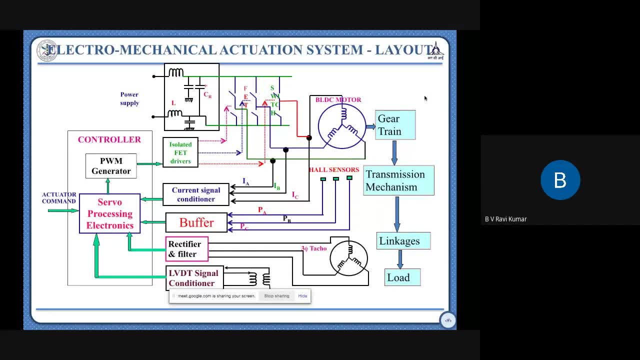 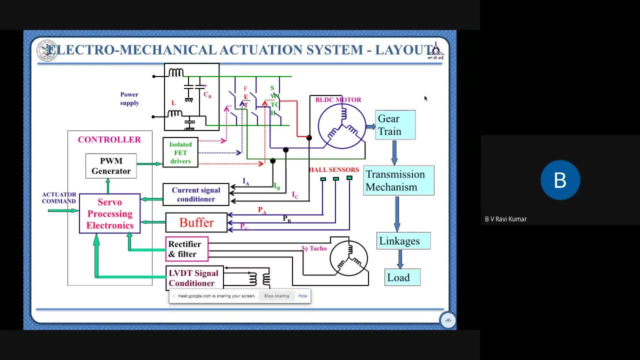 a power amplifier and we have a power amplifier section and a signal conditioning system. we have processor stage, signal stage and power stage to combine it will become a controller and finally it will be connected to the motor to control it in a closed loop. now what is the advantages? i think we don't need to go much on this. we already know these are the. 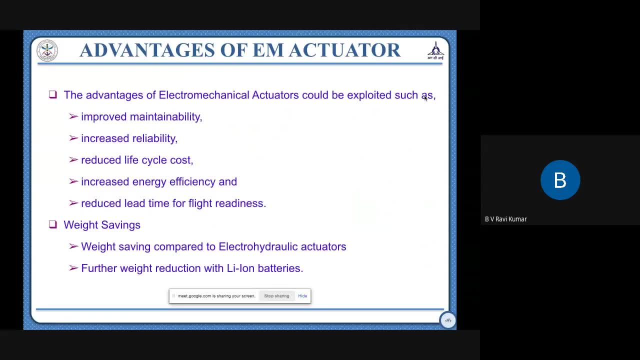 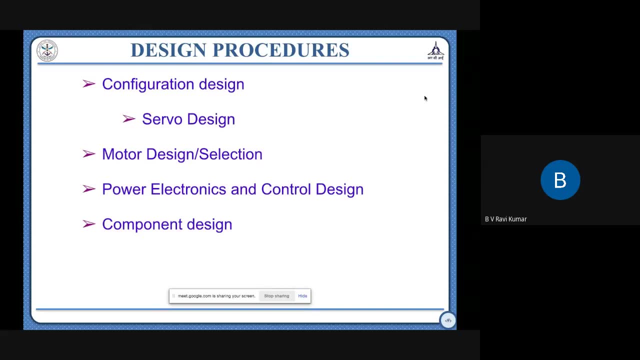 major advantages of electro mechanical because of no reliability, maintainability, so high reliability for all aerospace vehicles and all missiles. now it is completely going into the electromechanical actuators. only even the space vehicle is what is what is doing. also, they want to go for electro mechanical of very high power. so, but there are some limitations. 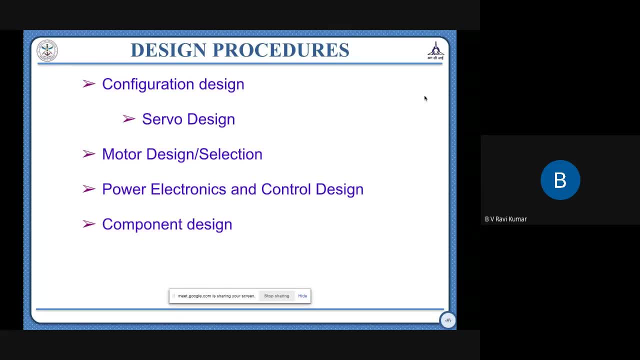 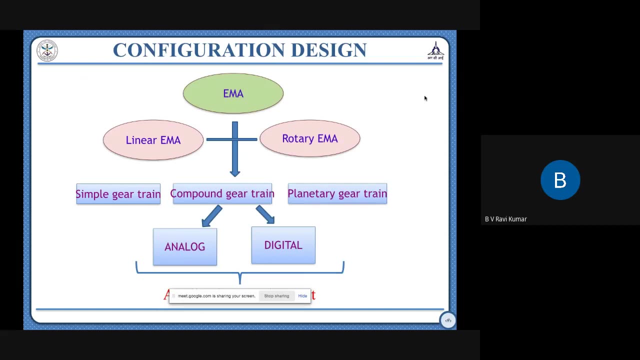 which i will be covering next slides. so coming to the configuration: design: servo design, motor design and selection, power, electronics and control design. so these are the major things. so coming to the ema, this already explained. we have different ems- linear rotary- and we have also controllers which are digital, analog and analog. nobody is using it's completely. 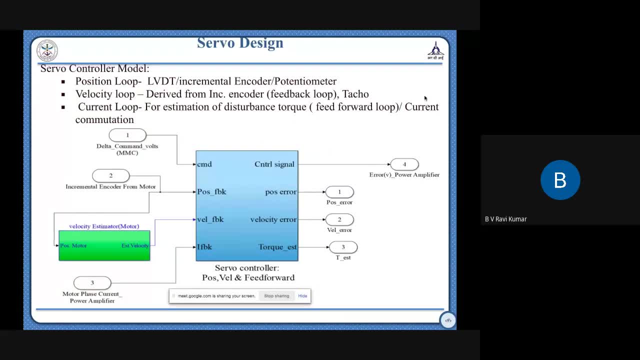 digital platform now. so, coming to the servo design, this will be something interesting to you because this is the area which has to be more concentrated for all actuation systems, because there are a lot of constraints and requirements coming from the missiles day by day. so position loop, normally lvdt, incremental encoder as a sensor which we use, a optical encoder or magnetic. 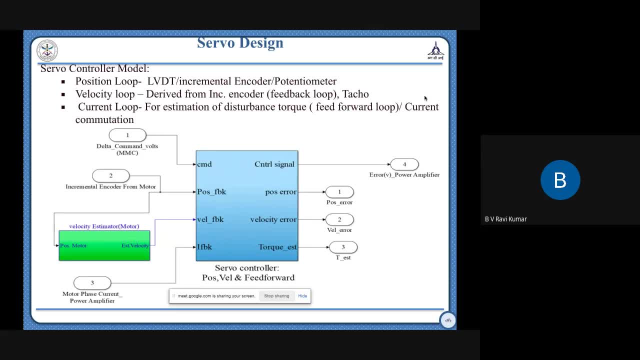 normally we use magnetic encoder because of its reliability and ruggedness. magnetic encoder and potentiometer normally we are avoiding because of its own problems. normally it will be an increment encoder or lvdt, as a position loop and velocity loop. either it can be derived from encoder or we can have a taco if you want to have a higher velocity gains. 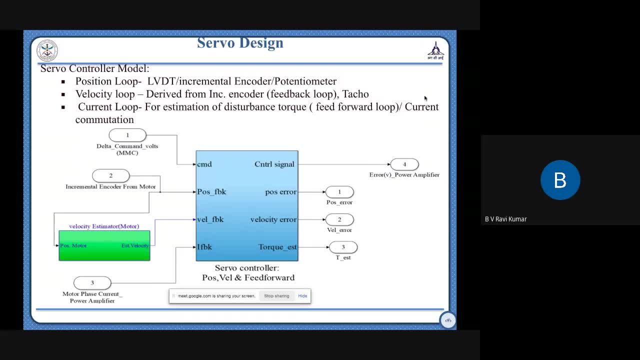 and for current loop for estimation of disturbance start, which we will call it the feed forward loop, and current computation. so we have a very interesting requirement for an for, especially for arrows based vehicles. there will be a lot of uh unset entities even when the vehicle is flying, because a lot of things you cannot estimate unless you. 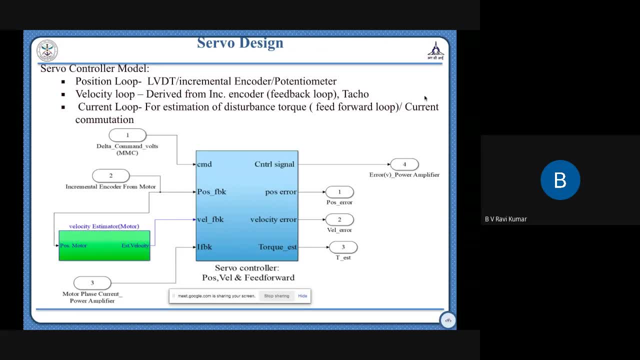 test and you cannot wait for your testing because you test, finally, in the air only. so you have, of course you have some setups where you can simulate the air air conditions on the ground, but still there will be a lot of uncertainties once the flight is fine, so our system should not be we. 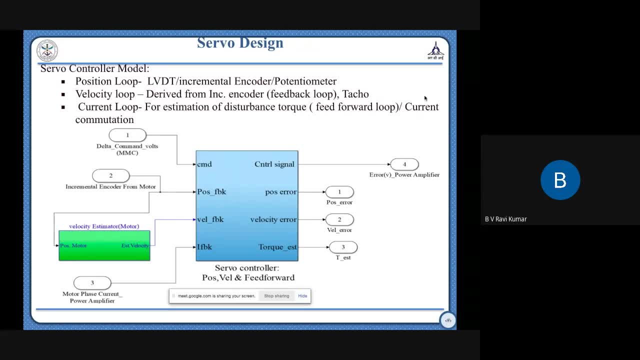 should not learn anything from the flight. we should design everything and we should fly it. we should not afford any failure. so for that, the major things come from the controller design, because we one is the aerodynamic load, one is the major thing is the opposing and aiding loads on the. 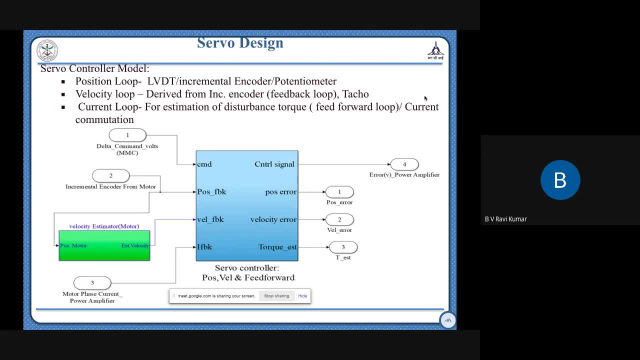 actuation system. so your control loop should be designed such a way that you should not have any difference in the aiding and opposing loads, for which you require a very tight and high bandwidth current loop. so it should require, in the terms of 10 kilohertz current loop you should have. 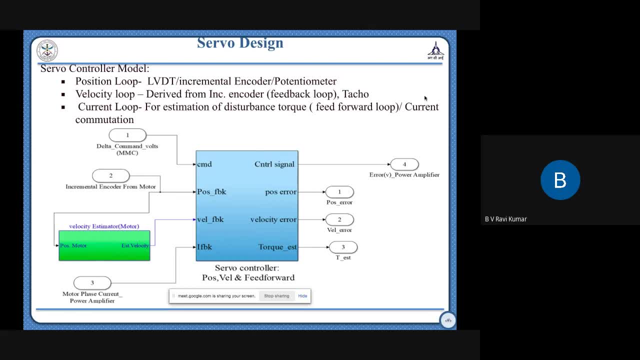 to control your actuation system perfectly in aiding load as well as an opposing loads, which is a hundred percent aiding and 100 opposing loads. so that means what will happen if you don't able to control it. what will happen is if you know supposing aiding load, if you're not able to, 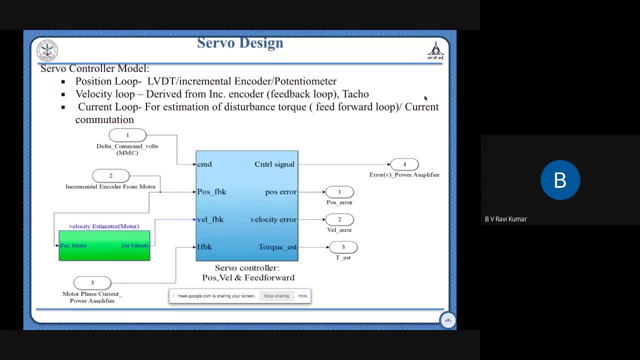 control it, you will have a huge overshoots which will eat away your margins, control system margins- because of which your vehicle may become unstable. so these are the areas which is very much required for any servo design. so you should have a very good current loop, velocity loop for having high 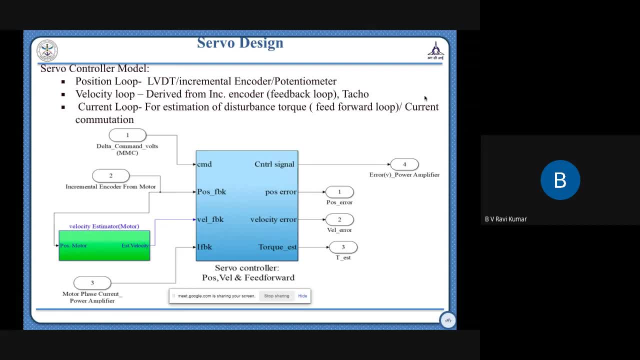 damping and of course position loop, because total system itself is a position control system. they require a position look as an outer loop. so this is how the servo design starts. so here the main element is the plant, because you have to design a motor first of all to able to control in this way, because if you're 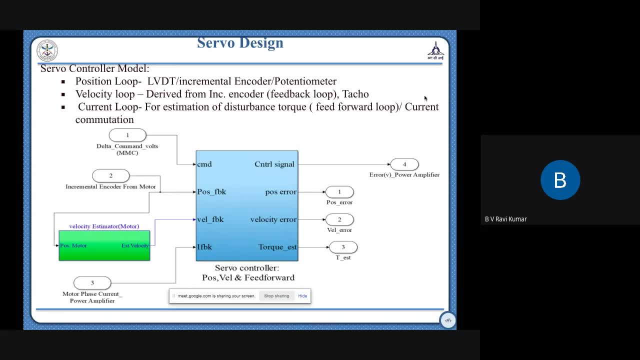 designing a motor with a very high inductance. probably your aiding load you will not be able to control because of high inductance. you cannot control in the aiding load and of course you will have a lot of speed drop in the machine. so these are the design parameters we have to take in the 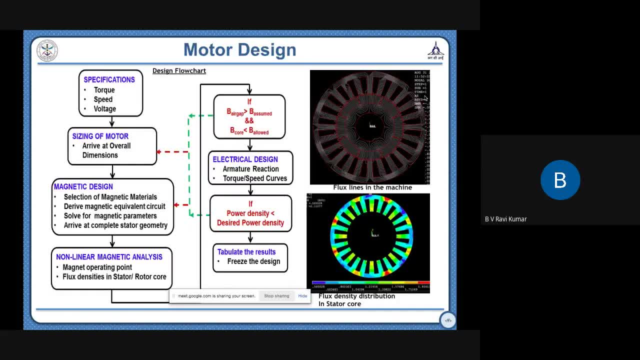 right from the beginning of the design. so i'm coming to the motor design. just one slide i'll show you about the motor design and criticalities of any drive design. not only motor, it's a motor plus power electronics, because the major thing is in any machine, the whatever. you can ask me one question: why little? lot of companies, of course. 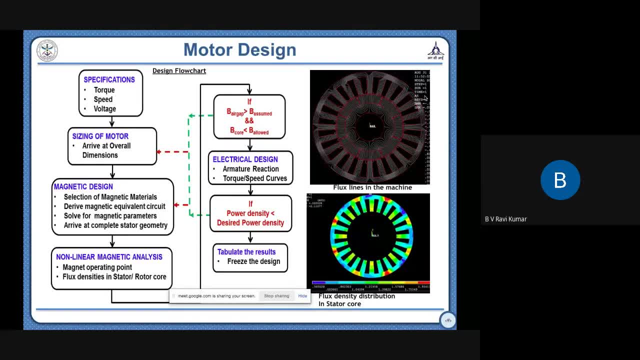 in india. unfortunately we don't have any company who design a servo motors. we have a lot of uh students presenting a lot of machine designs but unfortunately everything we have to buy from outside. only like you name any company like uh uh, fallahobar or kilo and some of the companies. 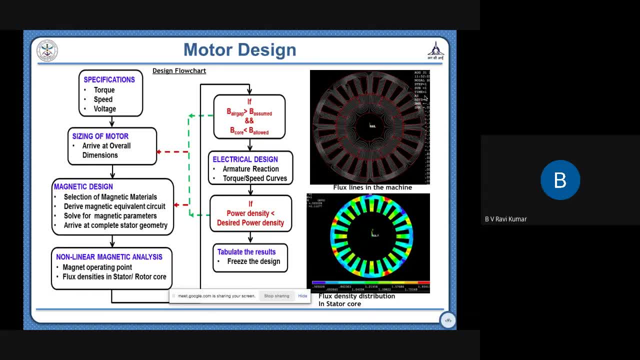 which we call it a sermat. all these things are very famous motor designers and we are buying it them for some of them, but definitely off-the-shelf motors will not give our requirements. because a motor designer and control design and power electron design should be same as far as i am concerned, because 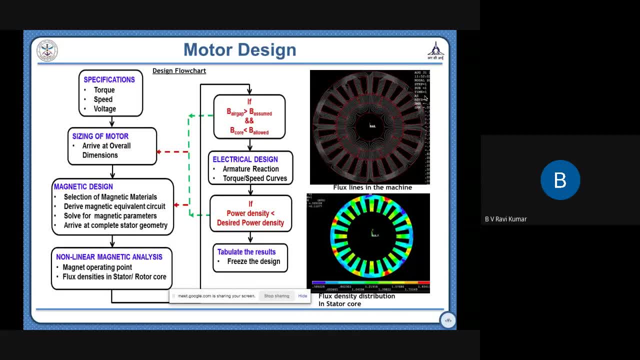 motor alone. if you design, you don't know what is the current control it is doing. you don't know what are the harmonics are injected in the motor. you don't know what is the period of frequency it is operating, the motor design is incomplete. if you're designing a power electronics drive without knowing, 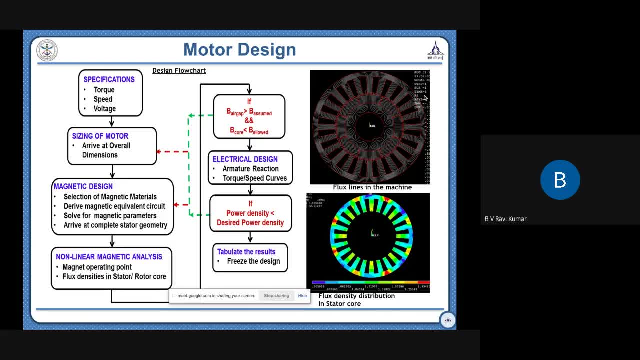 what is the motor actually doing? what are the type of transient it is happening, what is the type of? what are auto? then we have to design our polo tronics according to that motor, which in some applications may work. in some applications it will not work. so what i am trying to do is to actually use the приготов. 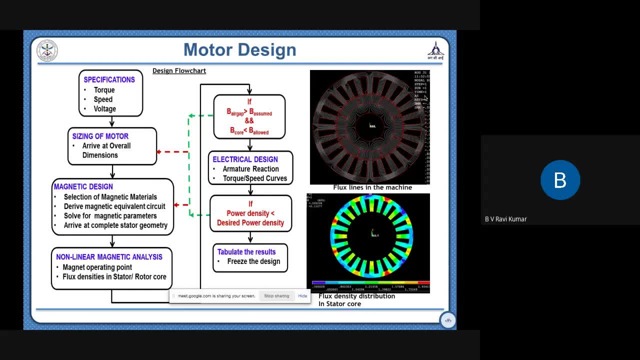 so what i want to say in this slide is: this is the motor design which normally followed. we cover place. we design all the motors, uh, in-house, for our all missile applications as well as space applications. like we start from the torque, speed and voltage, we'll arrive at the motor. 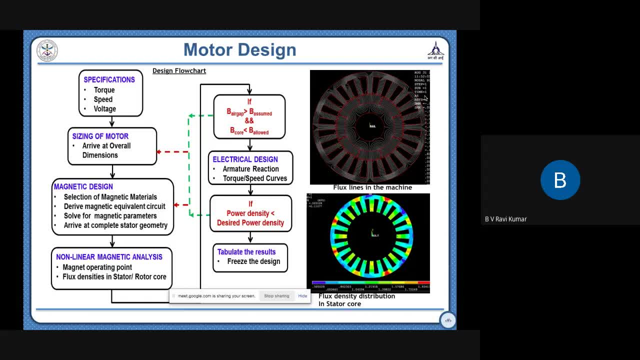 design parameters, the magnetic design, where there are a lot of materials, selection of magnetic materials right from it. bh characteristics, its magnetic properties. it's very much to start from the beginning because any outside motor you are buying, normally they rely on the commercial applications. they will use a non normal commercial material because the cost is important for outside. 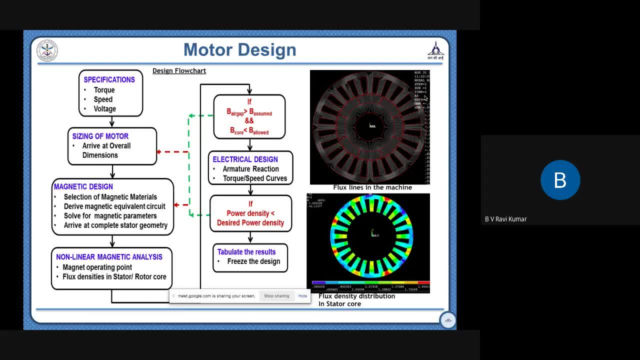 industry, but ferreras aerospace also. cost is important, but some of applications the performance is more important than cost, so that also we are coming like we should have more performance as well as low cost. there is one more subject also i'll just cover, so selection of magnetic materials. 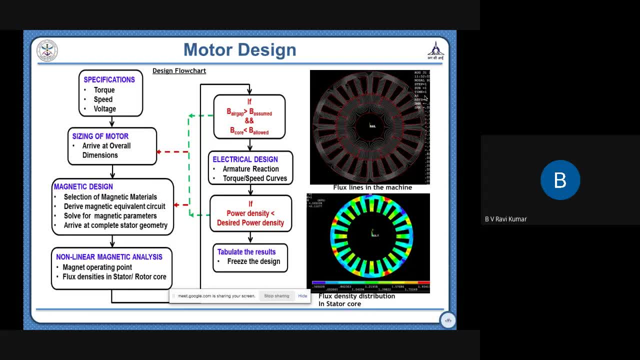 derivation of the magnetic equivalent circuit, and all these things are the standard design processor for any motor. and next comes electrical design and finally you, based on your optimized parameter to design. so this design should include your control system requirements. so you cannot design motor separately. it has to come from the control system requirements of our application. next comes the control design. 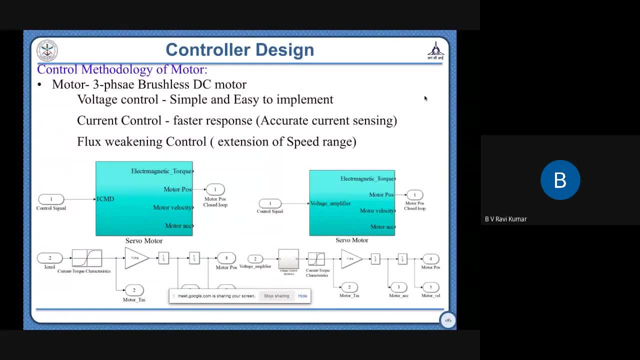 now comes to the control methodology. probably this very much you will be learning in your power: electronics and tech. you will have a lot of flexibility, control, all those things, but they are very much required for the industry. i will tell you now, since electric vehicles are into the 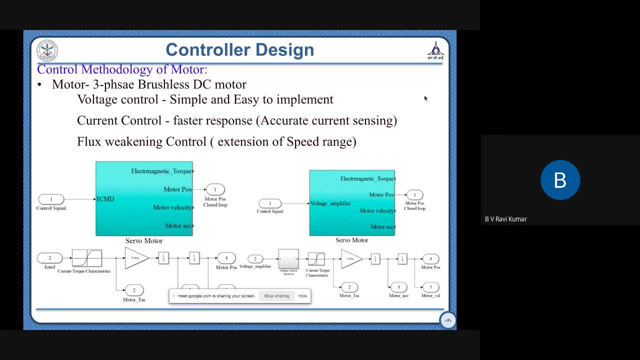 market. we have a lot of ics which are having all controls in the singularity, like texas instruments. they are having ices where they have their own algorithms which we call, i think, imotion, or something which we are giving everything, but actually industry, if you take it's like it's. 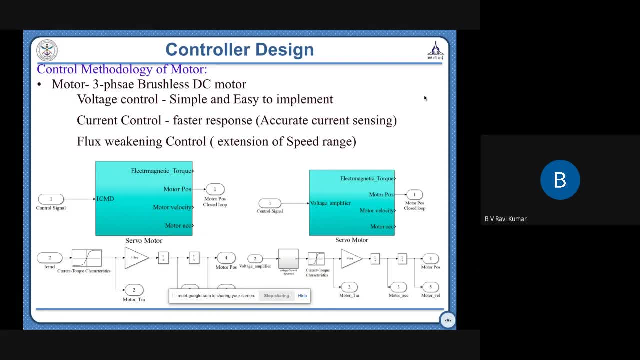 not very much required for some of the applications, like blz motor. frankly speaking, foc is not required because, as such, blz itself is designed with a qd axis with 90 degrees to each other. so but the industry is projecting some of the ices in such a way that can be used everywhere, but it's not. 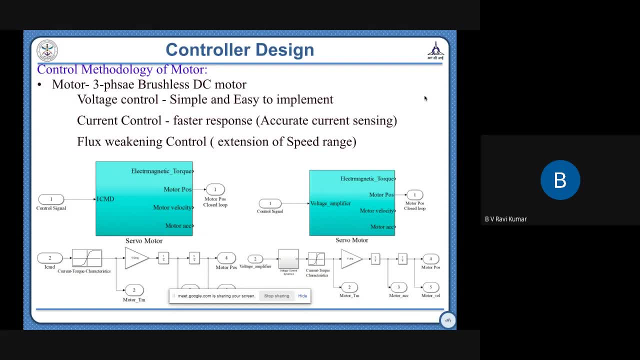 so it depends upon the application. if you're doing for a voltage control, it's simple and easy to implement. so some of the applications where we don't require aiding load and opposing load, then again just simply we have to go for voltage control because it's very simple and there 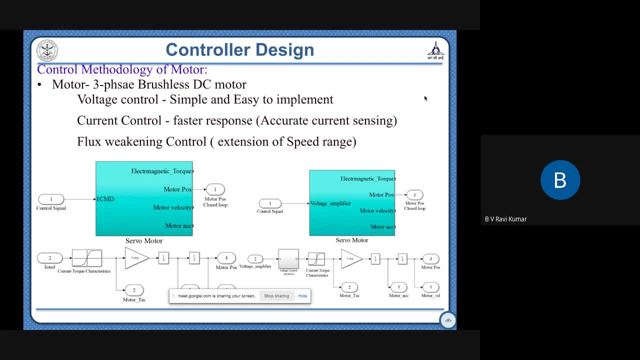 industry, ics, all those things projecting. they have their input- current sensors- but definitely they will not work. i mean, they will not work to that level of sensing. so that depends. so we have to make our own custom requirement based on our requirement, based on our type of currents. 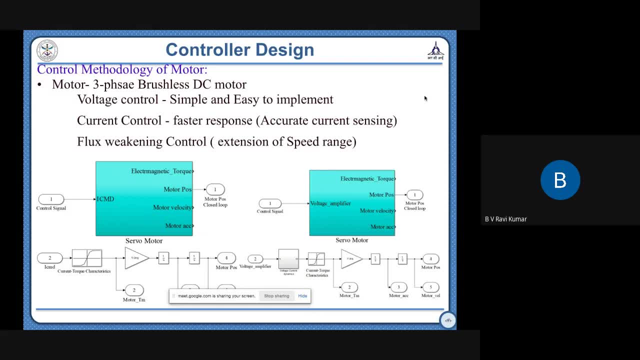 handling, we should be able to design our own control. and coming to flux control, these are flux weakening. this is very much important in terms of the machine as well as the control, because from the motor point of view, all battery voltages we can reduce if you can improve a flux. 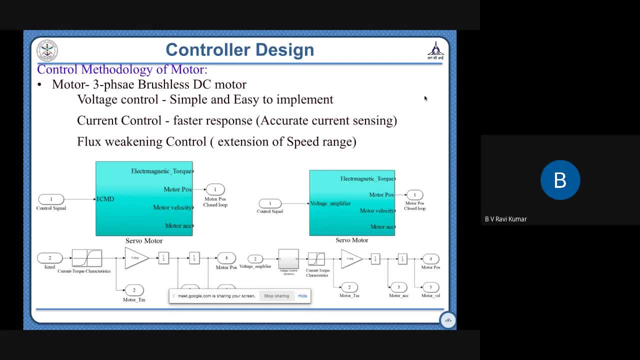 weakening control. that's what we are doing for the space vehicles. we're employing the flux weakening control so that the battery voltage- we can only to go for high voltages, normally the velocity requirement in a missile or an aerospace will come. will come whenever there is a demand from the system, so the demand will not be continuous. so for that we no need to carry a. 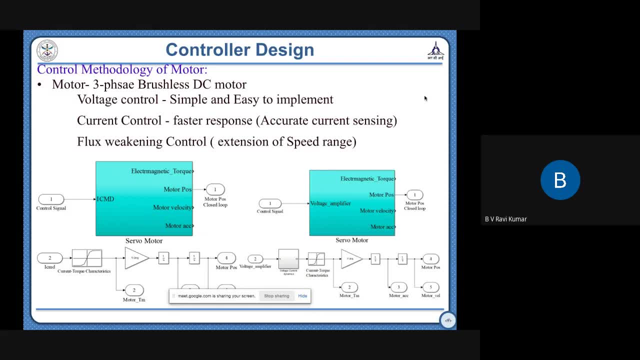 high voltage battery. so that's where we can overcome the hydraulic actuation systems, where even for high power wattage also, we can use blc motors and actuation system, electrical action system by employing flux weakening control, which already is being done. so the main criticality, flux weakening control, is well established in. 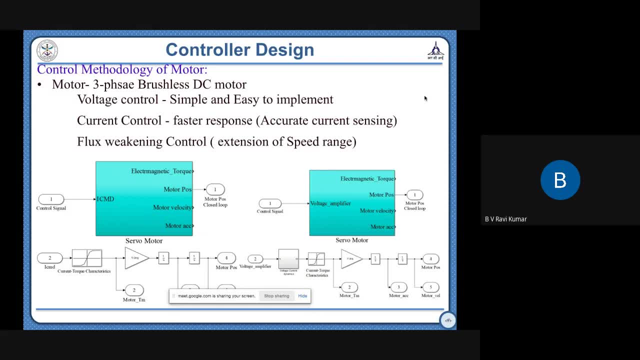 terms of controller. there is nothing new in that, but only from the motor point of view. the main difference for the motor, the capability of the motor, should be for flux weakening. that means we should be able to give the torque as well as the speed extension, that from the motor design, the 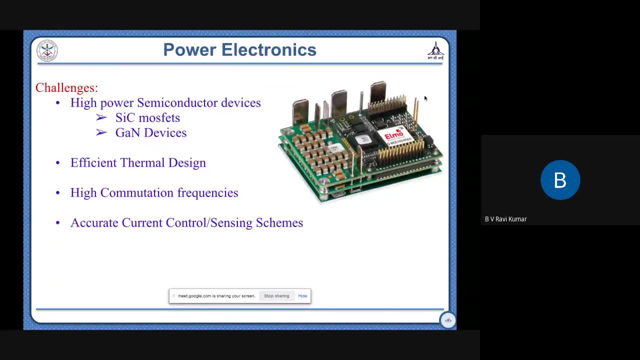 main criticality lies. so, coming to the power electronics, it's a very much important area. normally, in fact, we have a lot of power electronics experts in the in academia and industry in india, but unfortunately we are buying a lot of power electronics drive from outside. so there is a famous company called elmo which i am talking to. 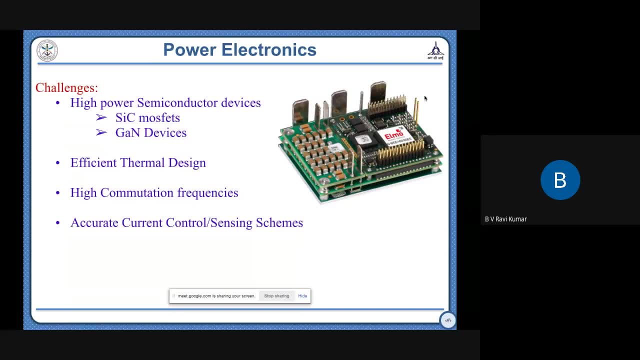 every industry in india to make it, because this is a elmo motion control drive which is from israel, which is we can say it's the best. it's an excellent motion control system which everything is lies in one asset. so they developed their own asset with all sorts of control. it's a very good. 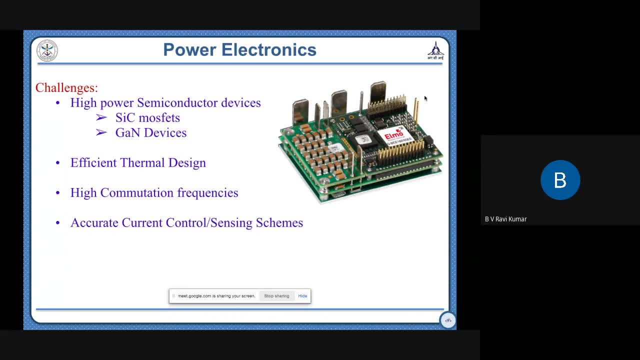 device giving an excellent performance that's being used in a lot of new generation missiles, but i want to make this in india happen, because we have a lot of experts from. we have a lot of students, youngsters like you, who can use this. very simple techniques are available. 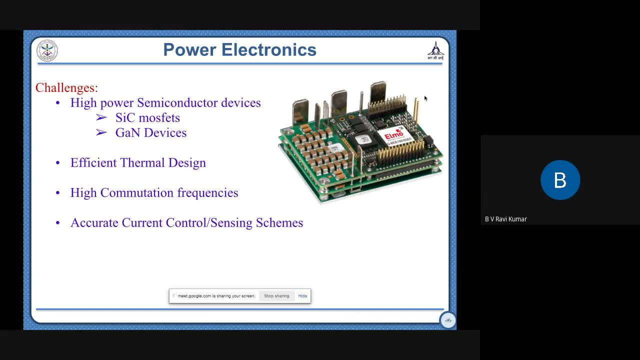 which we are already studying. same thing we have to apply to our application and make our own controllers, which will come from india. so in this main thing is what we can go further is we can go for sac mosfets, which already industry is doing. there is no doubt ssc people are using for all. 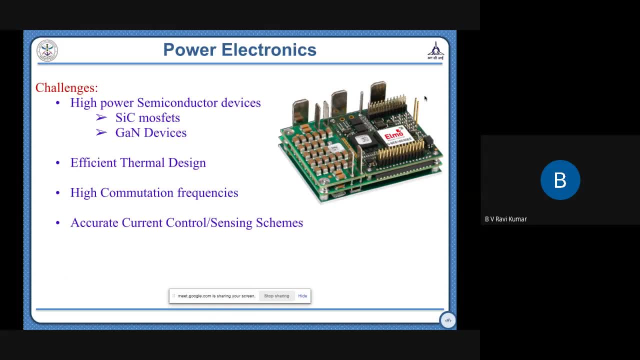 high power applications and we can go for a candy versus if you are going for very high frequencies. probably that may not be required for power electronics for drives, so that will be one of the features of the ssc. the other thing is that we have a very efficient thermal design which is 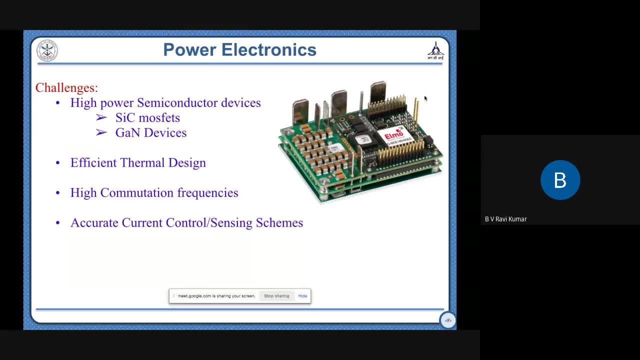 very well known in india- and efficient thermal design, especially for actuation systems. that is very much important because we have a huge currents, because actuator has to move in a very high frequency- 30 heads, 40 heads bandwidth we have to move, so always the action system will be of that. 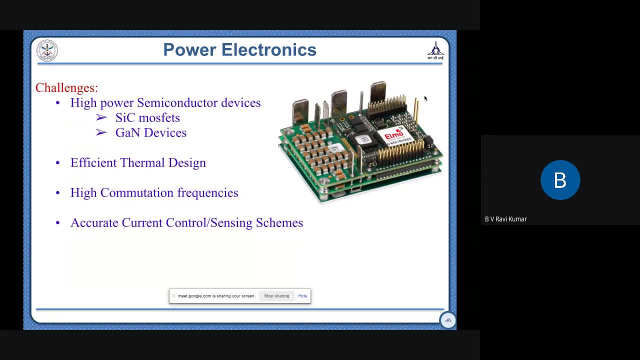 range the current requirements in that small space, because we want to. we want to reduce the weight, so obviously thermal design should be very efficient and of course high commutation frequencies, because itself we are going up to 30 000 rpm. so once we are going for a very high speeds, the accommodation 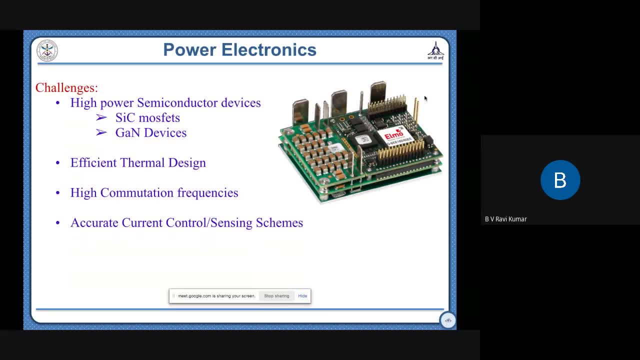 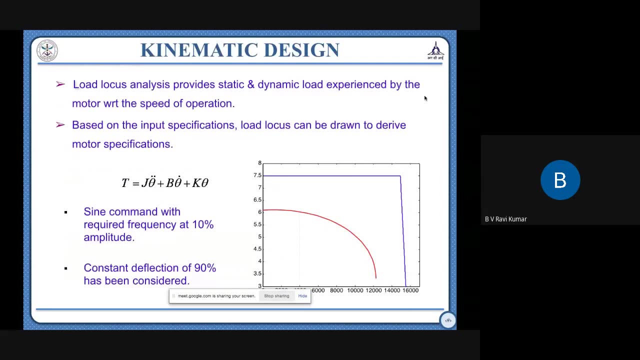 frequency should be very high and your losses should be minimized. so this is one of the area, from power, electronics and devices point of view, very much is required. so this, of course, kinematic design of an action, this slide i want to show you, because the torque depends on the motor, it depends upon the inertia. it's a very famous equation, but here only the. 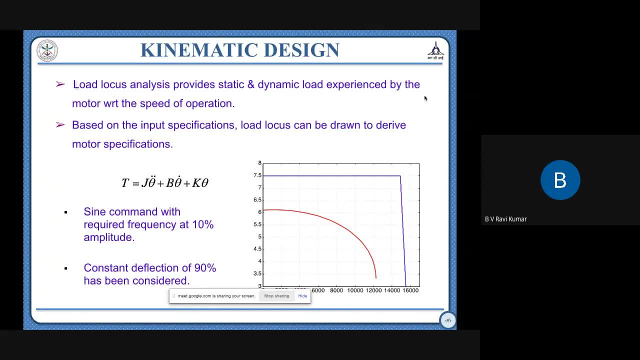 uncertainty comes from the inertia, because there will be a inertial variation once the vehicle is moving. and also the load torque. i have not mentioned here that low torque is uncertain. it can have an aiding or an opposing. so this, based on this equation, the total sizing of the motor. 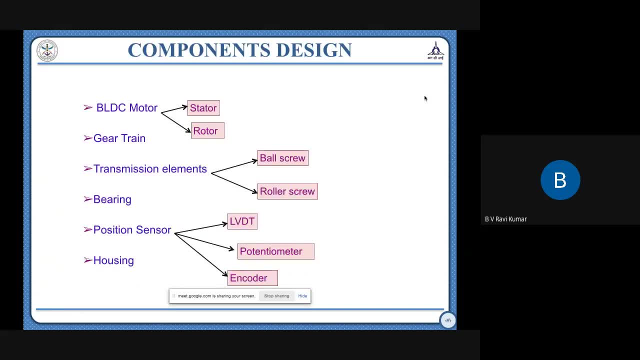 will be done. this is, of course, same thing. so now we'll come to the. i'll just skip this. it's a again a component design where most of the mechanical things are there. and coming to the blc motor, it's only the stator and rotor, which already covered. this is about the transmission mechanism. 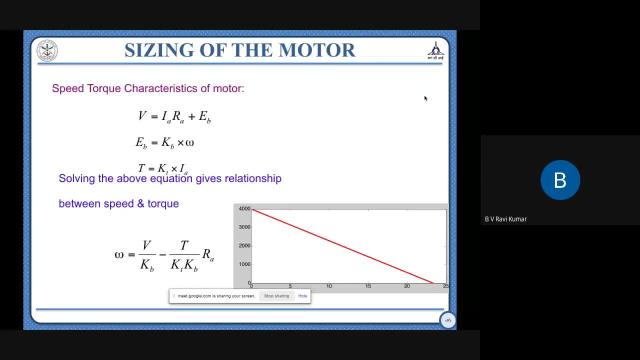 this is again the gate trends which we can just go through it. yes, this is one important slide. i want to show all of you which very simple basic equation, what we have studied in btex, but this equation never actually follows the actual result. so it's a very important thing which normally any industry motor drive designer. 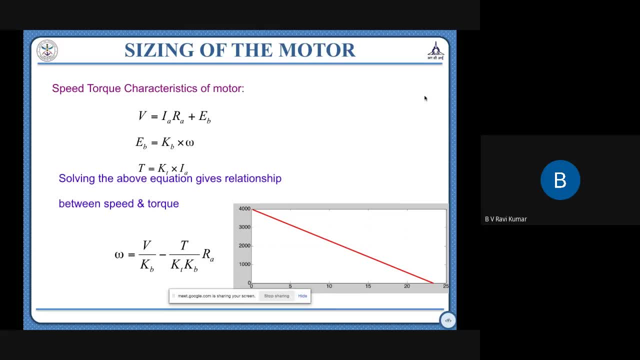 will not give any information of its speed torque characteristics. he will just give speed torque characteristics based on this equation, which is not at all true when you actually design a motor. so there are a lot of parameters. the major parameters are the giving, the, the, the, the, the. 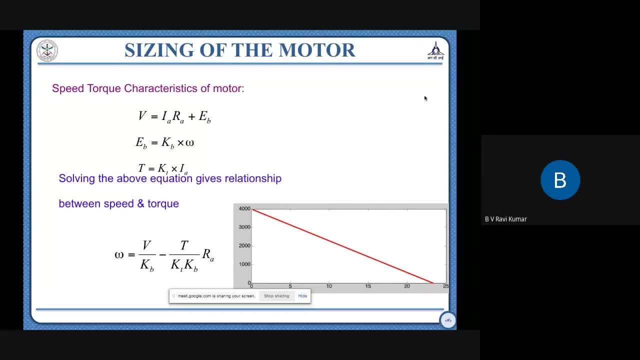 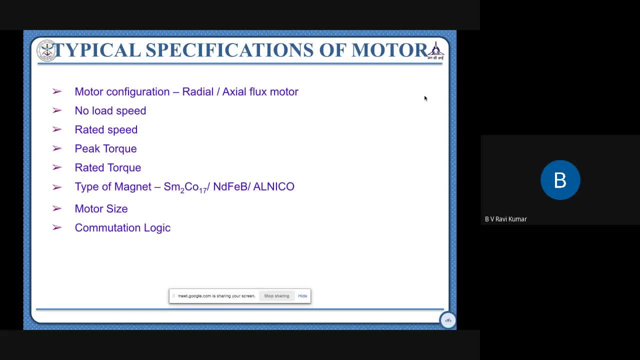 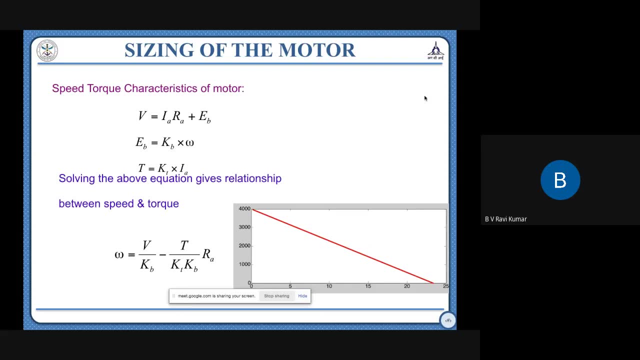 data sheet, and this all will affect your control system design. so the major thing of showing this slide is this: as a motor, i can give this, but ultimately this will affect your control system design, in which you will have a lot of overshoots because your speed is not that desired speed. 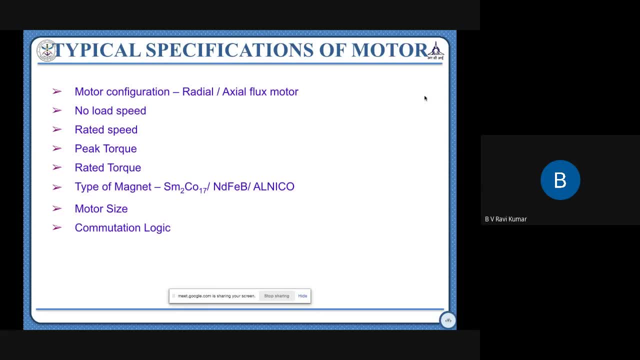 as the load is increasing, you are operating at a very lower speed, so you're not able to meet the required specifications. so you'll increase. you'll simply keep the increasing gain, because of which you'll ultimately result in increasing the overshoot. so these are the very much important. 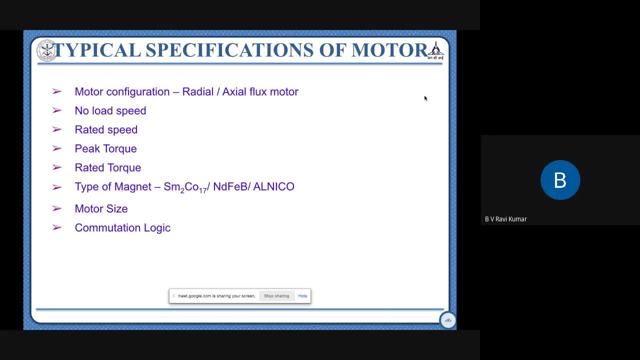 parameters which as a designer, as a machine design or as from the power electronics then you can use, go for a flux weakening, in that cases to increase your base speed of course, then your actual power requirement may come down. it depends again on the motor design. so these are the important. 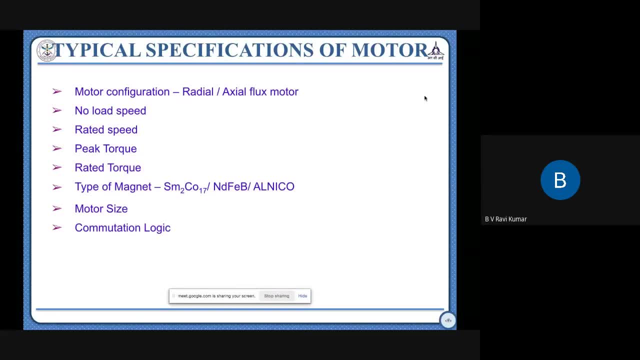 parameters. we have to look into it during the design or during the selection. and if you tomorrow, if you go for a control system designer for any company also should be able to understand the servo motor. if not designed, the parameters of the servo motor should be able to model it. then you have to use for the applications. next, coming briefly about, 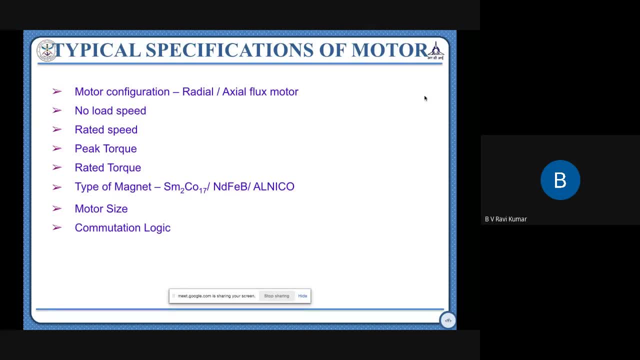 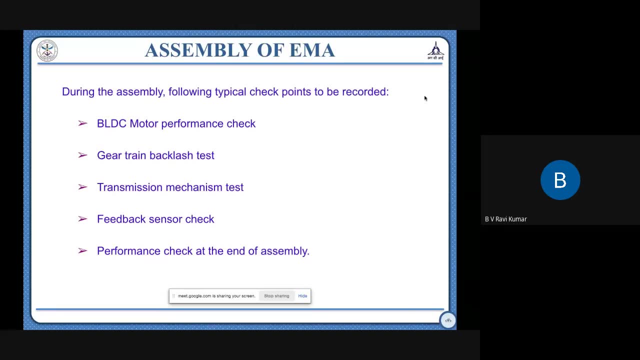 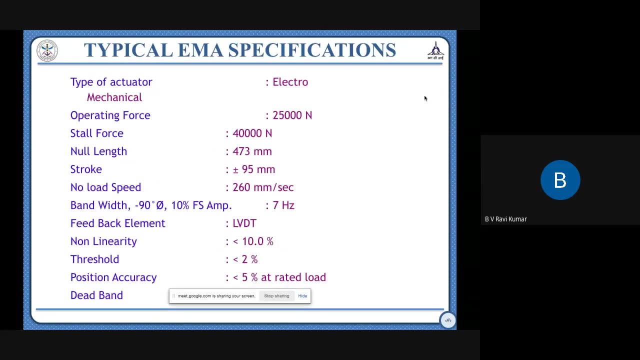 the motor. i'll just show my major parameters. these are the major configuration, speed, all those things, and this of course it's a general thing we have to during the assembly check. then these are some of the specifications. just i want to show you what the type of forces normally we work. 25 000 newtons, that means 2500 kg force. these are the actuation. 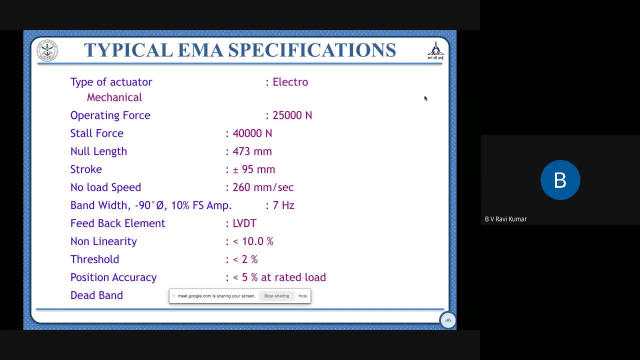 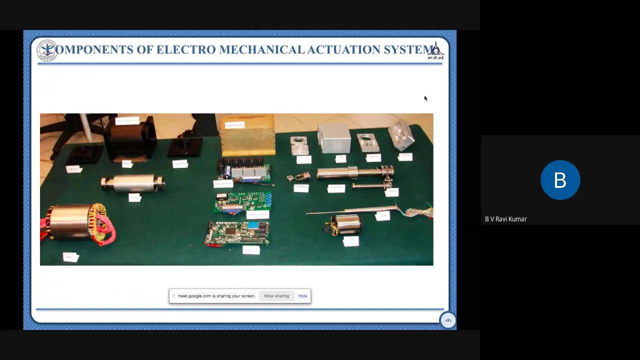 systems we are using, and this will go to something like 25 000 kg force. if you're going for a space vehicles, so it actually has to give this much high forces, so your design should be so, uh, robust enough to take this type of loads. so these are different components. just to get a feel, this is. 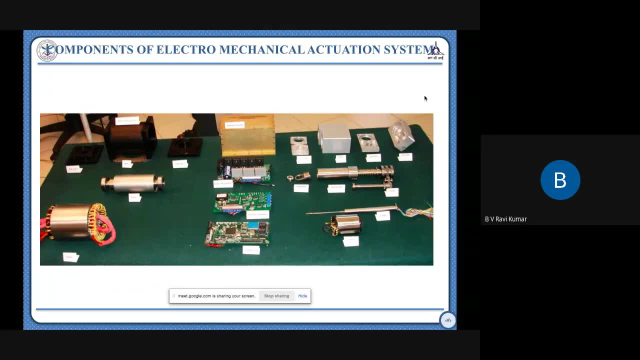 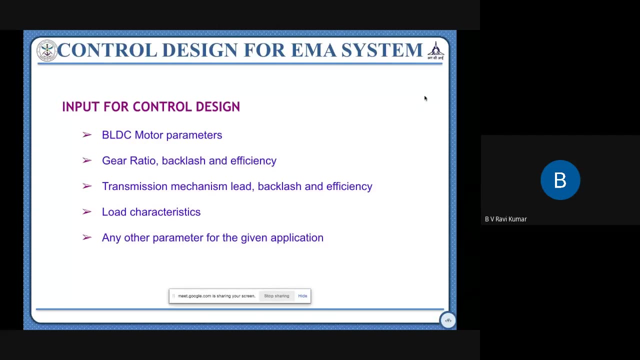 the stator and rotor which will, which are all being used in missiles. these are the kit of parts type of thing which are developed separately in our local industries and we are import and we are using in the missiles. this is about the control system design. major thing comes from the bl dc motor and its parameters. 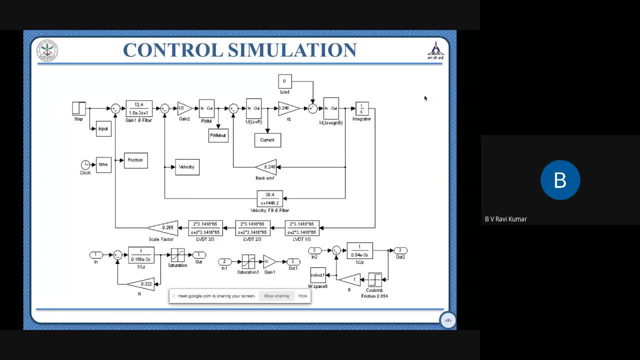 this is uh. here also actually we have a three-phase machine model including all sorts of inductance effects and all sorts of- uh, ig, i mean device effects. we have a model but that i could not bring to you. it's a single phase model. here actually, bl dc motor is model model equivalent. 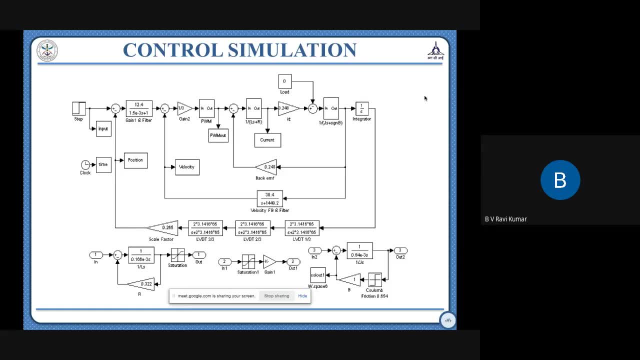 to a dc motor. this is absolutely not correct. we should have a three-phase model, because the three-phase model will only give you exact picture when you are operating at higher speeds, because the mode machine is switching from one phase to other phase while it is running, so each time the inductance of each phase will have its own effect. 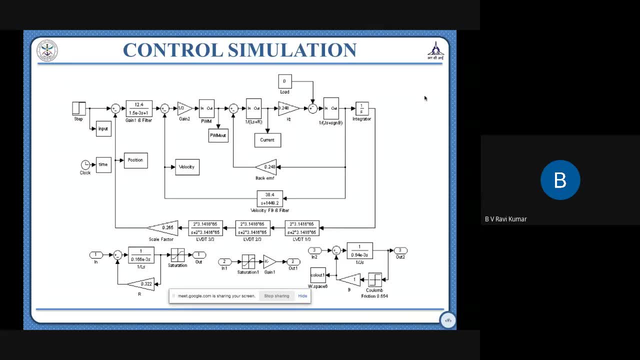 in the total current raising. so that has to be able to bring out in the three-phase modeling. but this is, i think, old slide. it was same like that. but this type of simulation first we have to do from where we have to arrive at the actual parameters and we have to go for the design. 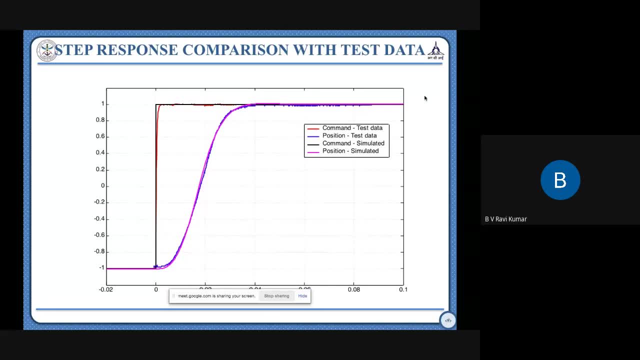 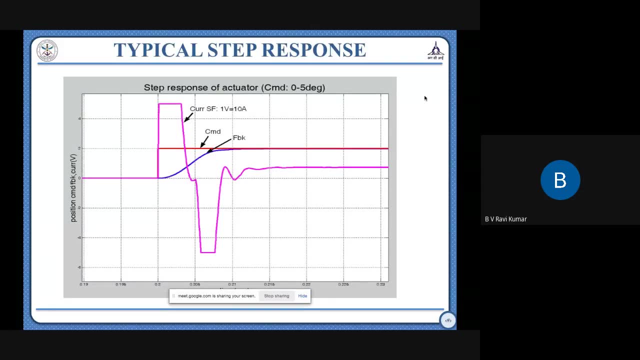 these are the simple step response, the actual hardware and final model. so this is different. uh, this is what i am telling. currents, the current requirements, will be very high during step response and we have to handle this type of currents frequently. if you are going for a very continuous type of step commands- and this type of step commands are very much- 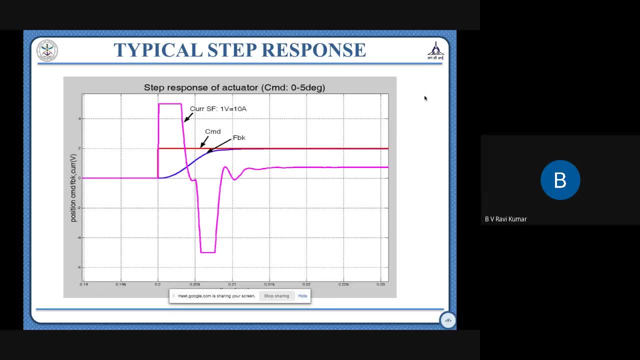 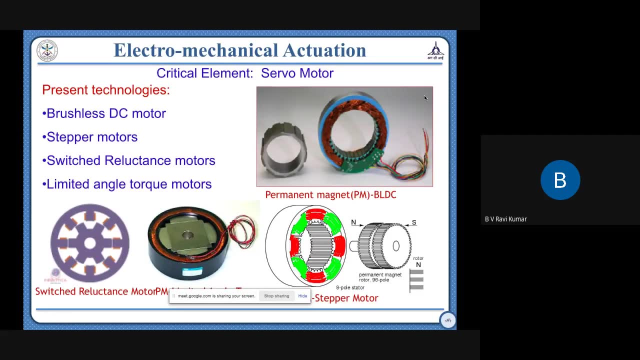 required, which is very much expected in the actual flight conditions. now we will come to the critical element: what are the present technologies and what we have to do? so come coming to the brushless dc. i think now brushless dc motor as a research, i think we can make it as an absolute, because 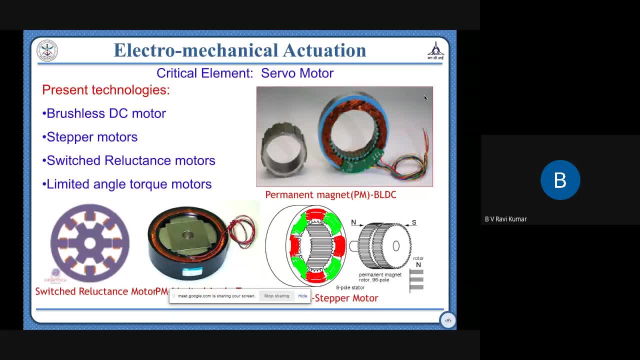 bldc motors are completely coming to the evs, electric vehicles and people are even industries also well matured on this. so there will be, uh, we can say almost- bl? dc motors, we can say at the budget of absolutely in the research point of view, commercially people are coming now and they are 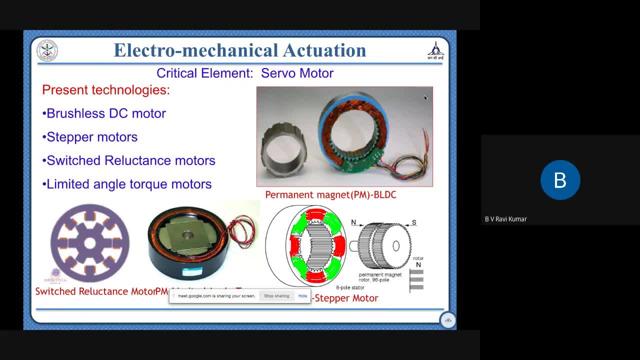 using for evs. definitely there is a lot of requirement, but i'm telling from research point of view. stepper motors, of course they are coming now. this is a lot of research and i think we can make it as an absolute. because we can make it as an absolute, because we can make it as an absolute because 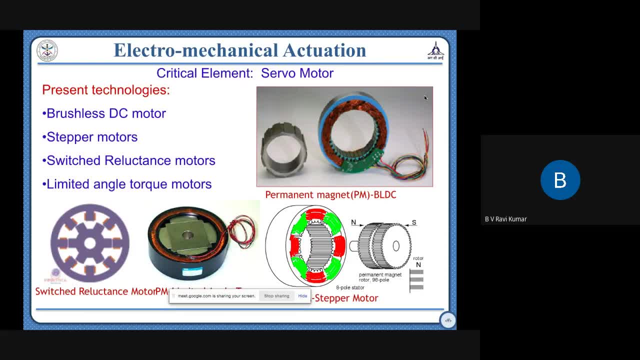 these are also very uh used wherever the open loop requirements are there. next comes the switchable trans motors. in fact, this is not a present technology. i might have made a mistake here. srms is one of the area which is very much required for servo application. normally nobody. 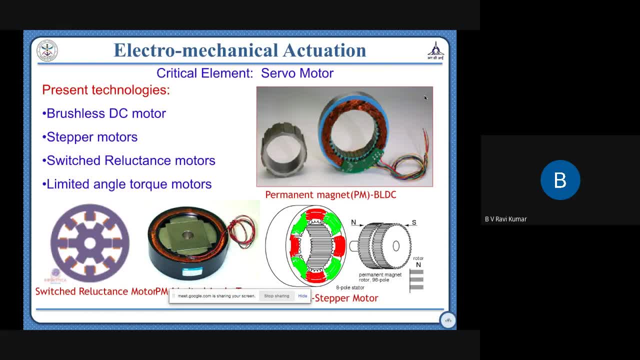 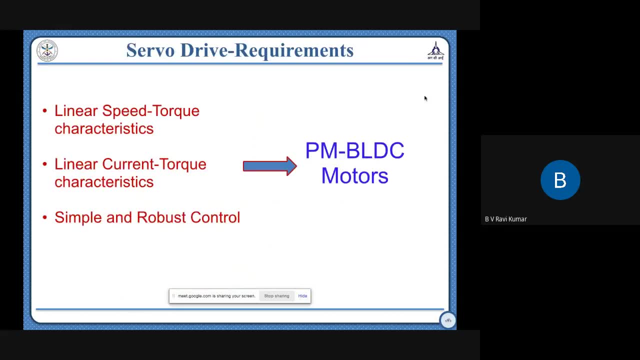 tried it for a servo application, normally for evs. they are doing it that also come to the next slides then why? we will ask why bld sims are so famous. because what is the requirement for a servo drive? is it should have a linear speed or characteristics, it should have a linear current. 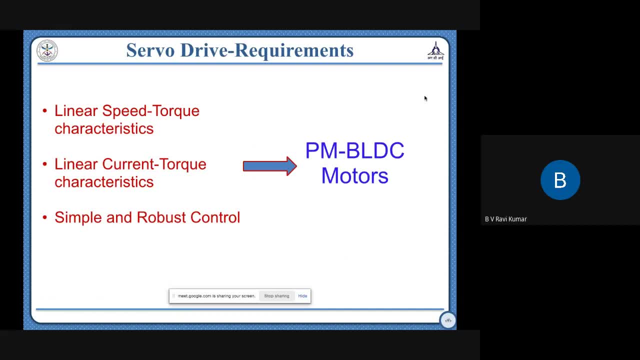 or characteristics, and simple and robust control. all these things are possible with blz. that's why people are not just moving away from blz, because, as far as i know, i joined in 2001 in rci and right from day one- 2001- actually first time- we imported a motor from outside and that we started our own. 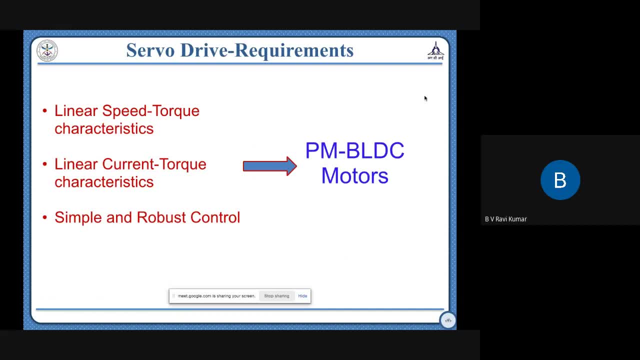 design in 2002. from there onwards we are using same blz motors with little bit improvements in terms of design, but not in terms of technology. but definitely now industry is well matured when when we started industries, nowhere in blm and blg motors. now all industry in fact in hydra but itself. we 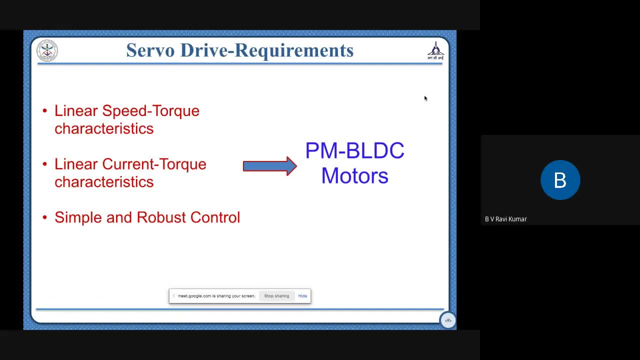 have some few industries which are doing village motors. based on our experience they are doing and even they are doing for evs also. but why people are not moving bls is because of these advantages, but at the same time of course i'm not showing any disadvantages. of course i'll come to 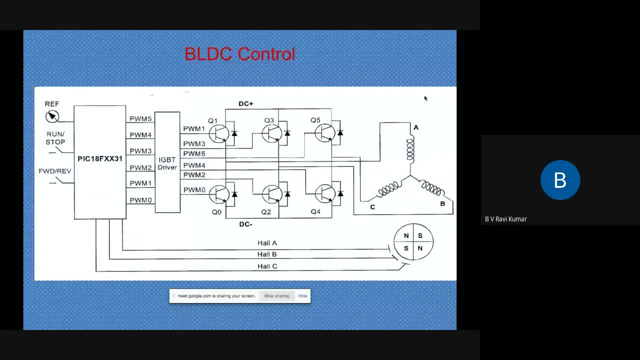 that. so i'll just take another. uh, 10 minutes, is it okay, dr pradeep? am i running out of time? any other question, dr pradeep? yeah, it's okay. uh, just five minutes, i'll come here. so then, uh, which type of action system? 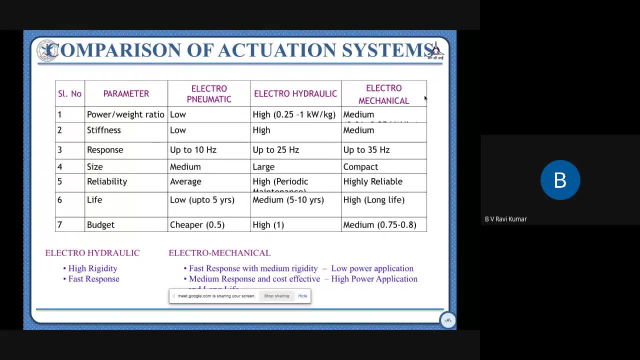 should, we should? i use this now. by this time you should be able to understand that for a high power you have to go for hydraulics. for stiffness- high stiffness- you have to go for hydraulics. so these are the desired wonders of electromechanical, which definitely from. 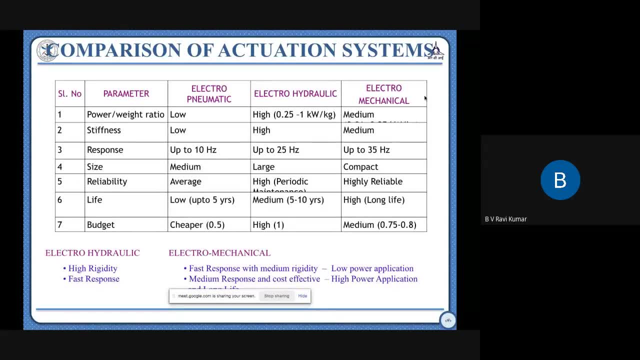 power, electronics, whatever control techniques i told we can overcome that response. of course electromechanical- we're going up to 35 heads and size- is also just compact compared to electro hydraulics. so the normally in fact, to put these uh comparison chart essay, we can say for all missiles now we are using electromechanical, not only india, all over the. 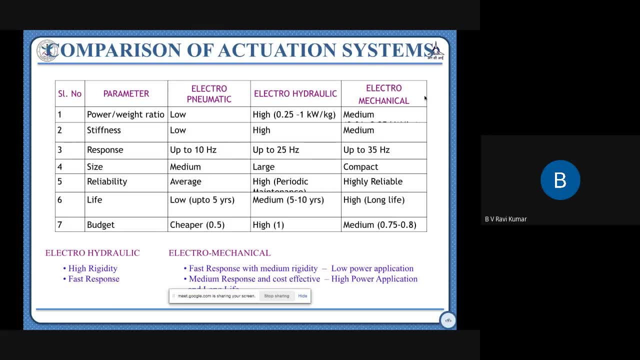 world. coming to the launch vehicles, people are using hydraulics, but that also they are shifting to the electromechanical. so we can say aircrafts, people are going for actuation system and it's a electrical action, that's electromechanical and propulsion, which we are telling all aircraft. 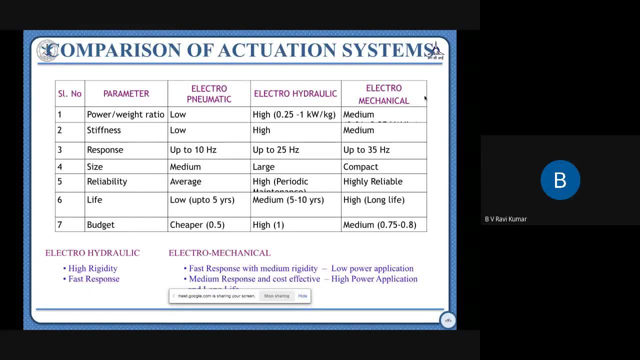 at least for the passenger aircrafts with the short distances, even for propulsion it's going for electrical systems, so it's a complete electrification. as we tell in electrification of transportation, same thing is happening in the air also, so aircrafts also becoming all electric aircrafts. we have a loitering missiles which is completely electrical. there is no chemical. 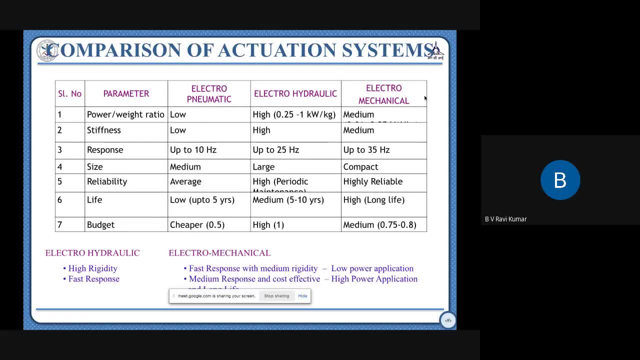 propulsion. that is the one of the area which is very much required. it's a complete electric propulsion is going on. so power, electronics and mechanical machine design plays a vital role in all these things. so electromechanical, the major disadvantage from this layer, you can say the power, but that can we can overcome with a combination of. 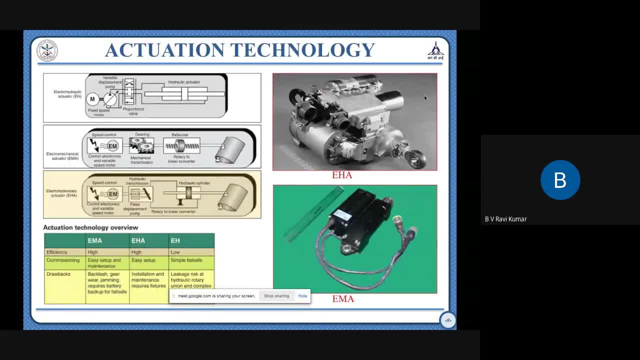 new designs which i'll just show i have. i'm showing you only, i'll be showing only one or two topics, but there are a lot of topics which definitely can be worked on. this is one more technology which, of course, i kept here, but it's a electro hydrostatic actuation system in which you use 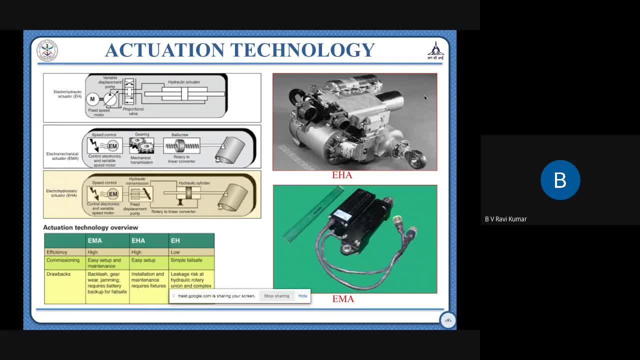 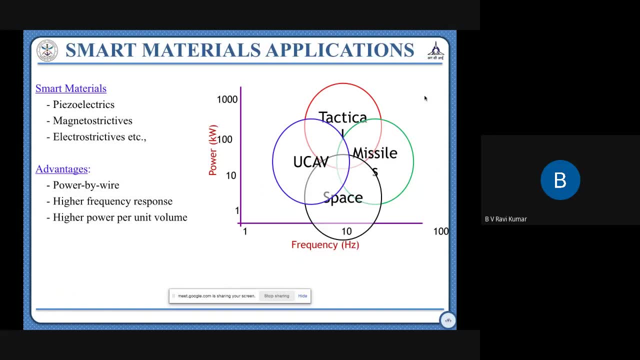 an electric motor for the control of pump, but obviously this is also not people are using. they're going for complete electric. so this is one of the area which, in fact, i'll not touch. it's a smart materials. now we'll come advances in future, so this year we'll spend 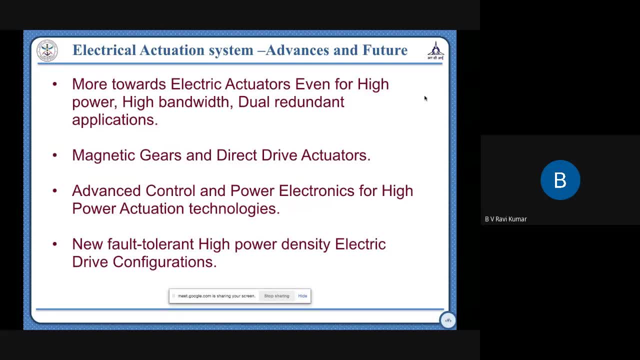 a little bit time now- more towards electrical actuators, even for high power, high bandwidth, dual redundant applications. so this is the requirement, because now we want to use the action systems everywhere, electrical actions even for space launch vehicles, where we're telling high power. also we'll go for actual systems, electrical only because of its advantages. next important: 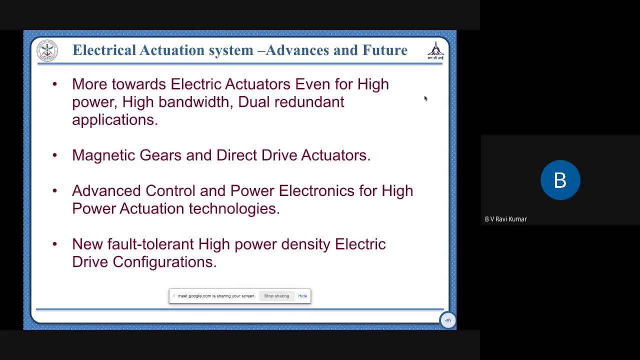 thing is that we're going to be able to use a lot of electronic devices and direct drive actuators. so here you will get a lot of topologies and machines, especially transverse flux machines and 3d flux machines where you can go directly for direct drive applications and magnetic gears. 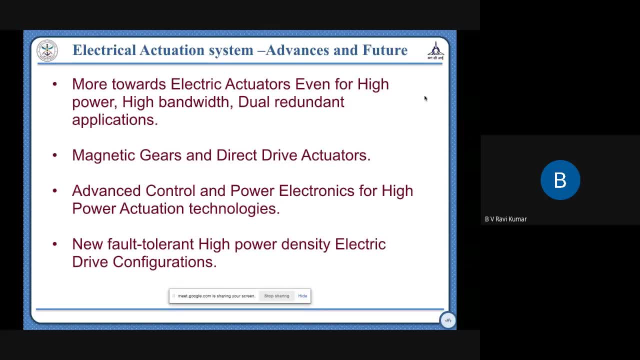 which is a very hot topic and a very interesting topic in terms of magnetic gears, where you can completely eliminate electro, electromechanical- yes, sorry, mechanical- gears- and you can get- you can have more advantages in terms of efficiency and backlash can be removed- an advanced component and systems where you can combine the power electronic power inverter within a boost converter. 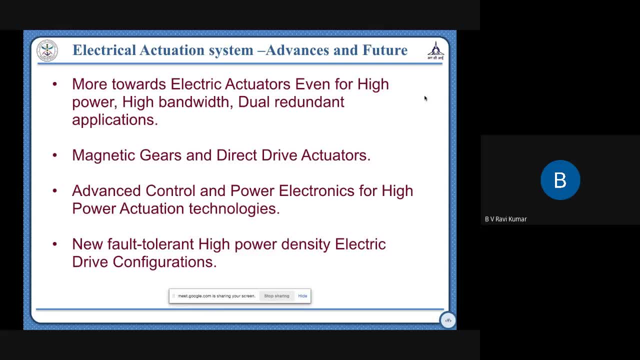 to improve the voltage requirements, as normally done in the electric vehicle. same thing can be applied for aerospace vehicles also and new fault tolerant, high power density drive configuration which is very much required for aircraft propulsion where the redundancy is a must. so these are the areas which has to be worked and which where the power electronics control. 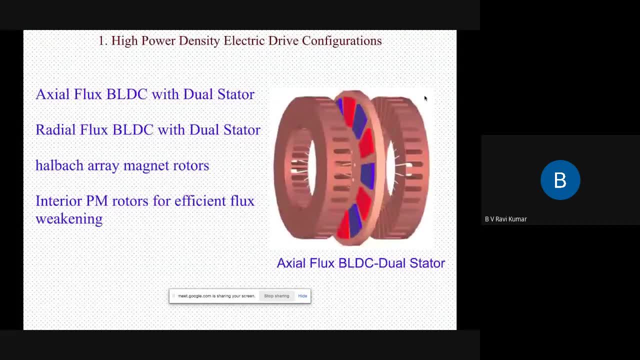 and electrical machines plays important role. now, coming to the drive configurations, you see in this example here the и g flex materials, which normally china is doing a lot of activity on this and unfortunately, india a lot of motors. i can say we, a lot of models are being for electric vehicles, in fact a missile complex. all these things we are doing. 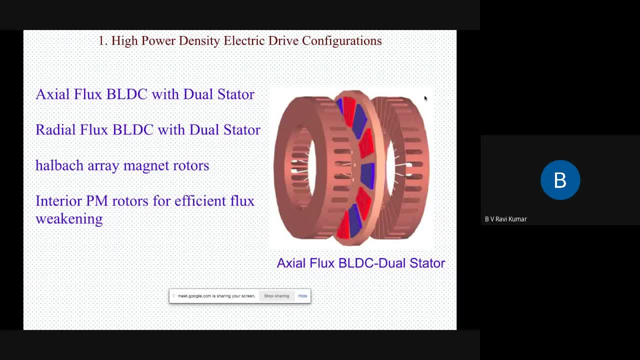 but for electric vehicles, people are totally residing in the outside world, and especially for drones and this type of application, because ultimately, the next generation will be the drones, where everything is coming from outside another. because we are making one of such applications where the 例- having so much technology with us, so much of human resources and, uh, we have a lot of academicians and 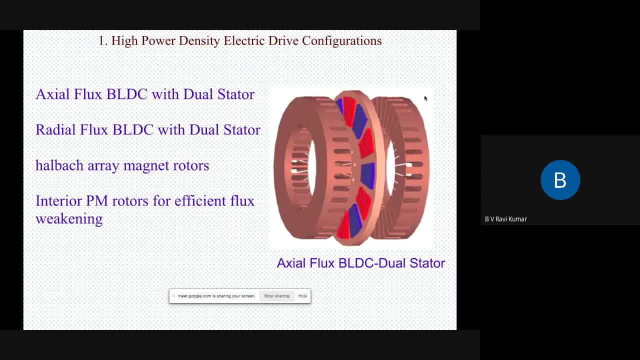 a lot of students are coming out from iids and ias and nids. still we are depending for the machine design and fabrication and this type of technologies outside the world. that is one of the part which, as an industry, as an academicians, we should work out and bring our own technologies. 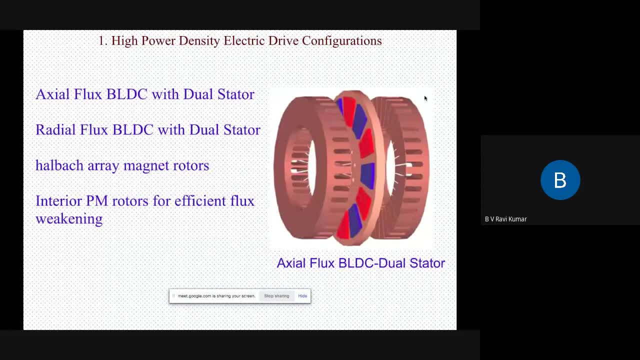 in the market. so excel flex bl is. the only limitation is it's a material which normally soft magnetic composite should be used. but there are research organizations like arca where they're using the smcs for developing this type of machines and this will be useful more for electric vehicles. for aerospace applications this may not be that relevant. 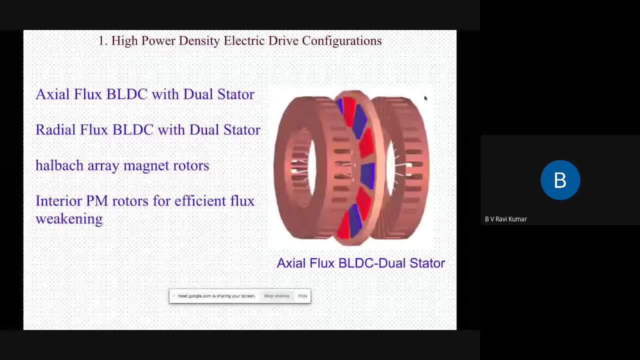 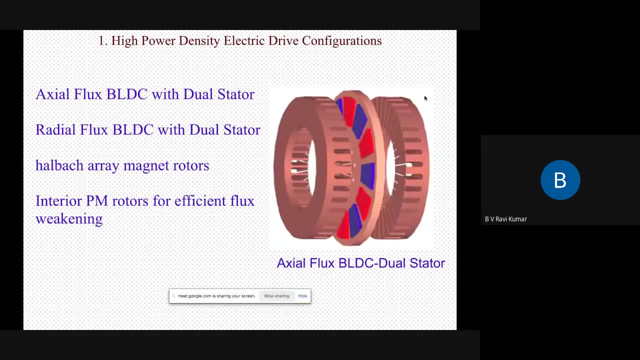 but it's very much used for electric vehicles and which is a very much important for novartis industry because all industry is moving towards evs and halbach mario magnet motors and interior pm motors for efficient flux weakening. so these are the major areas and of course this i will not. 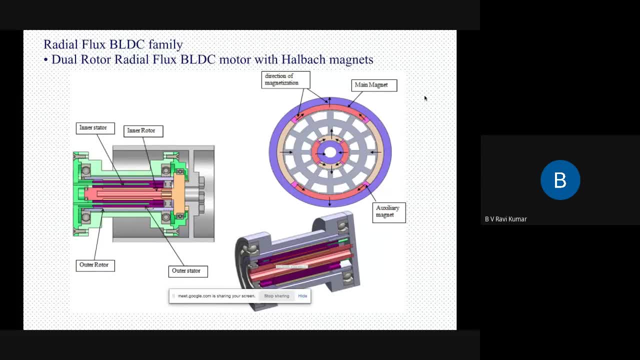 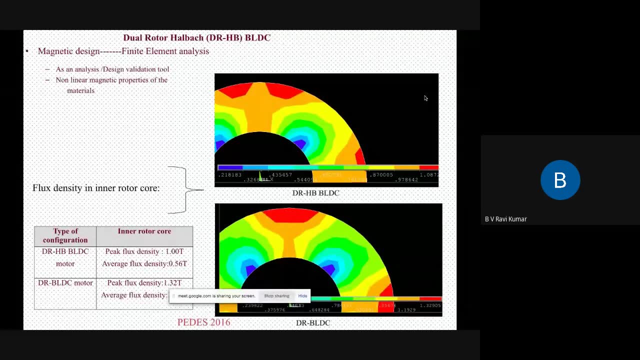 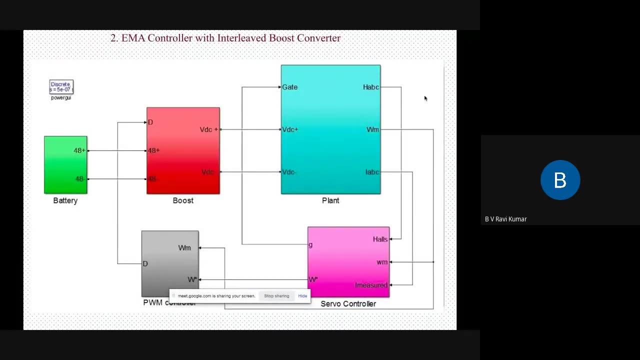 touch much upon this because of the time is, i think, running out. i'll just go through this, one of the area where we have used a dual rotor halbach blz motor which will be used for increasing the efficiency of the machine. so now this, i'll just spend small time the what i want to say is the controller combined. 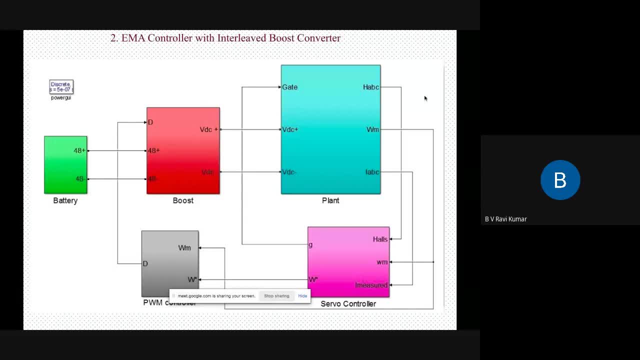 with the boost converter, because such type of things we have to do it to make action system useful for high power applications because for especially for aerospace. it cannot be used for a normal industrial electric vehicles, but aerospace. what is happening is you have to have a high power system for high power applications because for especially for aerospace. it cannot be used for a normal industry or electric vehicles, but aerospace. what is happening is: 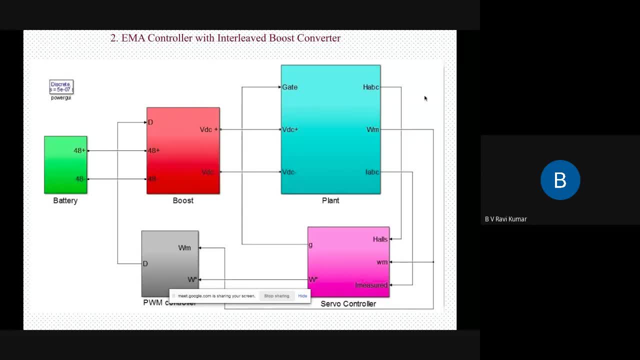 the requirement of the velocity will not be much. the velocity requirement will be where, whenever there is a demand from the obc or onboard computer based on the vehicle dynamics. some missiles may not be continuously requiring that velocity. for that we no need to carry a very high voltage battery. we can have an interleaved boost converter with a very high frequency gang. 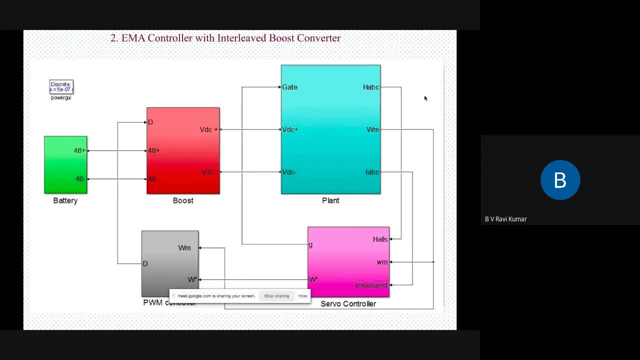 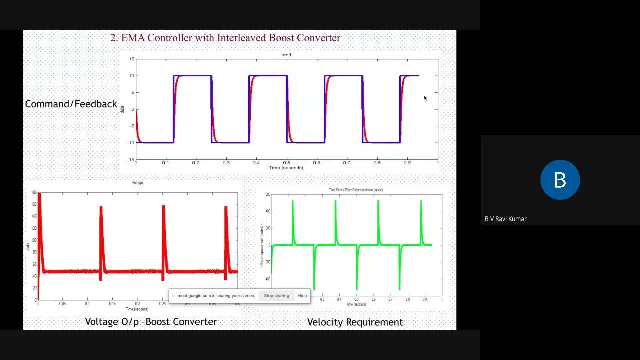 devices, or you can use even sscs also, and we can use a boost converter to boost the voltage based on the voltage required, based on the speed requirement. that is what this type of combinations can make total systems some useful for, even for electric propulsion applications. so that is the point in showing. 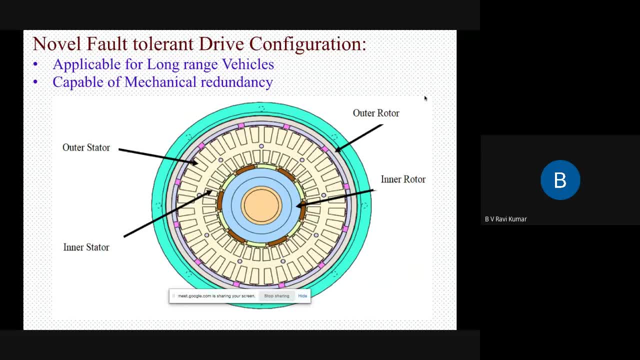 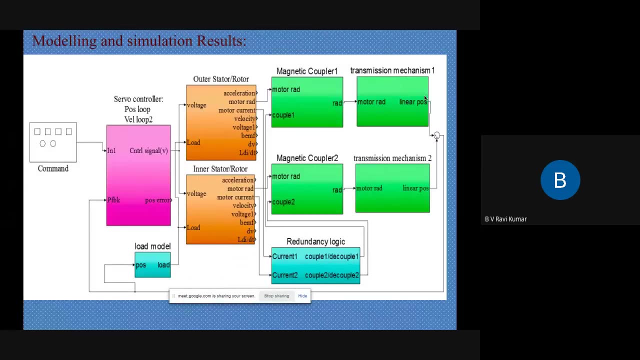 this slide and fault tolerant applications. these are the one of the fault tolerant application which we have done for a different various missile application where we can use it two starters in a single housing so that the switch, the status, can be switched based on the fault. so these are just to go through it. these are some simulation results also. i'll just go. 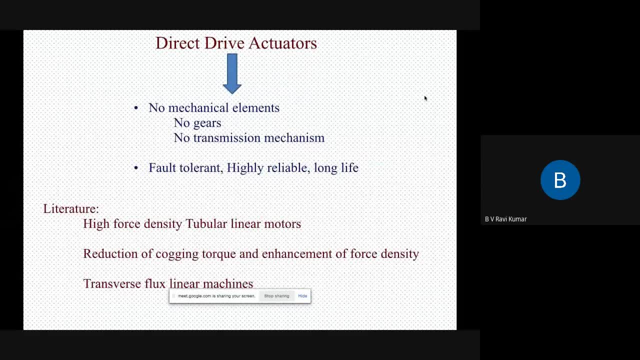 now i'll come to the direct drive actuators, which is a one major area, especially for uh. here, if you see the literature, there is a called a transfer flux machines, which is very much required for a direct drive actuation systems in missiles or in aircraft applications. 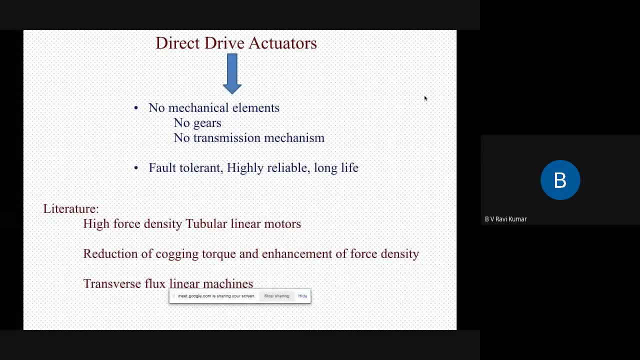 because you don't require, frankly, any transmission mechanism. you can go directly as an electrical thing. we don't require any mechanical elements. so no gears, no jamming, no backlash. so all those things can be overcome. if it is a direct drive configuration, for that you have a high force. 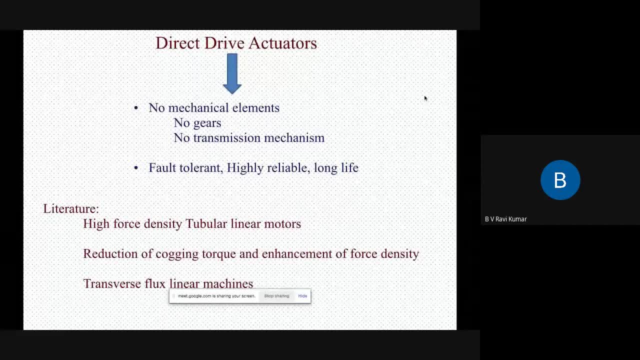 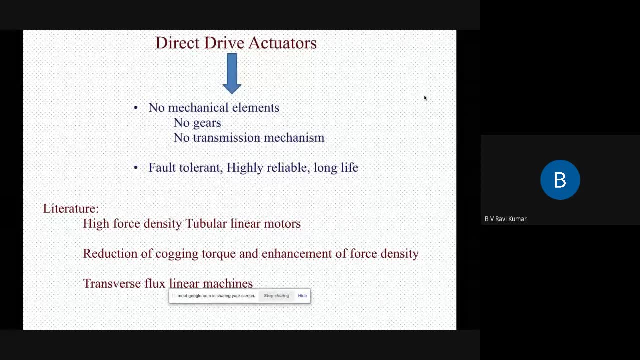 density, tubular linear motors and the reduction of cogging torque and such a of techniques can be employed and major thing is the transverse flux machines, where we have to use a 3d, which we also call as a 3d flux machines, or we can use smcs, soft magnetic composites. 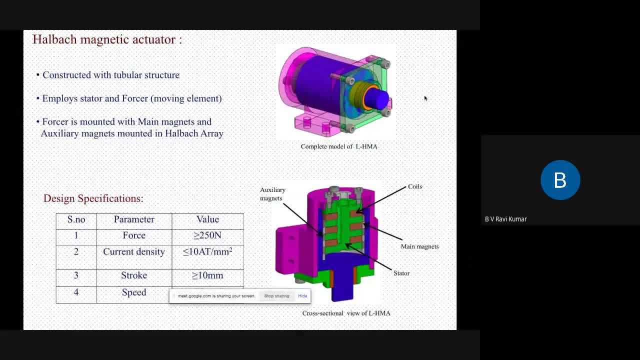 this is one of the actuators which is developed with the hallback concept. this is a very famous concept which nowhere has all the western world already shifted to this type of designs for aircrafts. so this where we can improve the power density of the machine, this is just a. 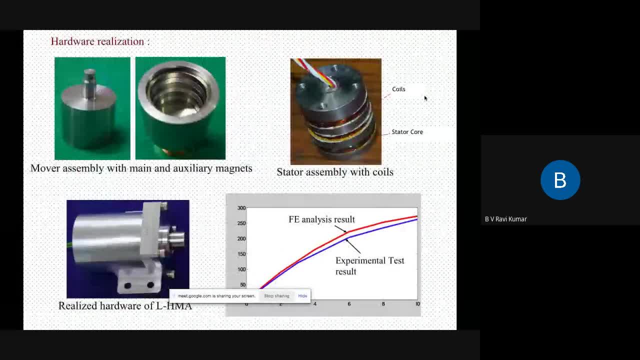 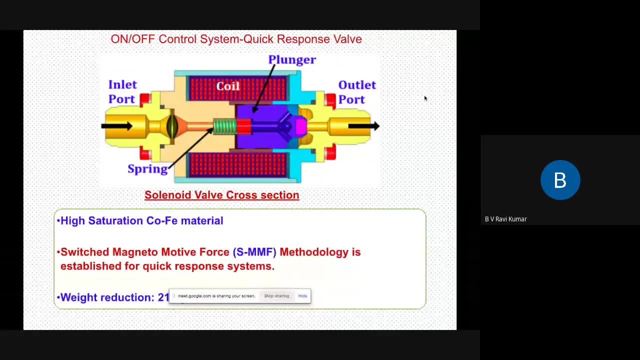 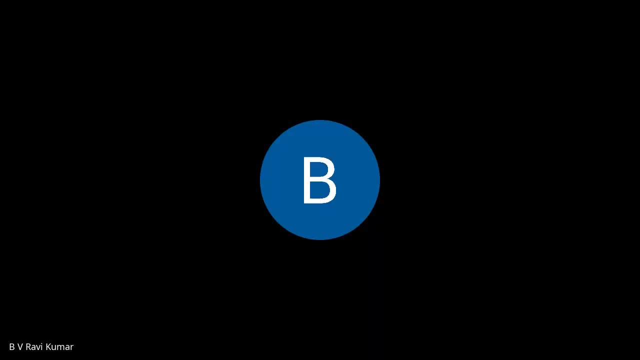 design flow chart which is equivalent to any machine design. so these are the different hardware components which we can use to improve the power density. now this is the slide which i just wanted to show you, which we are calling, which we are using for important projects which will improve. 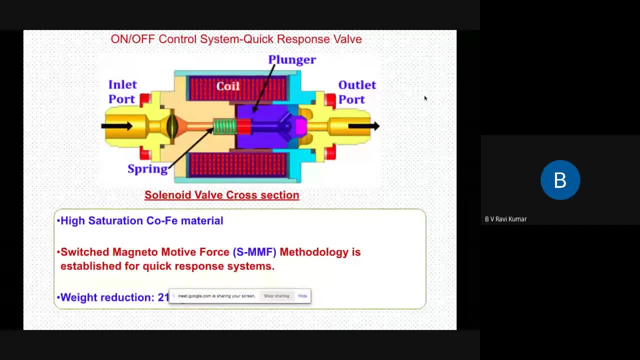 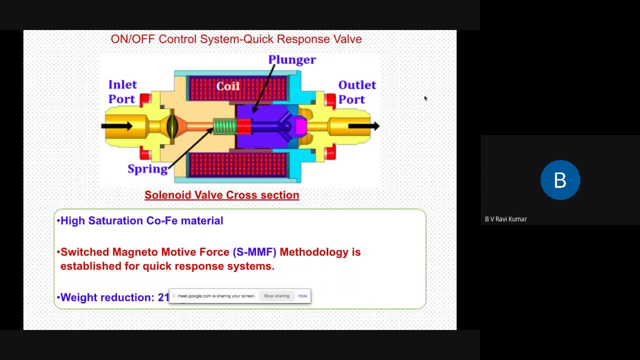 the performance of the valve by using a simple technique of switched mmf, because if you take a stoner valve it looks like an overcome mechanical element, but if you go in depth it's a more electrical engineering is involved in it. the major thing is, by using this concept, we could able to 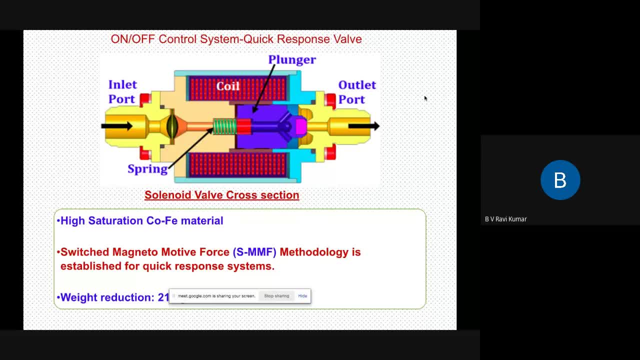 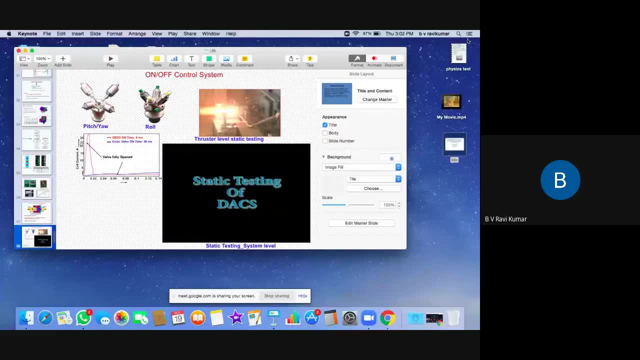 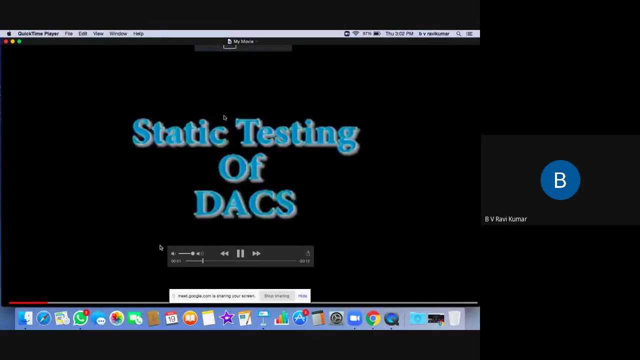 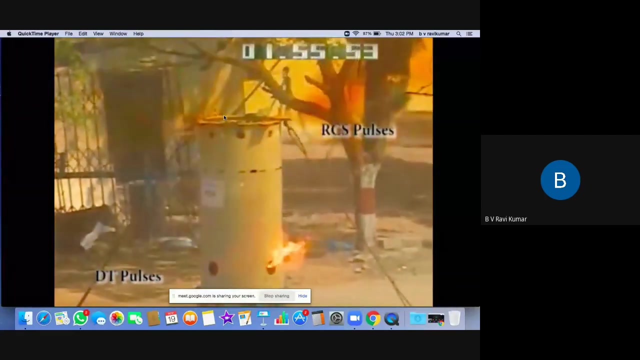 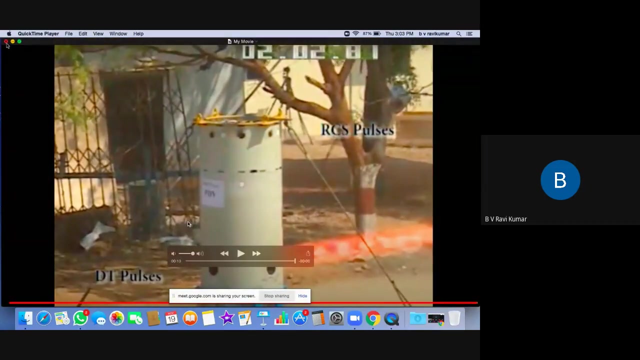 improve the power density of the machine and as well as the response times are reduced from 100 milliseconds to 6 milliseconds. so this year, one small video i'll just show you so that you can appreciate the way of happening in the actual design. so this is what i have shown is this is what we are calling is on off control system. 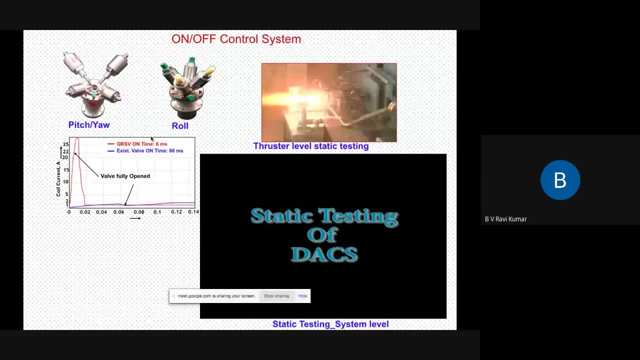 where we use valves, electromagnetic valves, that is nothing but a solenoid valve. here, what we have done is a qrsv on time earlier. it is around 166 milliseconds, which has reduced to six milliseconds, because of which we could achieve the complete kill probability of the vehicle. 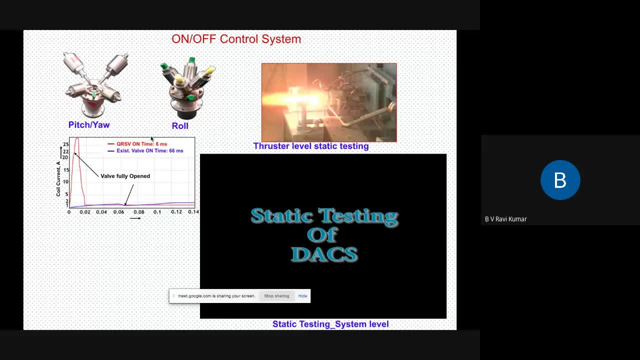 the complete maneuverability of the vehicle increased because of the reduction of the time. that means the response time has been improved by design of the vehicle. the response time has been improved by design of the vehicle, which means the response time has been improved by design of the. 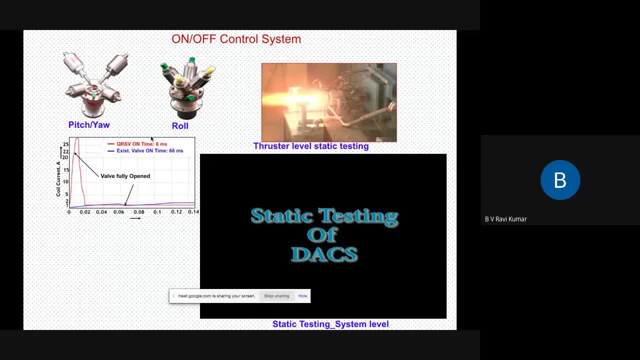 of the magnetic material by design of SSMF, by which the current is controlled in the valve instead of pumping a constant MMF throughout. we changed the MMF because the reluctance is varying in terms of the sonar wave. It's not like an electrical machine where the reluctance 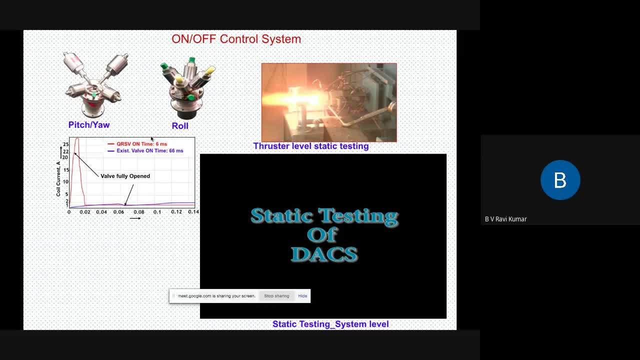 is constant. Here the reluctance is varying based on the plunger position, because of which the MMF can be switched based on the requirement. By doing so, the complete on time has reduced something like 66 milliseconds to 6 milliseconds, because of which the complete controllability. 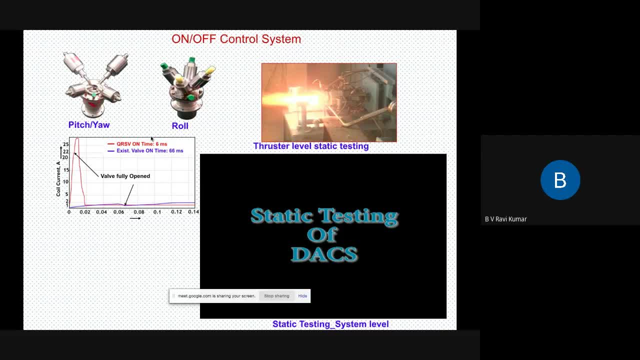 has been achieved, and it has been excellent performance in terms of actual flight. So this is how. this is just a small application. this is what I want to show you is the combination of power, electronics, electrical machines and control system can do lot of things in. 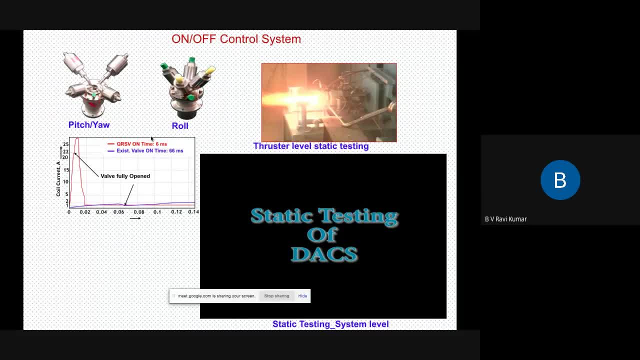 aerospace industry. Nowadays, all aerospace industries are moving from actual conventional hydro hydraulics to electrical and there are lot of requirements. In fact, there are lot of things where, from the DC-DC converters, all those things are there which are not present in here. 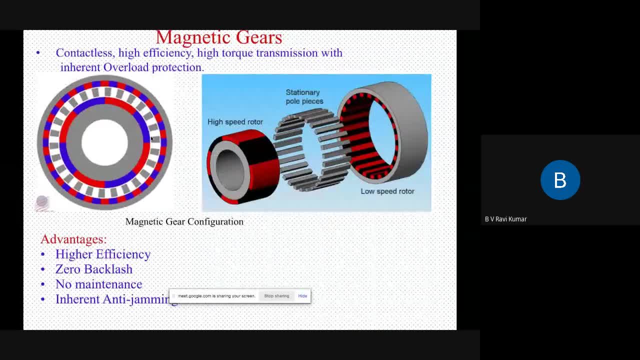 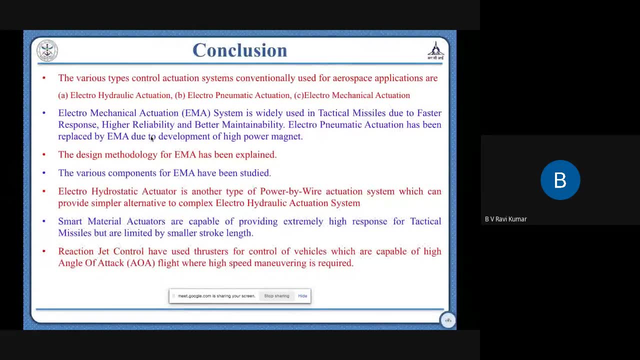 But that Back down. that's what I want to tell you. Of course, these are magnetic gears, which I already told you. So that's all. So I just want to conclude, because I think I have already some 2-3 minutes over This. I just covered. 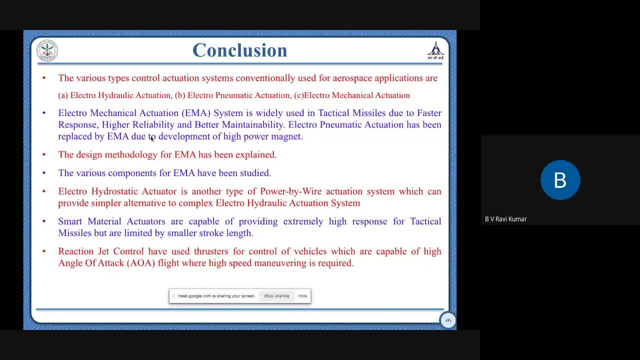 about different type of action systems and what is the design methodology. Probably I have not gone in depth about the design, just I have shown you that what is the important areas like electrical machine design, power, electronics. also I have not gone much into the device selection and the gate rails, circuit design, all those things I have not gone. But 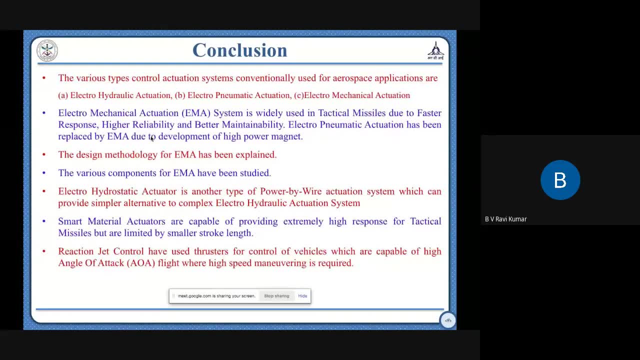 that is very much required, which I can definitely. next time, If I have opportunity, we can talk about that. And what are the new things we want to work? We want to work about the combination of different things like power electronics, inverter, as well as boost converter and actuation system, with the different type of machines and going. 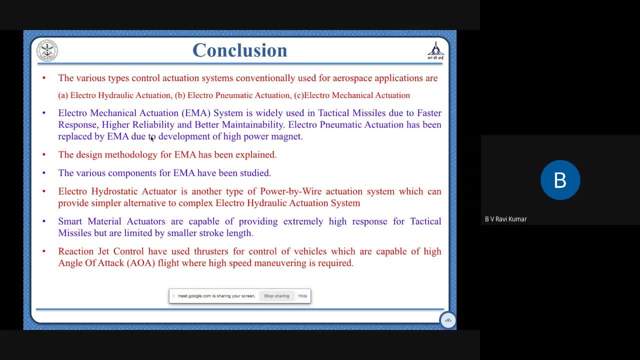 for multi-phase machines can type of things can be done in order to make action system more robust and more useful. in the high power applications, especially in terms of aircrafts, electric aircrafts, to make it all electric propulsion also, we can use this type of concepts. 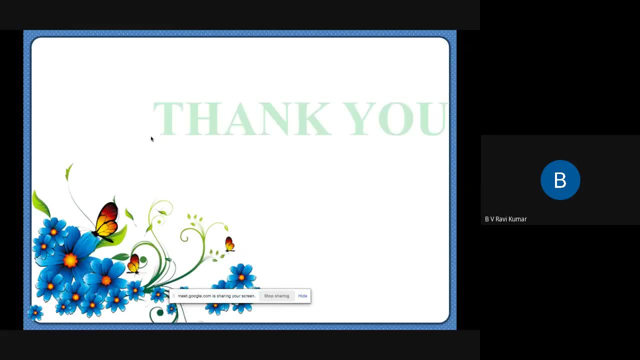 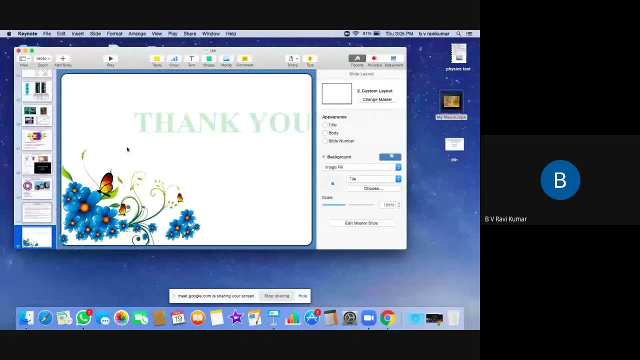 So that is the overall thing. So thank you very much. Thank you, Thank you very much, And if any questions are there, you can please ask. Excuse me, sir, Yeah, Can you tell me about the applications of sensors and communication systems in defense? 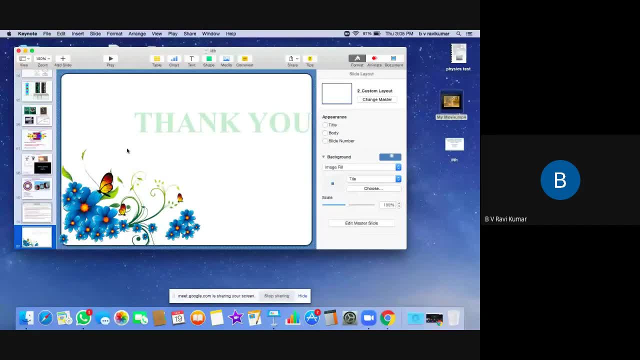 Yeah, Sensors. actually, if you take as a vehicle alone, you have a huge sensor requirement And in fact we are depending a lot on a lot of sensors. and also, the major thing, if you take sensor for guidance, Like, we have a IR sensor, infrared sensor- 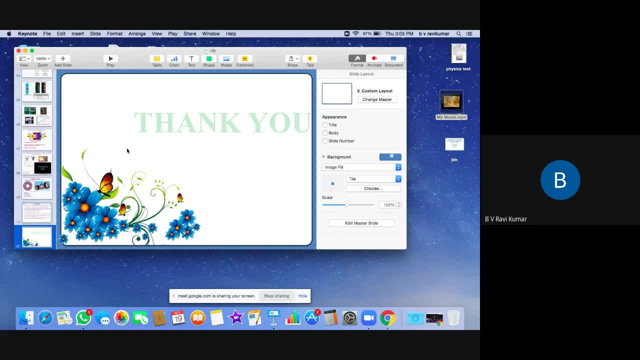 We should be using for the homing guidance application. We should have the infrared image of the target So that IR sensor, which is a very much signal processing and image processing oriented, That is one sensor which we require at the vehicle level. I'm telling you about the missile level. 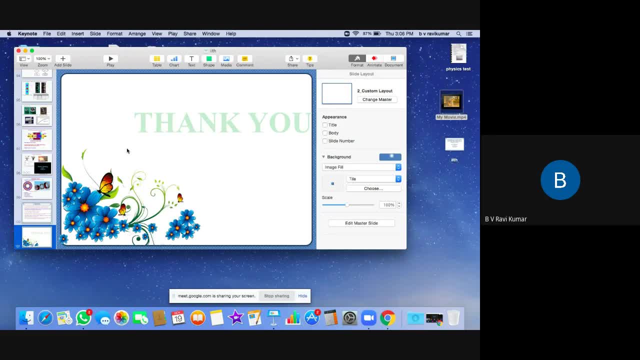 Next is the navigation sensor, which RCA itself is a pioneering navigation sensor department And we have done a lot of INS applications for different missiles. So navigation sensor, These are the main sensors at the vehicle level and coming to the communication normally as a weapon system. 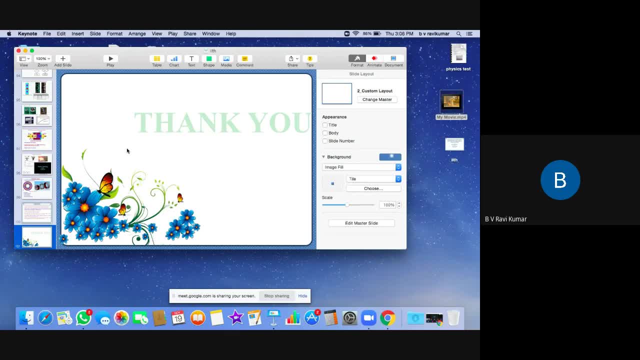 We have a lot of communication requirements because if you're flying a missile as a weapon system, I'm not telling you about the onboard communication, I'm telling you the communication with respect to the radars and communication, wireless communication. It is a very much proven. 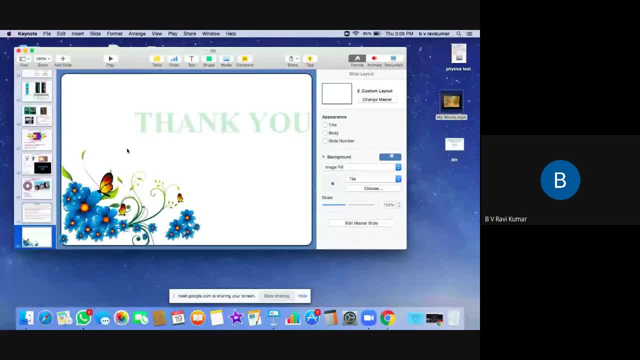 We have a lot of requirements because the data rates- what we are talking- will be of very high in order to get the better data from the radar for our onboard competition. and coming to the inside actuation system or inside the onboard communication between the onboard computer. 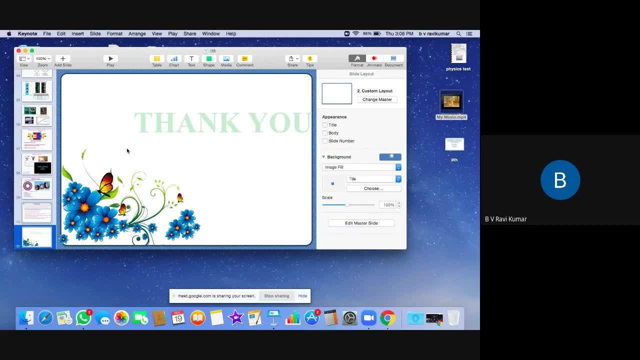 INS And our actuation system. we use normally different type of communication. One is the mid standard. 1550 is one of the communication where we use it because it's a robust enough And it's a dual redundant communication that is using. normally we use this type of communication. 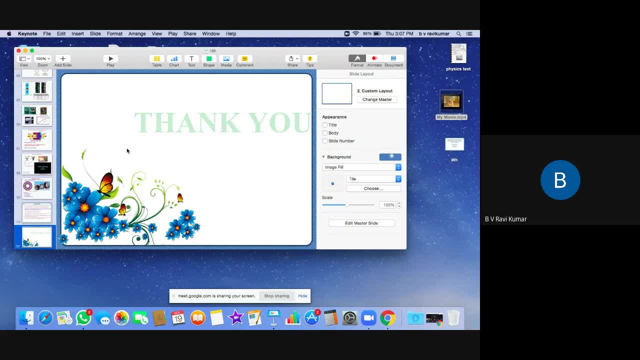 All of the missiles coming to the communication and coming to the sensors. at the actuation level, we use encoders for position sensing and we use same encoders for velocity And we use a linear variable differential transformers, that is, LVDTs. 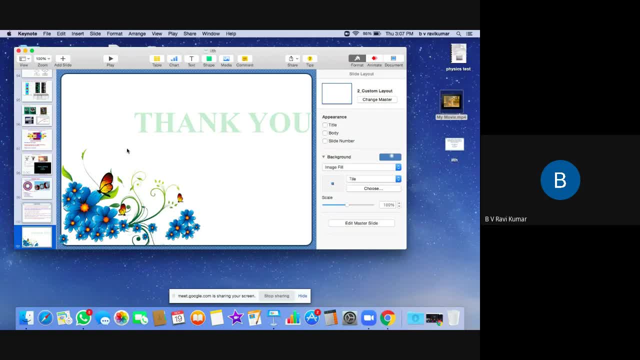 For position sensing, especially for linear actuators, and also we have minor to stick to sensing and we have minor encoders also we are using for some of the applications. Yeah, I think that's the what is it? Okay? 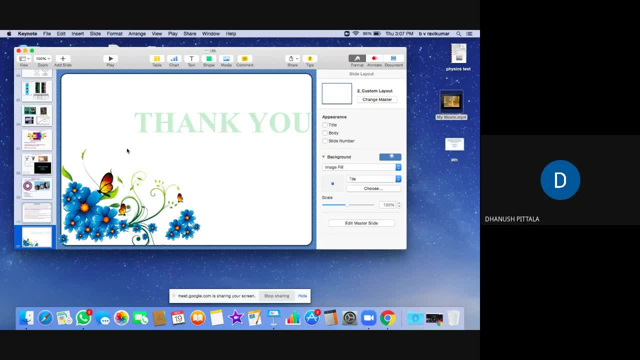 Okay, sir. So what are the knowledge? So what is the knowledge and skills do I require to work in the area of sensors and communication systems? Coming to the knowledge, basically, frankly speaking, I anything that knowledge we require. only major thing: what we require is a mathematical modeling of anything we don't really require, even if it is a power, electronics, even center the major things of physics we should be understood. 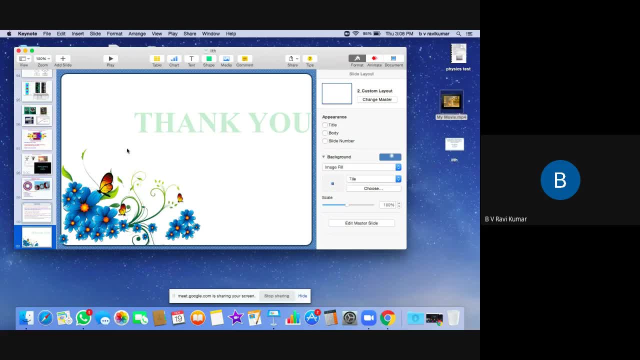 So the mathematical model. so right from your college days we should be always want students or the youngsters who are joining RCR DRDO. also we want the mathematical skills. that is very important because unless we model a system- because normally if a sensor was, INS is there- what we are getting from the INS is the acceleration rate data. 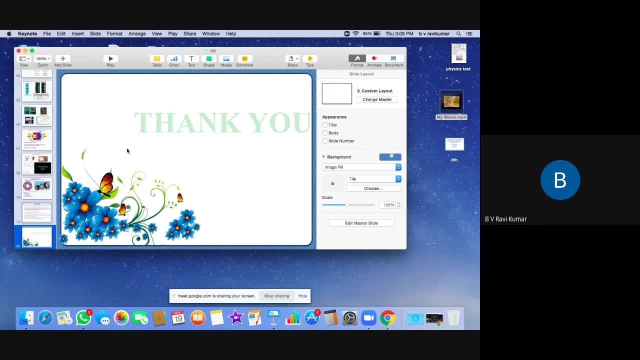 So the data we can extend. we have some code which already developed by predecessors. we have to. it is not that we have to maintain that code. the only thing is we have to model the system and for diagnosis. so such type of techniques is very much required. 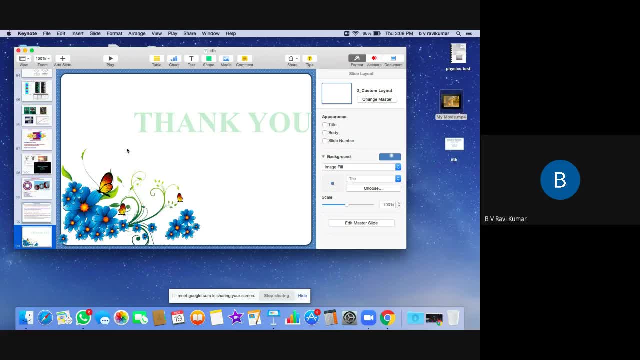 So, coming to the knowledge, probably, whether it is any background is electrical or electronics background, it is sufficient to work on that, but only when we come here. we should have that strong mathematical modeling skills to improvise on the existing system. So, sir, 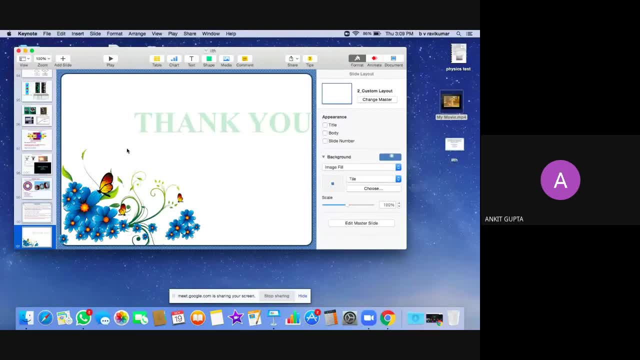 Yeah, Yeah, good afternoon, sir. I have one question regarding sir. I wanted to know like in order to join DRDO. DRDO is not recruiting MTech and PhD students, And so my point only was like: are there able means that, like you are working there for 19 years or 20 years now, your means like the BTech candidates which are coming joining DRDO? 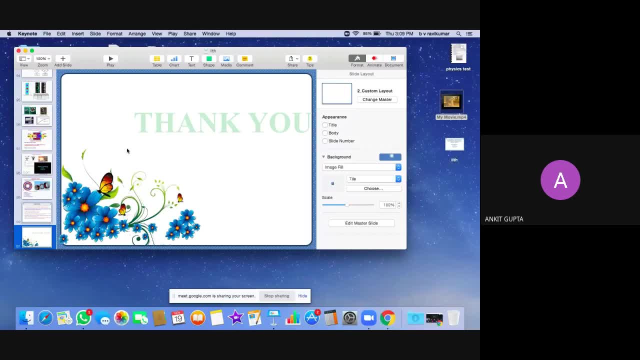 Are you able to. they are okay. that means you are able to manage okay, okay. anyhow, that is a good question, but i don't know, i'm uh, i cannot answer that directly because i am handing very few of them who are very good, definitely btechs who are coming first of all, we have our own type of what you tell. 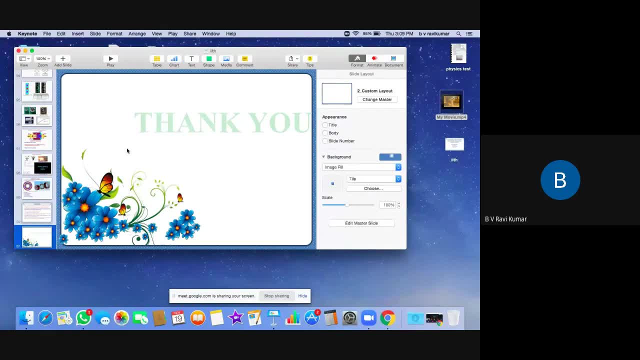 recruitment policy. probably we'll get a very good students. there is no doubt about it. it's only how we use them. definitely, everybody is expertise in one area. there is no doubt about it. it only depends on how we use use them. so and of course that probably is more related to the hr. 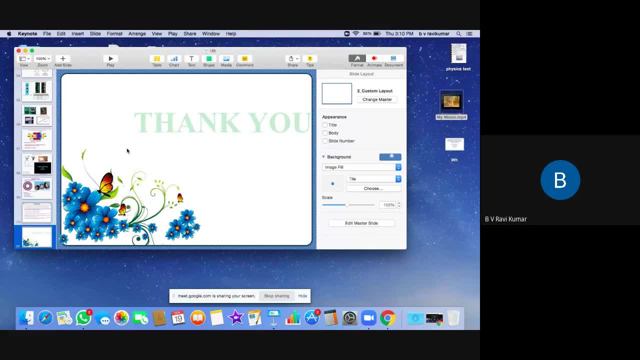 question. so, but as far as i am understood, whatever whoever are coming, it's not because everything is basic. so i don't think we are doing which is, again, it's everything from basics only application. so whether it's a drdo or isro or any other organization that questions remain same thing. 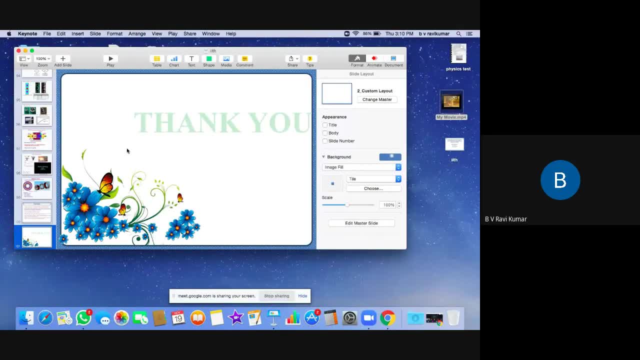 so probably depends upon the application, how the seniors use them. that depends on that. so that's all i can do. that's all i can do. Dr Avikumar, can i rephrase that question? yeah, let's say uh. i mean, maybe the student may appreciate this question. 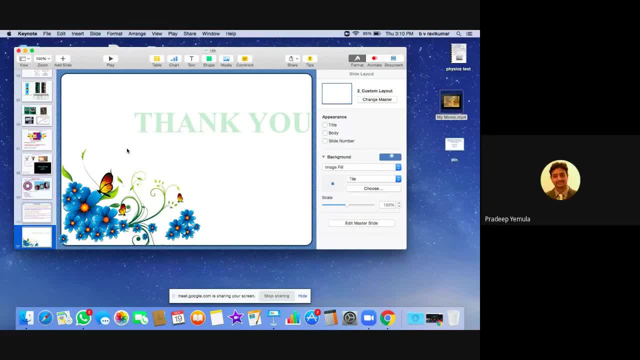 let's say, somebody has completed mtech. okay, now they want to- you know, contribute for drdo. yes, so how? how do they do it? because if you recruited btech, how can mtech or how can a phd person contribute to drdo? uh, compared to a btech. 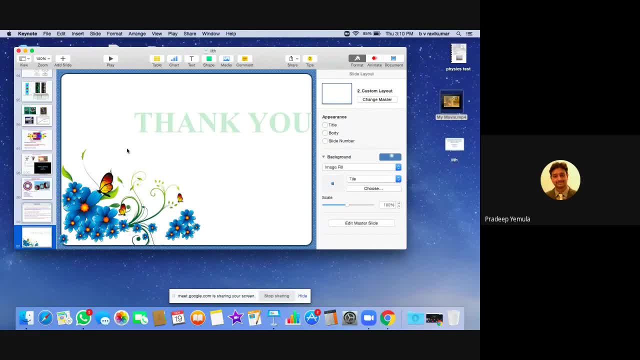 yes, not in comparison in in what are the ways in which an mtech graduate can contribute to drdo? definitely, because if you take a suppose i'll just an example: suppose mtech paul ganes guys starts joining in drdo, we have a huge requirement. i mean huge application orientation. 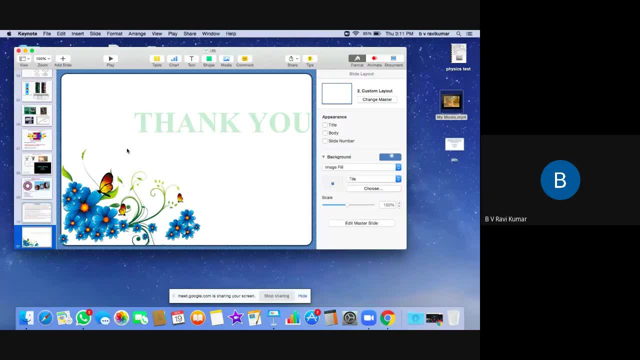 is because a lot of research is pending. in fact, i can say a lot of research areas are there which we are not having time to do. in fact, that word i should not use because time is already always be there- but it's, frankly speaking, because there are a lot of research areas. 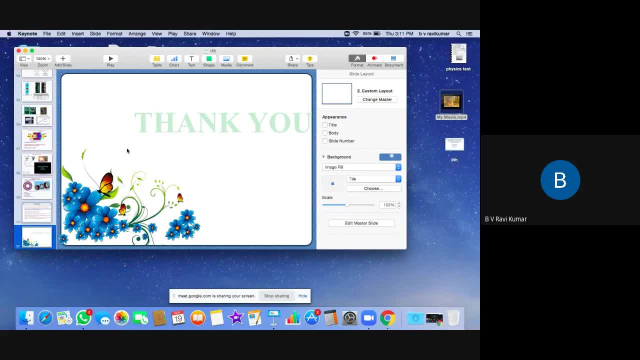 which we are not touched. in fact india itself is not touched. suppose, if you take electromagnetic propulsion, which are not covered here, it's a huge area where you require a lot of high voltage requirements and a lot of power electronics requirement, a lot of modeling and then from 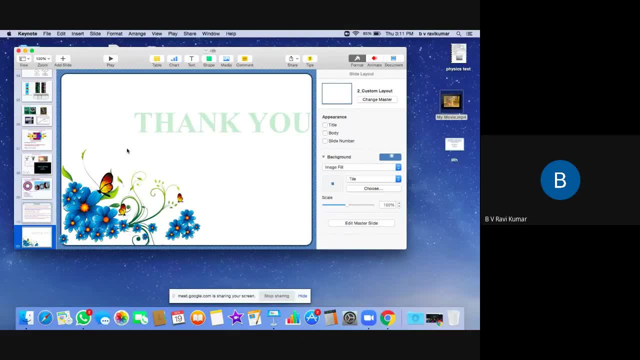 machine. also, you should design a very high speed linear induction machines or lennox linear bldc motors where nobody in industry has done, because for that application i've. i've gone throughout the india. i have already a lot of people have spoken, but very few people are in that area and they're also not up to the 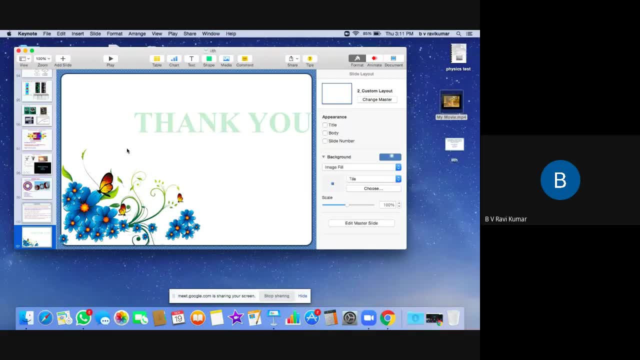 mark industry-wise, so from research point, that only we have to do so, only this as a research organization. drdo is ready to do a lot of things at the same time. we require the expertise from out, like youngsters has to join, so that expertise definitely can suppose a powderless guy use. 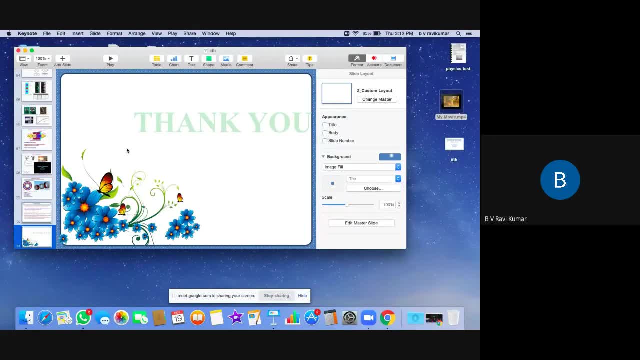 there are a lot of areas where we can utilize it. we cannot say one area, because drdo as such is handling a lot of technological areas which, as i have spoken, only a thing in a droplet in a ocean. what i told you so definitely it can be used in a different ways. there are huge. 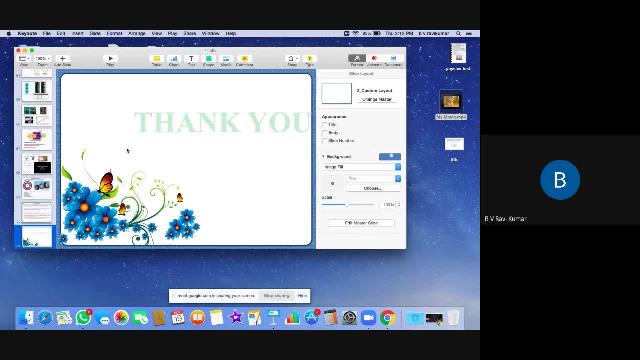 obligations, right from radars to missiles, to even tankers, to everywhere. wireless power transmission is one of the area- wireless power technology- where we want to make complete missile without wires because we want to, as i shown you that valves which i'm showing you, there are a lot of 40. 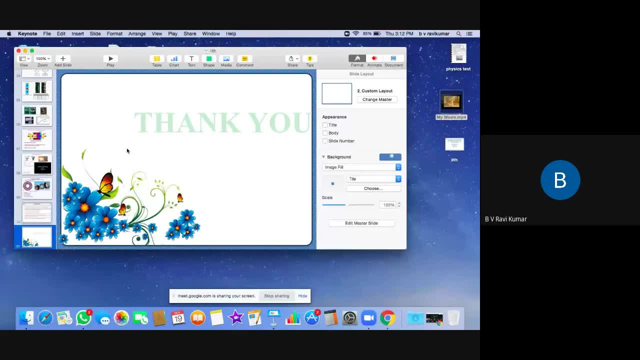 walls out there in a small space. so if you remove, remove completely wires to go for a wireless power, for a surface power transfer, which already university buffalo is doing for us. so this type of things, a lot of applications are there which can be utilized from whoever it is joining, whether it's a powertronics or control systems or any candidate. 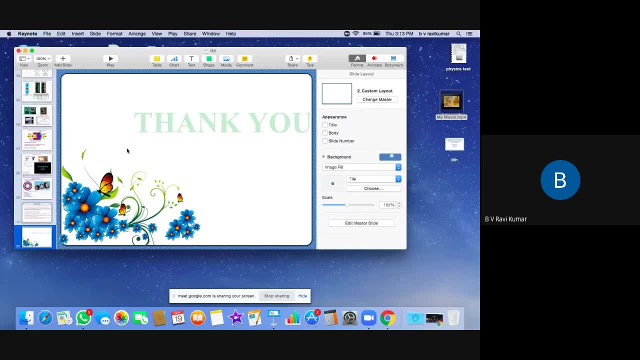 so hope i think i answered that answer one more. any other question? so one. one more point just i want to add: sir uh, like sir in the recruitment process of drd also, sir uh, there are very less vacancies for core electrical engineers. electrical and telecommunication engineers are pref. they are preferring more. any reason for that? sir? 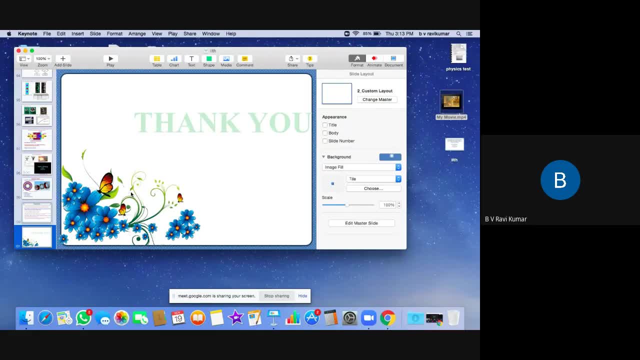 uh, actually this i can because i that's true. actually, probably that may be true, uh, but uh, that depends because, because drdo is a very big, i think i am not very much under the because drdo is having 51 laboratories and i am not sure that they are having 51 laboratories. 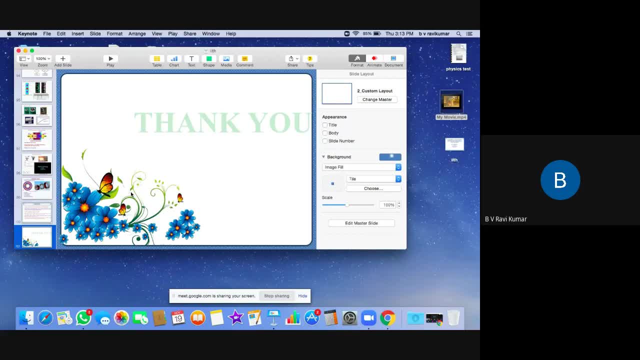 which we are using almost different technologies. so that will come directly from our director, delhi. so that requirements, that depends upon the thing, because as far as missile congress is concerned, we are having good amount of electrical engineers requirement. but whatever you are seeing as a advertisement or the recruitment that comes from the portal at a daily level, i mean all india level. 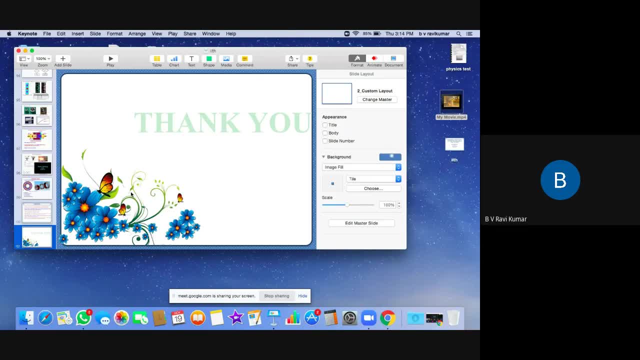 so that we don't know, because means i am not, uh, actually in authority to answer those questions, because i've also not known. but as far as missile complex- because i'm working for mizell- definitely electrical engineers is a requirement. design, we have enough people and people are. 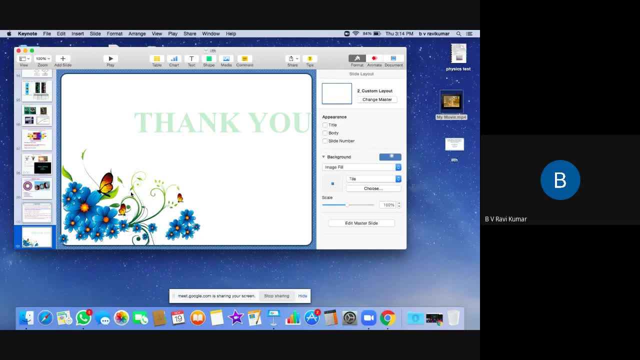 recruiting also, so that way. so you may be seeing probably the whole drdo. in that case it will be less. yes, because there are radar requirements, a lot of other requirements there where probably telecommunication, electrical, may be more fine. sir, thank you, yeah, yeah, any other technical questions? 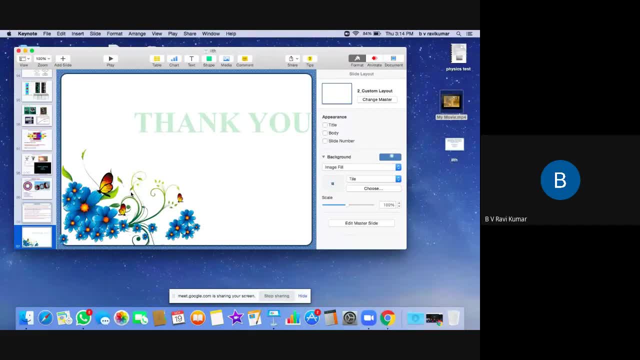 sir, how can we make use of ai in defense? yeah, that's a very good question. it's a very good question. so we have a lot of area which are forbidden. to tell you is only the robotics actually this in fact, already we have a lab in drdo which is working in- i think in bangalore is there, and also we have 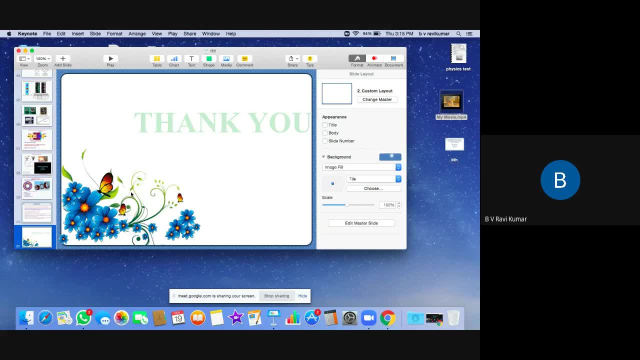 in our rca also on aaa center, where they are using a for robotics, where we are using a lot of uh. in fact i am not able to answer. i may not able to tell those things, but we are using robotics for different applications where the higher requirement is there and we have a set up a lab in rca also. 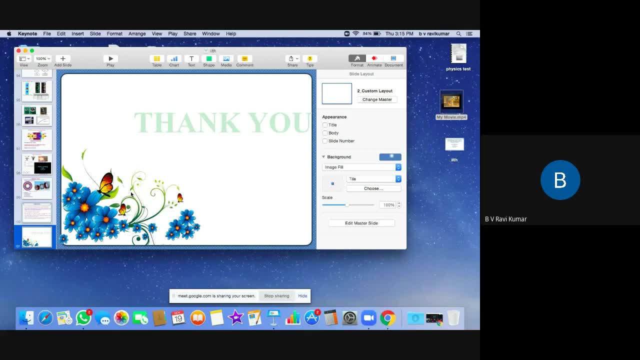 aaa application to the electrical machines also. we are doing because, as i told you, the fault diagnostics and fault uh tolerant electrical machines and drives, where we want to use an actuation system with a complete fault tolerance, there definitely a requirement is there. that is also one of the area in fact we have not worked on that. we have to work on that. but coming to the 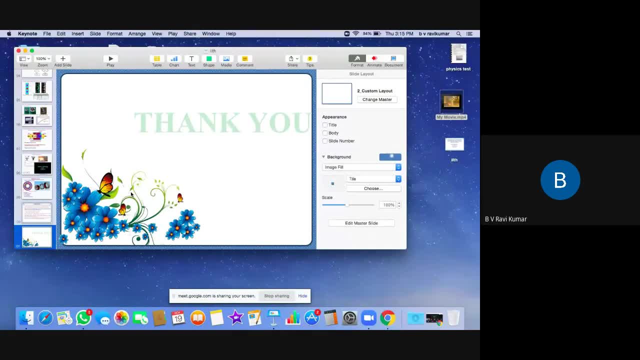 other lab. what i told already rca is that we are doing a lot of a techniques for robotic applications. yeah, good afternoon sir. yeah, i have one question. uh, sir, uh, can you please highlight, uh, what is the different operating voltage and current for the converters or the pneumatic systems, uh, which are? 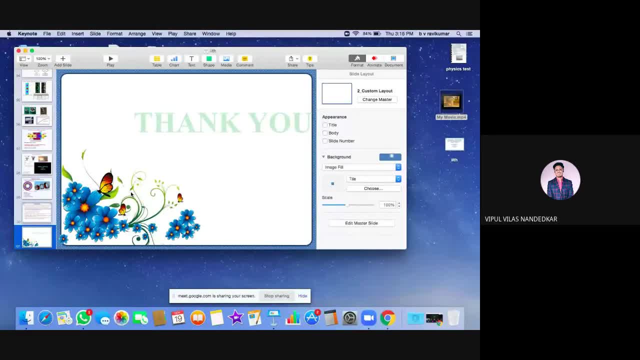 designed for the guided missiles such as prithvi or amni which you have highlighted? yeah, pneumatic or electrical. uh, yes, electrical systems. yeah, yeah, converters, power converters. so we normally have a lot of converters in the system. uh, coming to the in a missile system, coming to the converters. 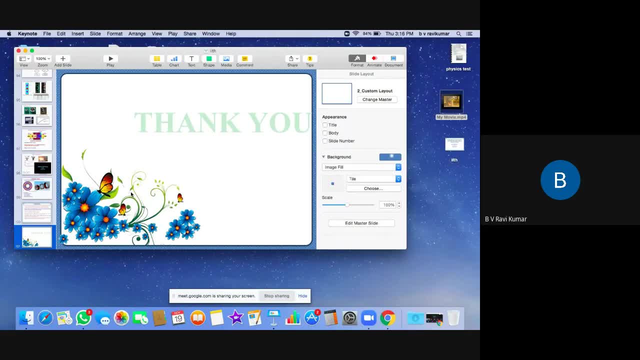 one is coming to the bl dc motor. we have a power inverter which will come from the dc to ac where normally the applied voltage will be in the battery. so battery voltage is vary from 28 volts to 140 volts. so we have missiles where we're using 28 volts and we have missiles where we're using 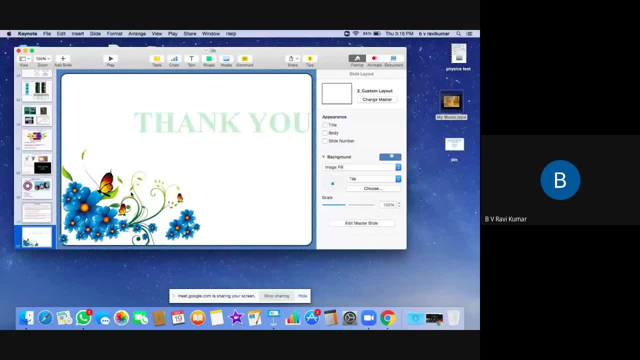 140 volts. so we have 28 volts, we have 56 volts, we have 70 volts and we have are four levels of voltages we are operating with, in fact, 56. you can agree- 28, 70 and 140.. this is for the dc to ac conversion for bl dc motor application. coming to the converter part, 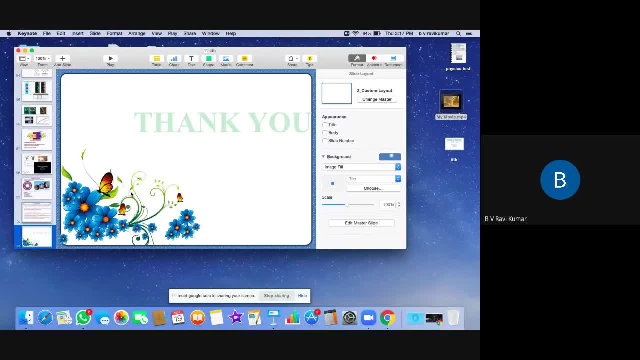 that is, a dc to dc converters for all avionics means all. all the missile consists of different subsystems. it will have an onboard computer, it will have an ins system, it will have some sensors, all those things. everything should be powered from a dc because we have to have a battery. so battery is unregulated so it will be connected to a regulated dc dc converter. so the dc dc converter normally operate from 18 to 36 volts input voltage and output voltage will be 28 volts constant. so we have an input range 18 to 36 and output will be 28 volts, so that 28 volts will be. 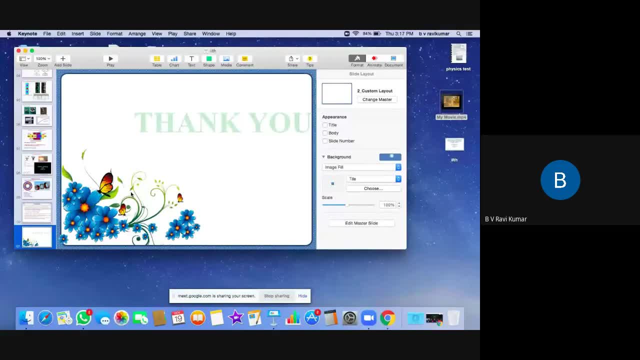 given to the each subsystems. like my actuator controller is there, it will take 28 volts from this dc dc converter. so all missiles. we use dc dc converters which are varying from 18 to 36 and 9 to 36 volts. so coming to this, one more just i want to give for information. 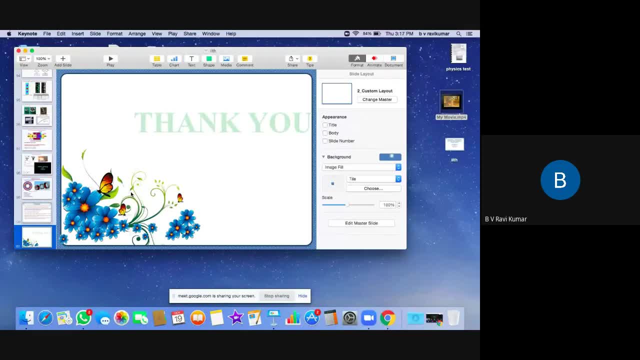 all these dc dc converters. most of the dc dc converters we are not getting in india because all the manufacturers are very from outside the whole, like western countries, but major dcdc converters. you people are presenting in lot of conferences all our indian students and indian professors. we are presenting a lot of papers in. 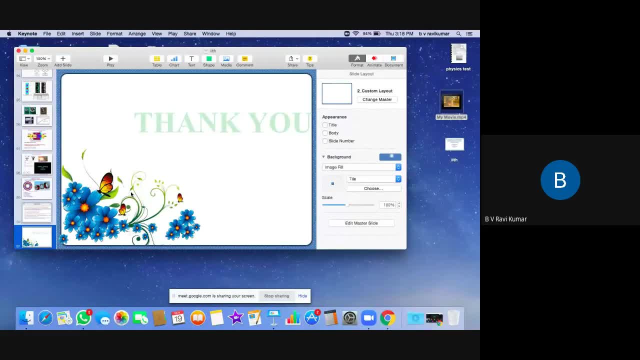 conferences. so this is also one of the area. we want to have compact dcdc converters with complete ema filter in build. so this is one of the developments we want to make so that we can utilize our own product instead of depending upon the outside world. so that is so. converters are being used left and right in all the 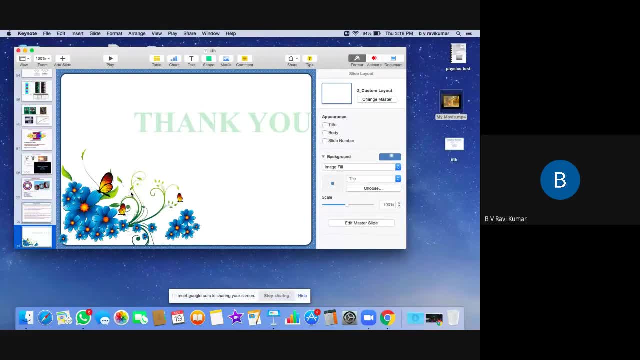 missiles. so you were asked for your question. everywhere we're using and these are the ranges. yeah, thank you, sir. sir, just one question. so, uh, sir, the current ranges, uh, does it go beyond 500 amperes or is it lesser than 500 amperes because actuators might be using a lot of current? to: yeah. yeah, but the current requirement, normally till now, whatever we have done, it has never gone beyond 500 amps. but because we are operating a little bit higher voltages, wherever we are going for the higher power, we are going for higher voltages. so maximum current. till now we have handled is 300 amps, so only on some applications we have gone up to 400 amps where we are going for igbts because that the voltage levels are some more so. so probably tomorrow we may have to go, but right now we are operating maximum at 300 amperes. 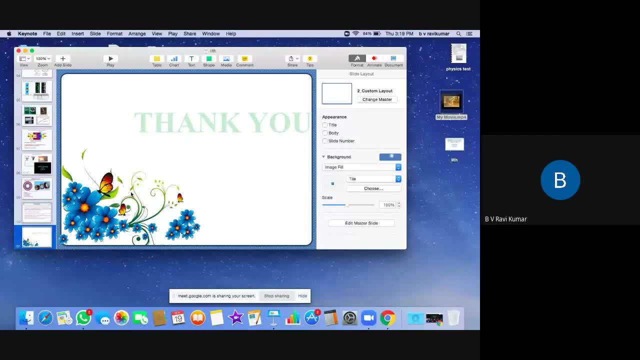 okay, thank you, sir, thank you, thank you, thank you, hello, uh, so is there any further questions or shall we end the session, sir, recently i heard that, uh, the rdo is going to set up laboratory at iith. what is it about? uh, yeah, yeah, something like that. 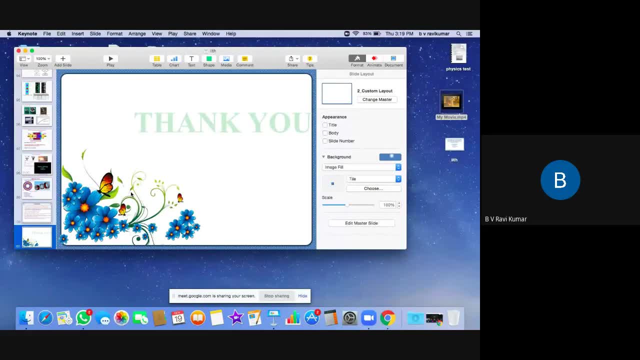 something is. i am sorry about that. i also. i heard that also, but uh, exactly, i don't know. probably i may not able to answer that, but one thing i can tell: iat and the hydra bear and our rci is setting up excellence at uh. we are based on our beloved chairman. 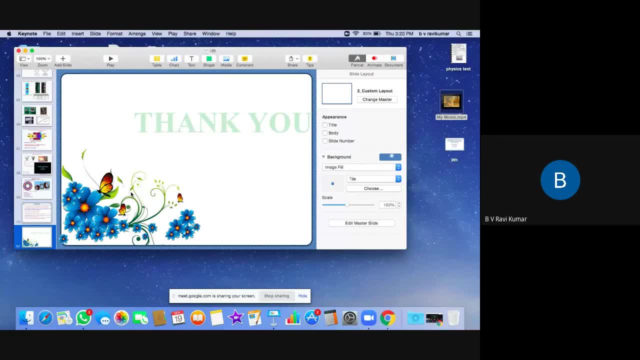 dr sufficiently. so i think we is one thing, i could tell you that we have an interaction with id for ph3s, so that i think we are starting women because we also- i am also involved in that- and we are just, uh, working out what are the topics to be worked out for? i think from electrical 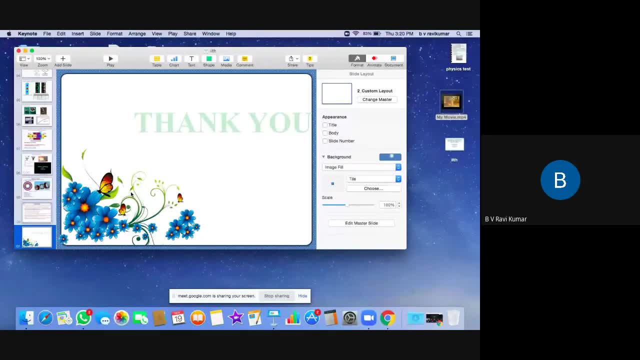 part we are just working out. but coming to the laboratory, to hydra bed also, it's true, but exactly what type of technology, all those things i don't aware at, frankly. so does dr do recreate from campus? uh, because, uh, excuse me, i'm sorry, i mean. 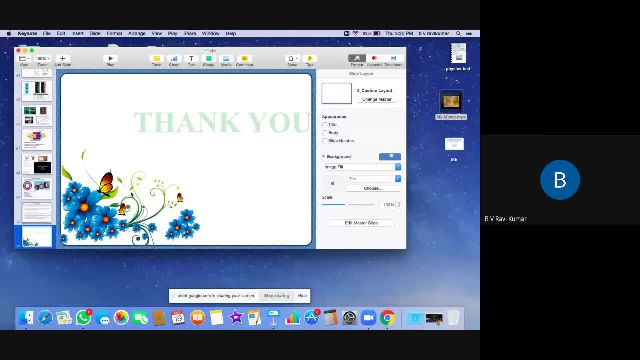 please ask technical questions. yeah, yeah, because there is more towards the hr i, i could not answer those things. yeah, yeah, so hello sir. yeah, yeah, tell me, sir, you are telling about control system design. yes, sir, still we are using pi controller. and what in the literature we? 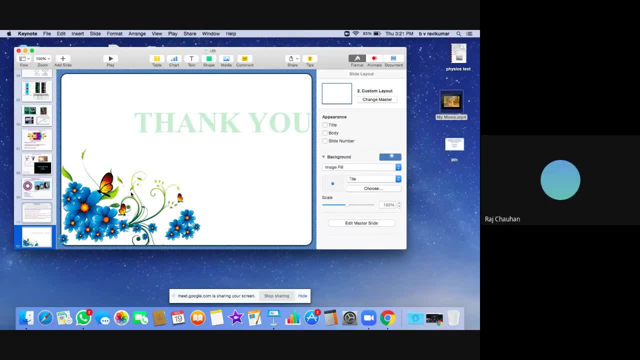 are reading till now. yeah, we are following that literature or some advanced techniques. i'll tell you, in the control systems it depends upon the application. basically, normally we use pa control. there is no doubt. whatever we are studying, same thing we are using in most of the applications because that is a sufficient for most of the provisions. but in some of the